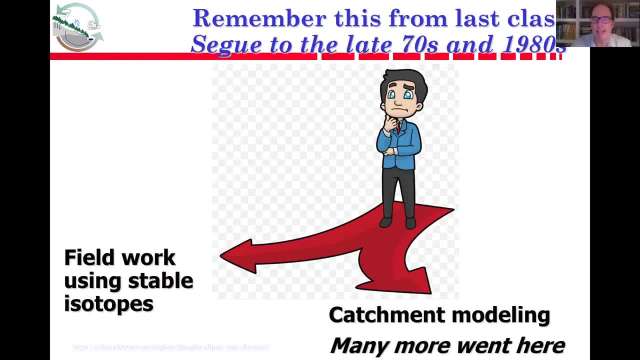 international hydrological decade And, as I mentioned last class, this is kind of a turning point around the mid-1970s because I would say most people working in the field transition to model were more focused approaches and only a smaller group of hillslope hydrologists continued. 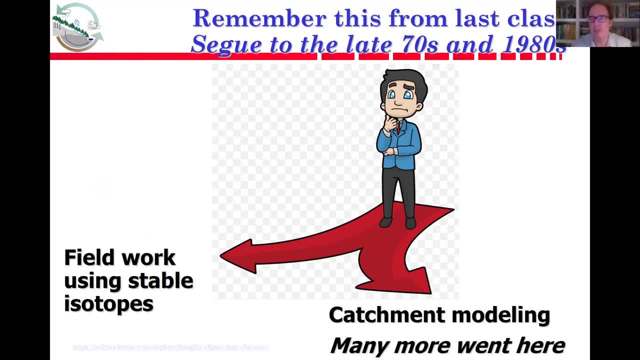 with field work, And much of that field work started to use these stable isotope approaches. Now there are many reasons for this. It was very attractive when computers became fast enough and easy enough to use to start to do computer modeling. There was a lot of pent-up. 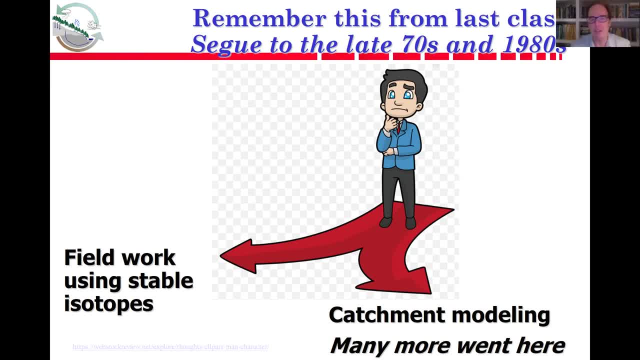 demand, as it were, But also the nature of funding meant that the number of people who would be interested in it- the number of people who would be interested in it- would not be as large as the number of people who were interested in it. 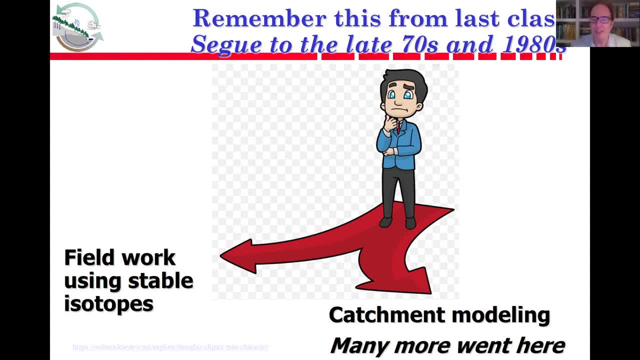 And so this is another interesting aspect of this. Now, field work is difficult and slow- production of papers and ideas. compared to modeling at the time and even today, much more can be accomplished in a kind of a modeling framework in terms of contributing to papers and kind of the immediate satisfaction that we have. 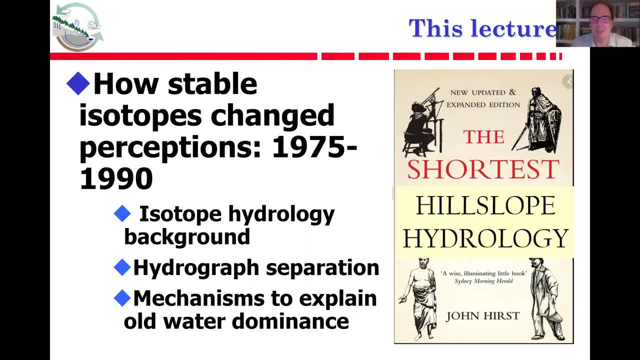 in science. So the shortcut or the roadmap for today's lecture is really how you can save money in the field, And that's a lot of work, But you also have to have a lot of money in the field. You have to have a lot of money in the field. So the idea really 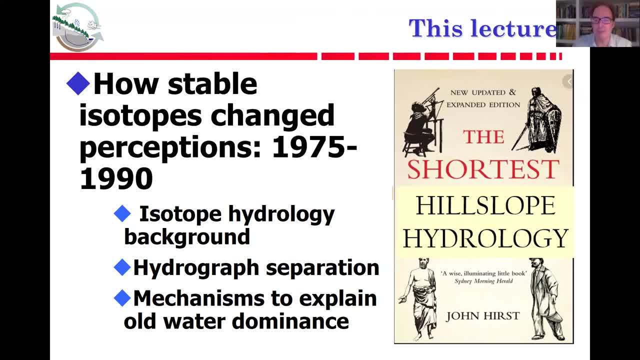 these stable isotopes changed our perceptions. We'll talk a bit about some of the background in isotope geochemistry, isotope hydrology. I'll talk about hydrograph separation and then some of the mechanisms to explain the early hydrograph separation results. And, just like 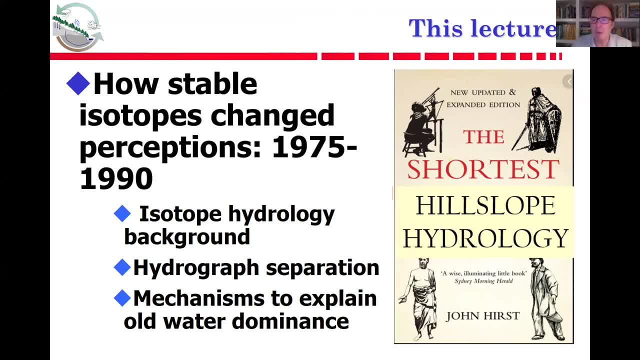 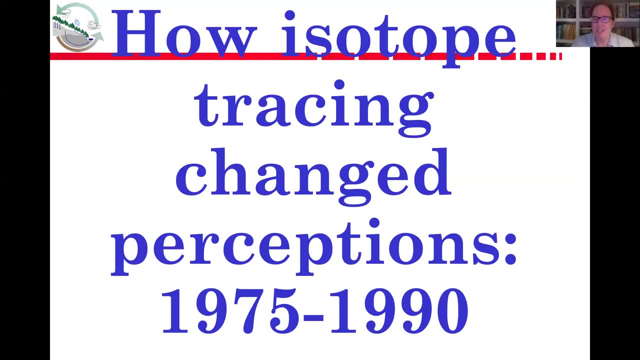 last class. if you have a question, just unmute and ask it, but we'll have a half an hour at the end for a longer discussion, So that's another possibility. Okay, so how did isotope tracing change our perceptions? Again, we're talking about this in the context of these periods that we've 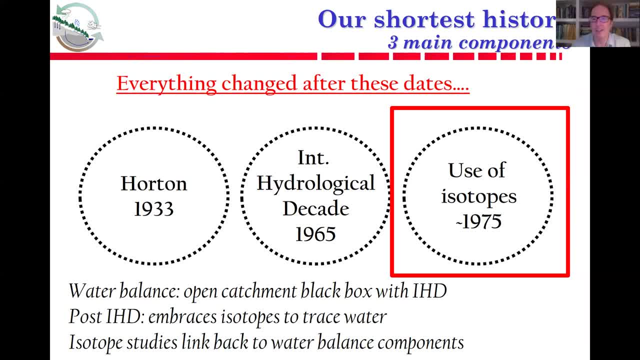 looked at from the beginnings of process hillslope work by Horton through to the great expansion of ideas during the international hydrological decade And how things changed, as we talked about last class, from a kind of an era of infiltration prior to the first international hydrological decade to an era of subsurface flow and its 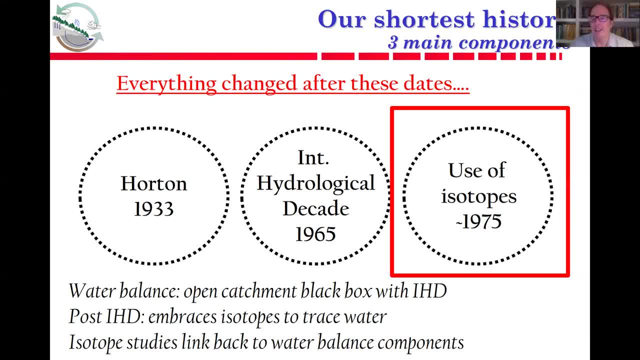 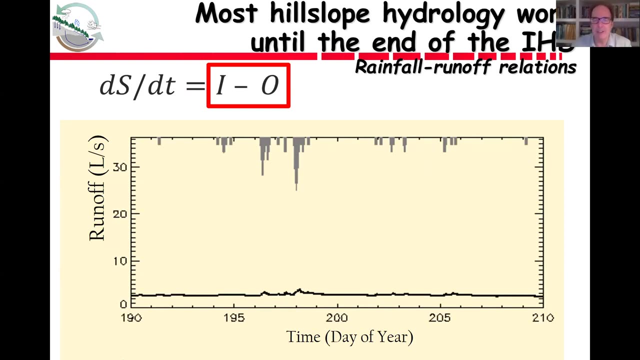 recognition And the isotopes you'll see today are really helping to understand the nature of that subsurface flow, based on the actual tracing of the water, following the water molecule, as it were, Through the hillslope. And just to go back to what we've talked about, most of the ideas and 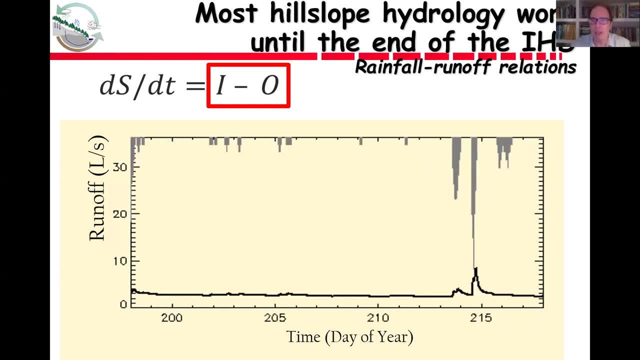 approaches to developing this perceptual model. this process, understanding of hillslope hydrology- was derived from so-called hydrometric measurements- rainfall runoff, for instance, And here you're seeing a rainfall runoff graph. This is for a small headwater catchment. 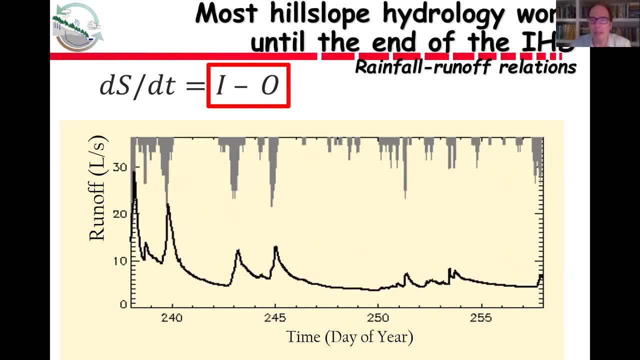 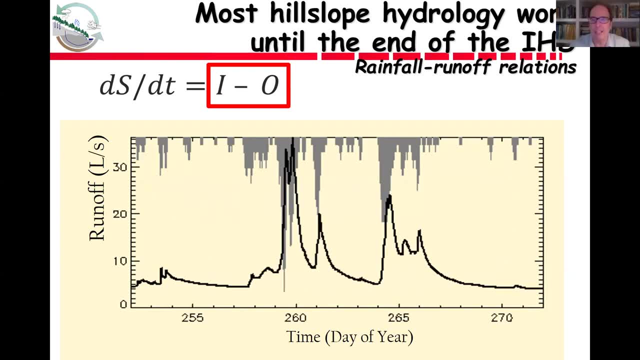 in Alaska And it's a very wet place, a surprisingly warm place, And you're seeing across the top the scrolling rainfall hiatograph And on the y-axis you see runoff and time of year or day of year, And much of the perception, then of these flow processes that we've talked about. 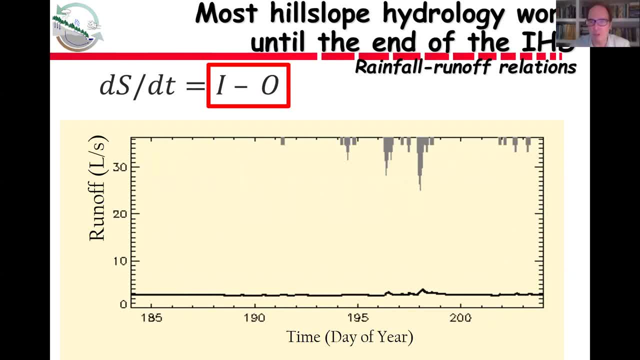 infiltration, excess overland flow, subsurface storm flow, saturation, excess overland flow- were all tied to the physical ups and downs of this hydrograph, And you've seen these hydrographs in your own work, I'm sure. But it's important to note that these hydrographs really are recording. 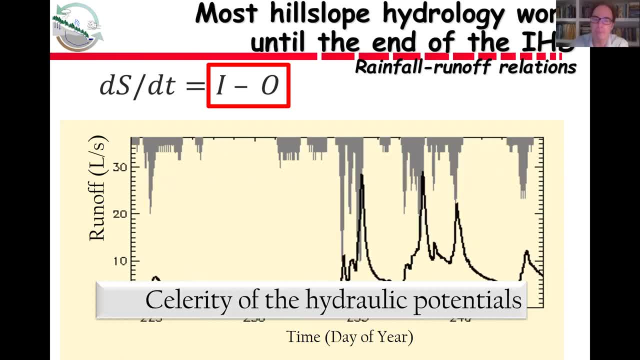 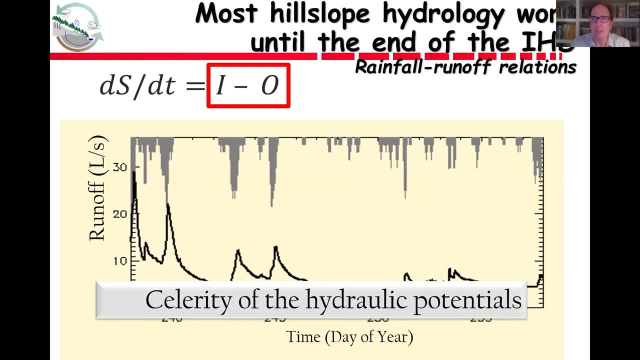 the pressure response through the landscape or maybe more precisely, the celerity of the hydraulic potentials. Remember we looked at the hillslope work of Darrell Wayman in East Twinbrook in England last class And there he had used tensiometers to measure. 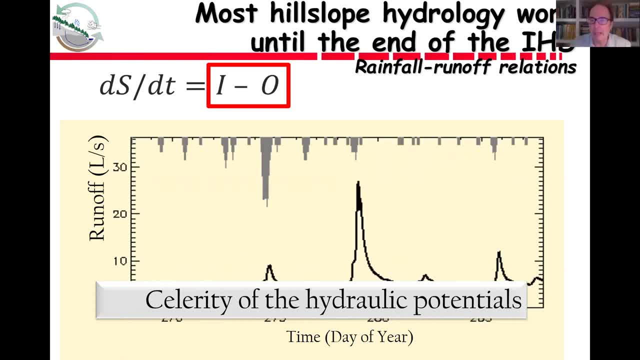 metric potential. Just remember, metric potential plus elevational potential is hydraulic potential And it's this celerity of the hydraulic potential moving through the hillslope that is forming this hydrograph response to rainfall or to an input. Now maybe you're wondering. 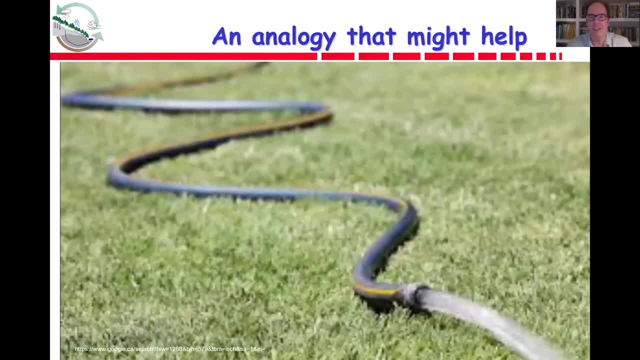 what is the celerity of the hydrograph response? So we've got a very simple analogy. just to kind of follow this through is kind of like a full garden hose of water that's sitting on the ground in the summertime And you pick up one end. 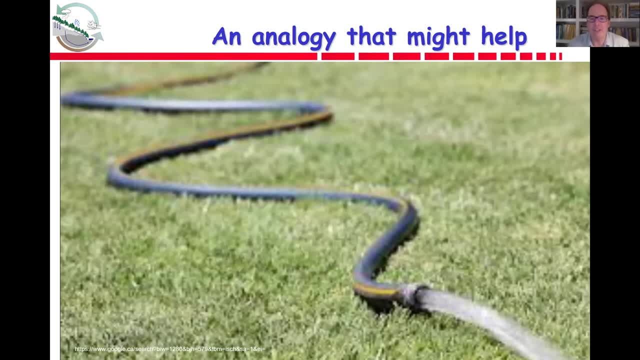 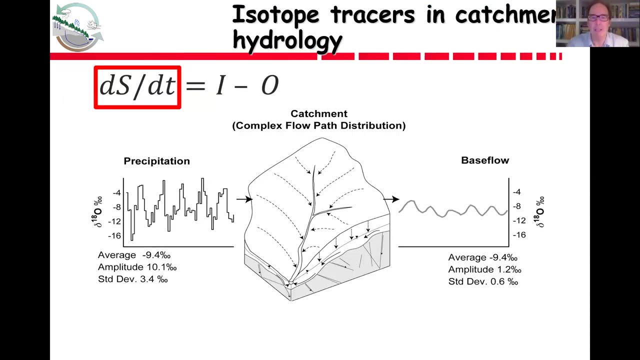 of the hose and what happens? Water immediately comes out And the immediacy of that flow is that celerity of the hydraulic potential moving through the hose, the pressure waves, the kinematics are a little bit like a water vapor. So it's a little bit more of a flow. but if we look at 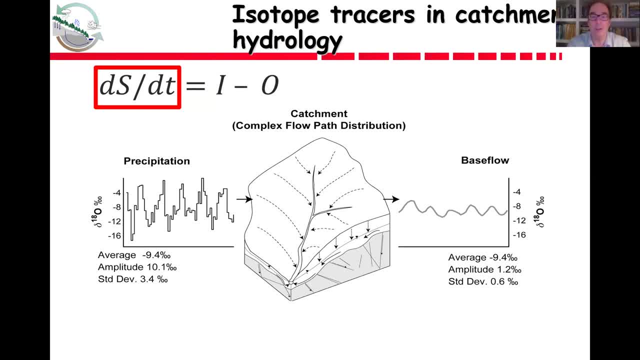 something that's carried with the water, in this case a tracer of the water or the tracer of the hydrogen and the oxygen that make up the water. then we can say something about the nature of the particle movement through the catchment or through the hillslope. 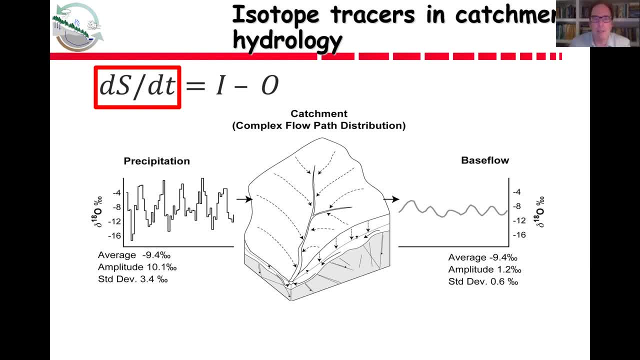 So on the left hand side you see the rainfall input, the precipitation input. this is a gauge that's collecting the rainfall and we're then analyzing for the isotope here of oxygen 018, and what you see is that the the rain is varying. 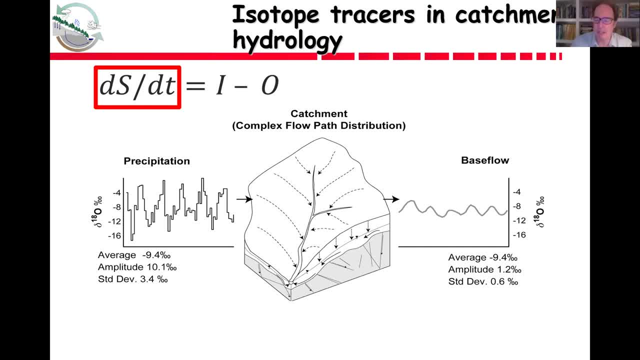 in a fairly cyclical way. and what's coming out? the base of the watershed. I don't know if you can see my my mouse here is a lagged and damped version of that input, so the isotopes are saying something rather different. the isotopes- 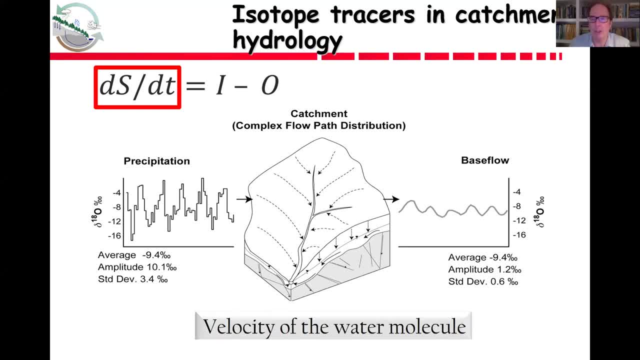 are tracking the velocity of the water molecule and this is very different to the storm hydrograph response. that's really tracking the celerity of the hydraulic potential and those two rates are very different. so we're going to talk a lot about these isotopes. so if those units or the nature 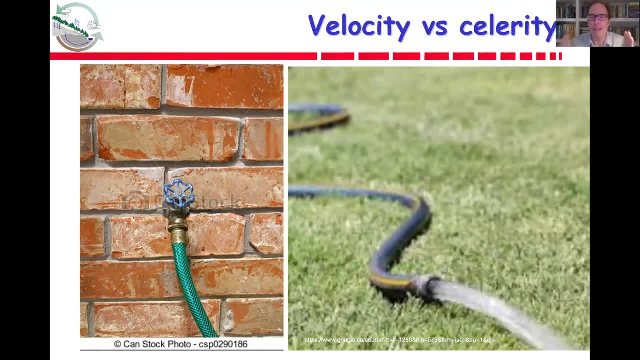 of those plots was confusing. we'll come back to that, but right now I just want to set the stage for the difference between velocity and celerity. so if we take that garden hose example I gave earlier and we take that hose and we hook it up to the water tap on the side of a house and we turn it on and this is. 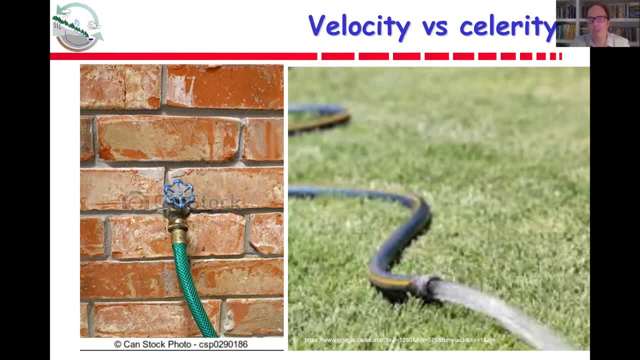 a hot summer day, the water coming out of the house is probably going to be cool and the water that's sitting in the hose on the ground is going to be warm. so you turn the tap on and again immediately water comes out the hose. but it might take several minutes before you feel, at the end of the hose, the cool. 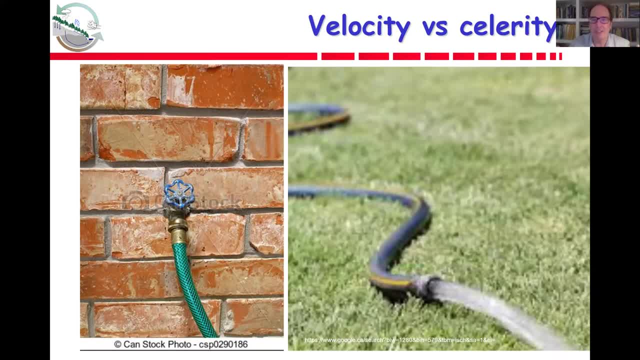 water. that's the analogy to the stable isotope. the velocity of the water molecule takes a long time to snake its way through the hose or through the hill slope, but the pressure response is immediate and those two things are quite different, and this is the added value that the stable isotopes bring to the study of hill slope. 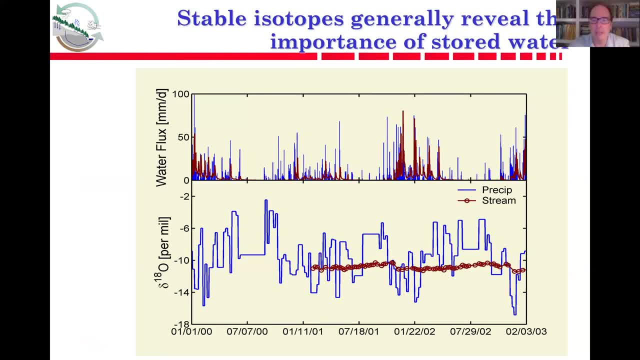 hydrology. let's look at some data before we get into definitions and more, more details. here's a catchment. this is in Oregon, in the northwest United States, and on the upper panel you see on the y-axis the water flux and on the x-axis is time. so this is about two years of rainfall. 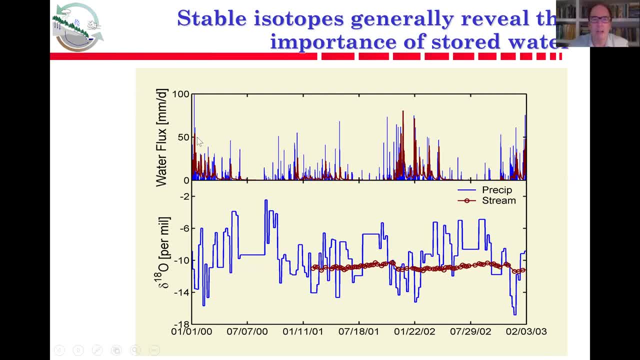 runoff data: the rainfall is in blue and the runoff is kind of in that dark red color and this is a catchment that has dry summers. so you see here, if you can see my mouse, dry summer, let's just see if I can make a bigger pointer. okay, maybe. 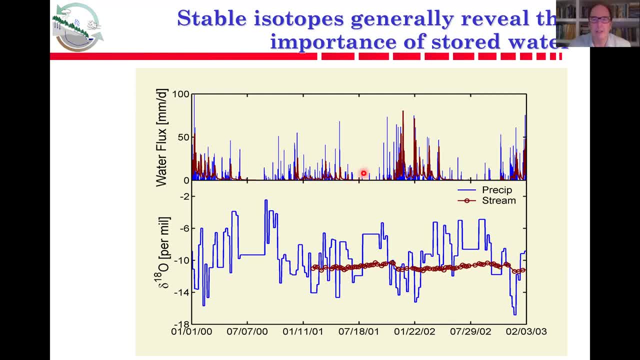 that's bigger. now is it bigger? there's a dry summer, there's a dry summer and there's a dry summer, and then these are the rainy periods, and what you see is that when the rain starts falling, you get immediate response in the stream. the hydrograph responds very quickly to the storm rainfall once the the hill slopes. 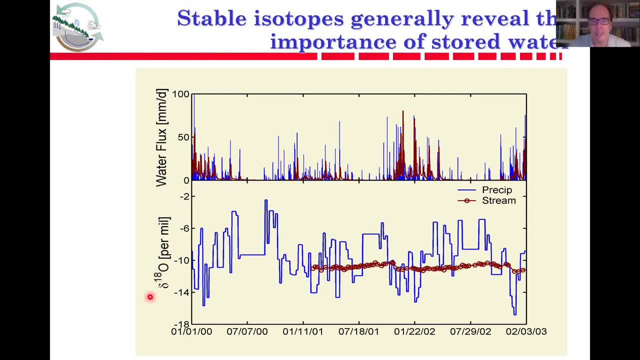 went up, but now look at something that's carried with the rain. remember, water is h2o and this is one of the stable isotopes of the oxygen molecule. that's part of the water molecule. and now look at the blue here this is the rainfall. again, it's a varying quite a bit. 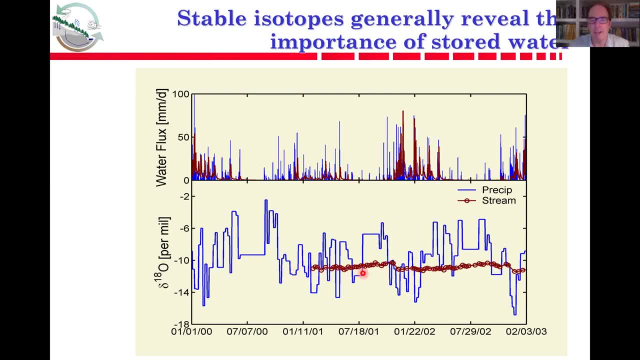 but now, rather than the stream responding very immediately to the rainfall input, isotopically it's very, very lagged and damped, and there's a really lovely paper that was published in 2003 by Jim Kircher, who is at the ETH in Zurich, and he called this the old water paradox. this is the idea that hill. 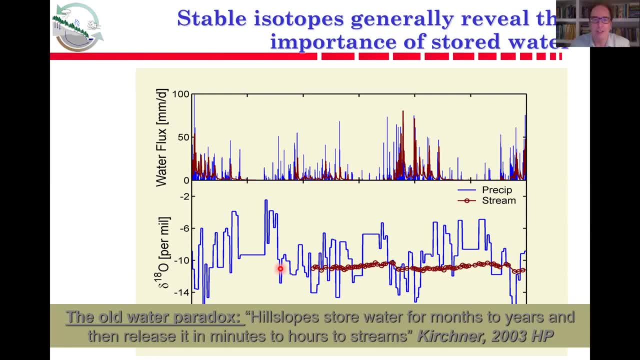 slopes are storing water for months or years but releasing it in minutes or hours by driven air to the stream, and this process, or this paradox, if you like, is something that's really been a focus in hill slope hydrology since the start of these stable isotope tracer uses in the mid 1970s. 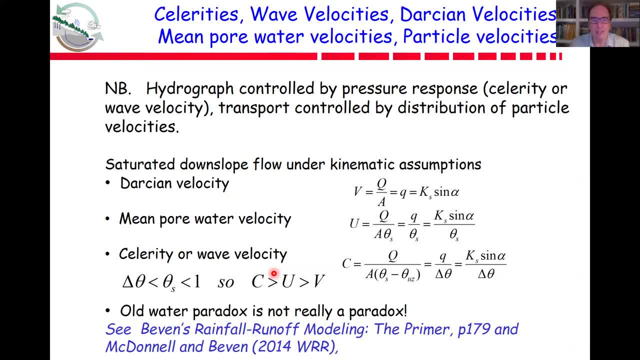 now, of course, if you read a textbook- this is from keith bevan's rainfall runoff modeling textbook- these are different velocities: wave velocities, darcy velocities mean poor water velocities, particle velocities, and when you read your hydrological textbooks you'll remember that, wow, these, these velocities are in fact rather different. for instance, the celerity or wave. 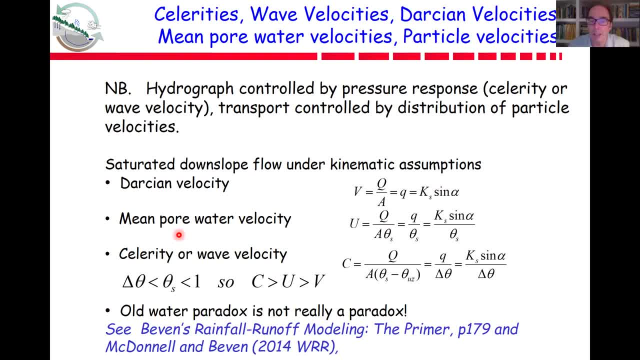 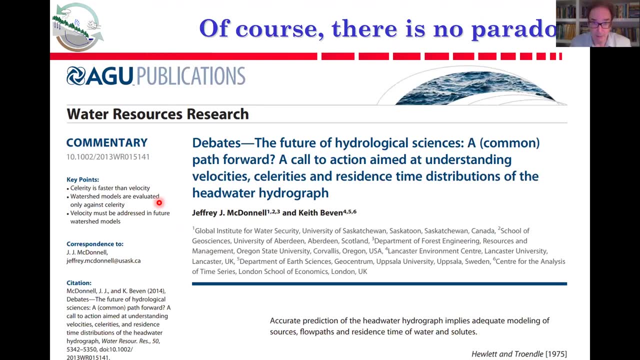 velocity in comparison to, say, poor velocity or darcy velocity. we're not going to go into the details of these equations today, but just to know, there's been a lot written on this. in fact, keith and i had a paper uh five or six years ago now in water resources. 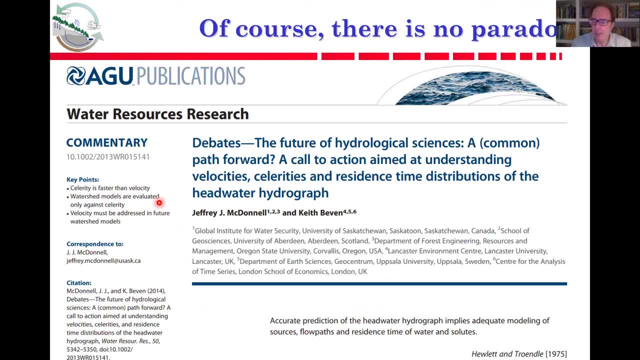 research on this, this very topic, and we thought it was urgent enough to have what we said was a call to action aimed at understanding really, the differences between velocities, celerities and residence times, because i think it's really important to understand the difference between velocities and residence times, because i think there's still a fair amount of confusion in the 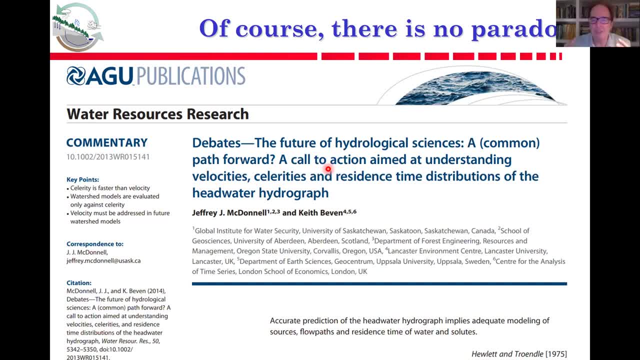 literature on this topic. but again, it's not so confusing if you go back to the hose analogy and that's a way to maybe simply understand how celos celerity is much faster than velocity and most of our work prior to the use of stable isotopes. 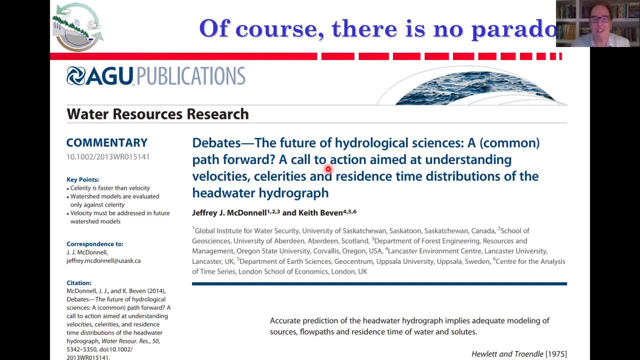 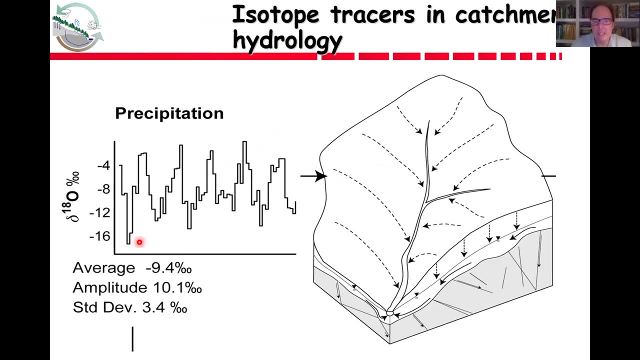 everything was evaluated against celerity, not velocity, and i think this is really a good way to understand. why are there these differences in the originality of the models, but really the future bringing velocity into our, our models. so what we're going to do now is try to understand a little bit. 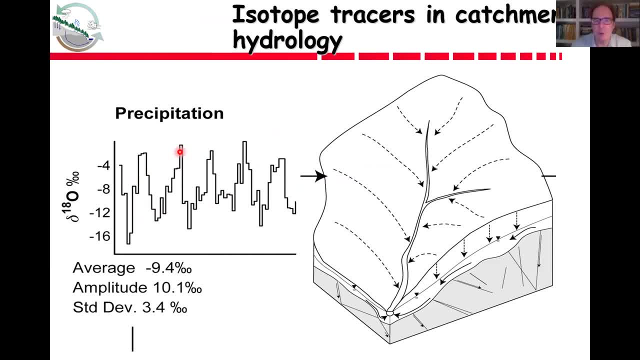 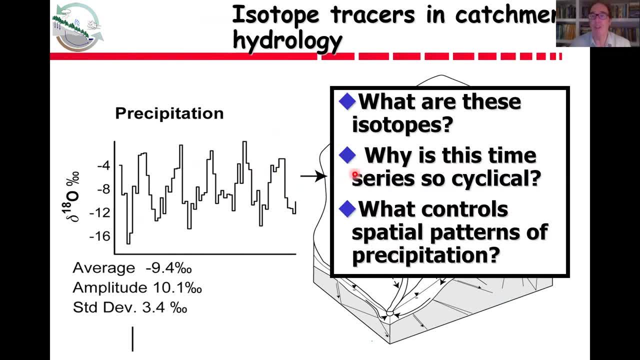 this nature of rainfall or snowmelt, isotopes, what is it that makes this go up and down in a kind of a sinusoidal way? and we're going to go after questions about: well, first, what are isotopes, and then, why is this so cyclical and what might control the spatial activity in the water? has to beああ. 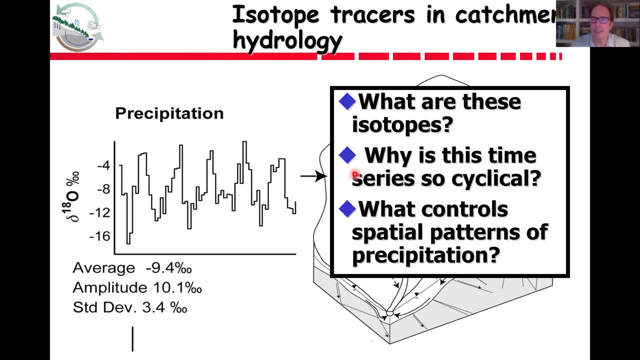 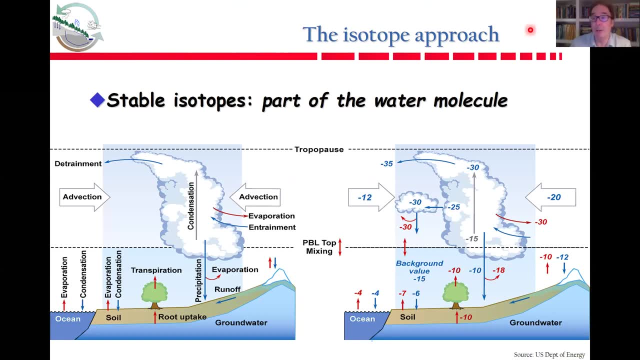 spatial and temporal patterns, So I want to just spend a little bit of time on that, in case you've not been exposed to stable isotopes previously, Well, what is a stable isotope? It's part of the water molecule. Remember we said that what we're talking about are the isotopes of 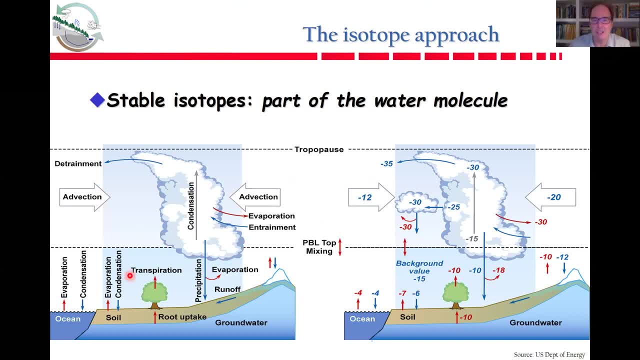 hydrogen and oxygen. Here on the left-hand side, you see a very familiar water balance or a terrestrial water cycle, And on the right-hand side you see the isotope composition. This is for oxygen-18 in a unit called per mil, parts per thousand, which I'll define in a minute. 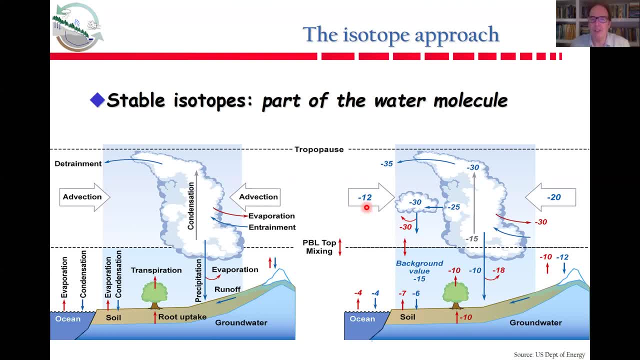 And for the vapor and for the water. we can now measure this with ease. When I was a student, like you, it was not easy. It was very difficult to make these measurements in a chemistry lab on a mass spectrometer. And for the last, oh, 15 years or so, we've had these wonderful things called laser spectrometers. 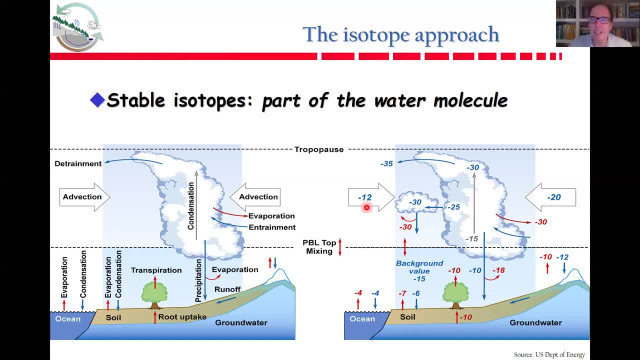 And now all of us can make these measurements quite easily, cheaply and simply and accurately in our labs, in hydrology labs and ecology labs and so on. But just to make it clear that we can measure not just the liquid but even the vapor now, of each of the pieces of this water cycle. 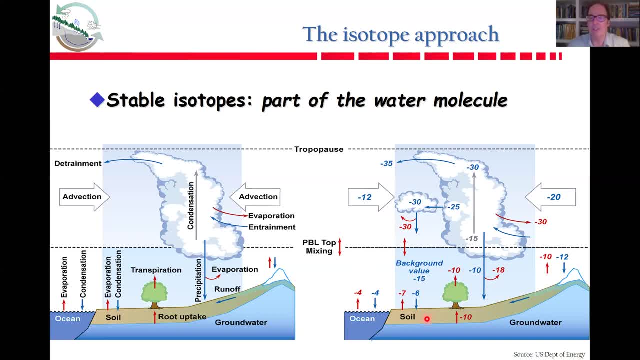 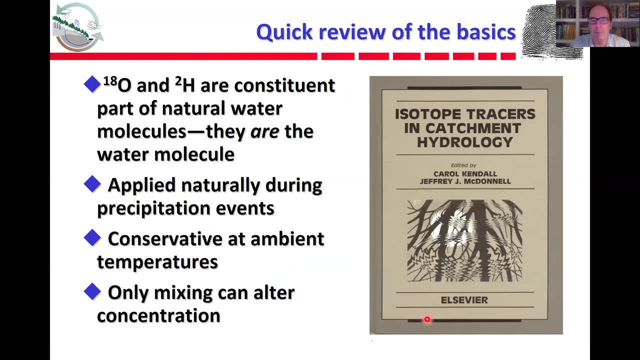 that's moving And we can use this to really track raindrops through our landscapes. So it's really come a long way since the beginning uses in 1975.. So a quick review of the basics. And this is a book that came out now in the late 1990s, a long time ago. There are many good recent books that have come out as. 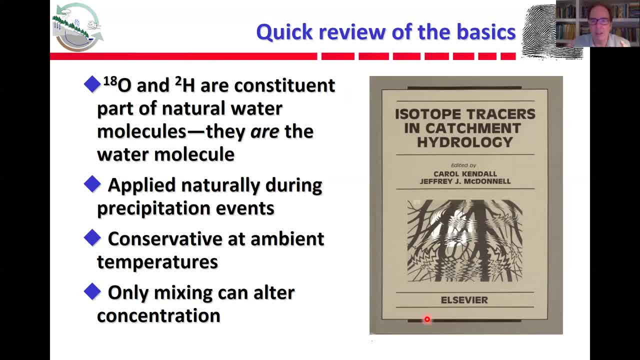 well, What I want you to think about is these are like fingerprints to track the water. They're part of the water molecule. They're applied naturally during precipitation events, So you don't need to add anything artificial. It's happening everywhere when it rains, They are. 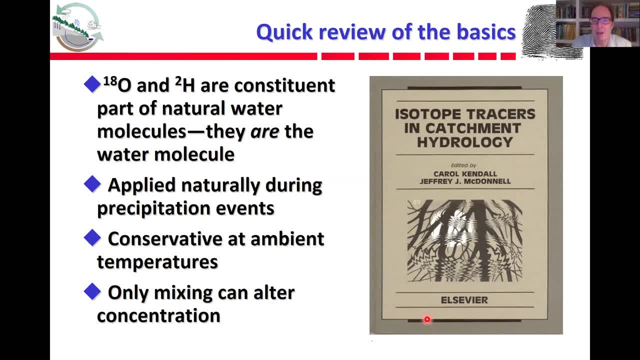 conservative at ambient temperature And only mixing can alter the concentration. So, unlike chloride or silica or electrical conductivity tracers you might be familiar with, these don't react along the flow path. They are beautifully, perfectly conservative, And we'll talk about some of the things that do change the 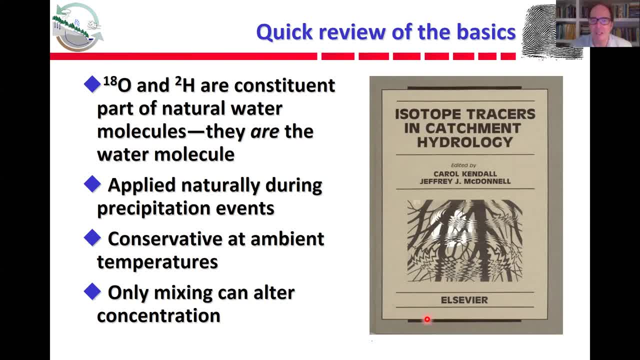 signatures. But this is why it's been such a revolution, Not just in hydrology, but paleoclimate reconstruction, climate modeling. There's now isotope enabled: global climate and regional climate models. If you're doing that kind of work, you might know of NOAA MP. That's an isotope enabled. 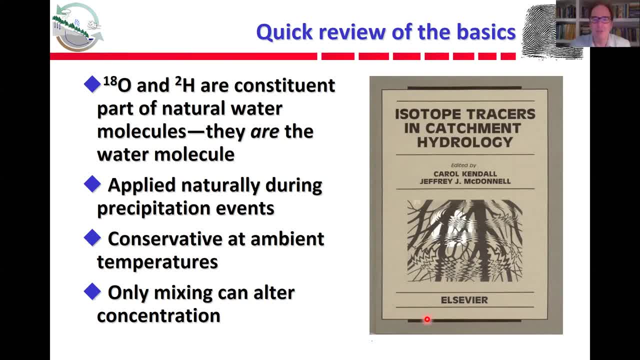 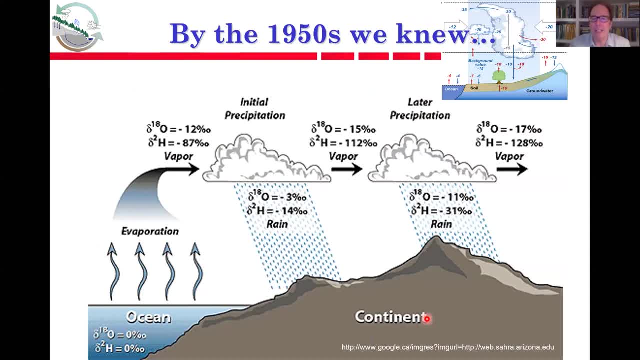 regional climate model, climate model now it's really found its way into so many fields. So already by the 1950s we understood how water that starts off in an ocean- and you'll notice the units here are zero per mil, parts per thousand. This is the origin of the cycling of water that we're going to track. 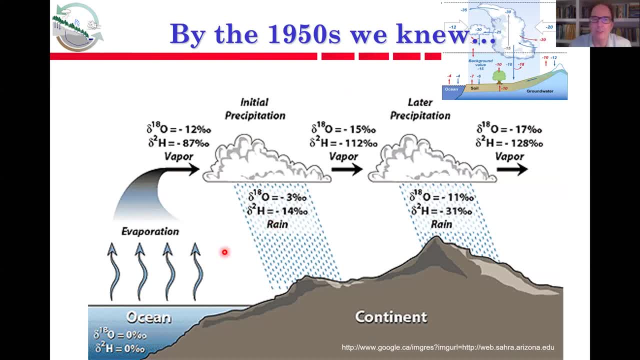 through our hill slope or catchment water cycle. So even by the 50s we understood how evaporation changes: the signal of the vapor that's coming out of this evaporation and then condensing in the form of clouds, and then the sequence that you might find as you move on land. 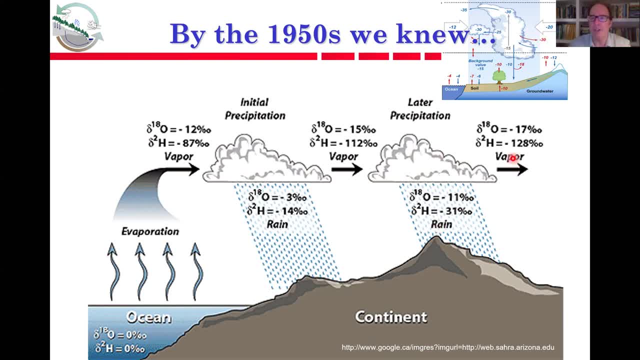 with an air mass and how it then rains out different signatures to our hill slopes or to our catchments, And these processes are well understood and have been now for many decades. We're going to look in a bit more detail at this as we go along, But I just want to give 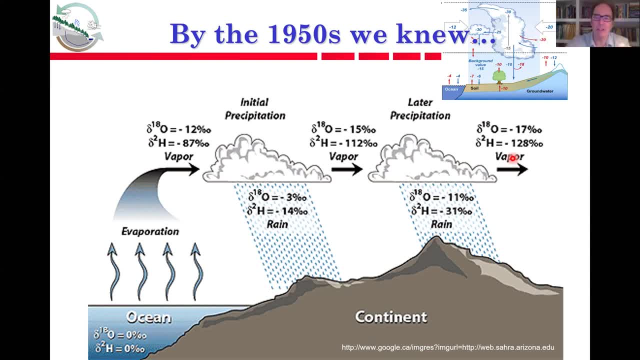 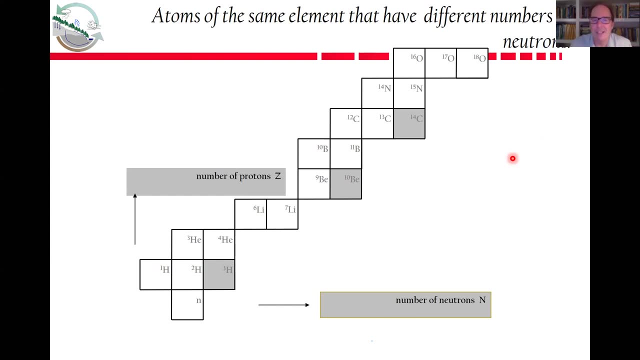 you some bigger picture of what controls those variations we were looking at earlier and we'll talk about how this works in a moment. So the first thing you need to remember, kind of going back to high school chemistry, is that these isotopes are atoms of the same element that have a different number of neutrons. 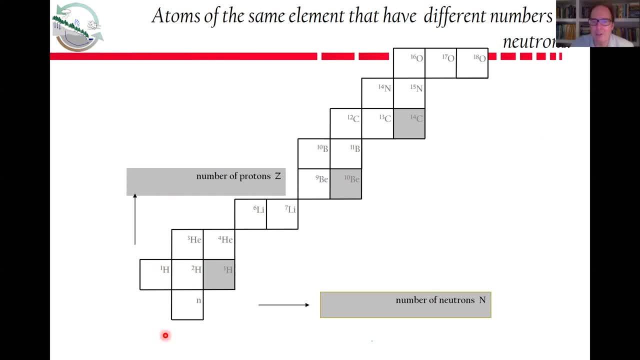 So, if you remember on the periodic table, protons go this way, neutrons go this way. So look for hydrogen. We have 1H and 2H. The 2H has a name, It's called deuterium, And then 3H, which is a. 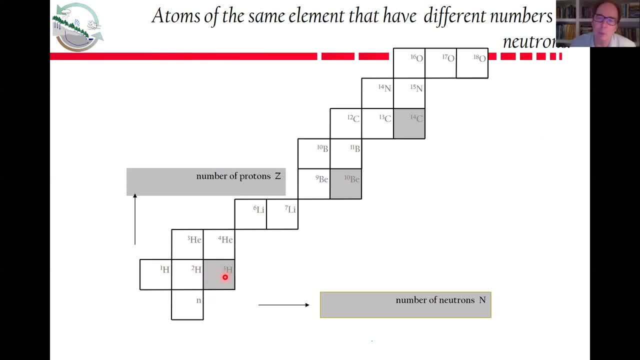 radioactive isotope. we won't talk about today but we will on the fourth lecture. This is called tritium, that you've heard about, probably, And then up here, oxygen, the other piece of the water molecule. going from left to right, we're. 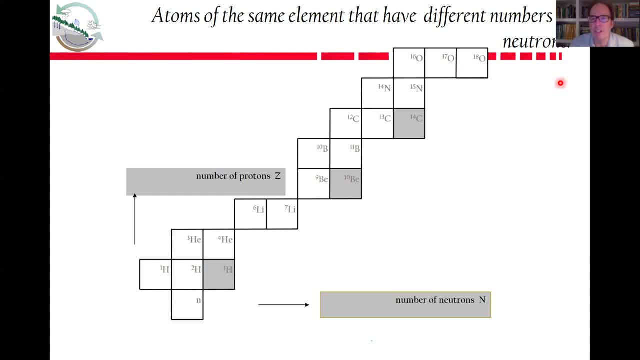 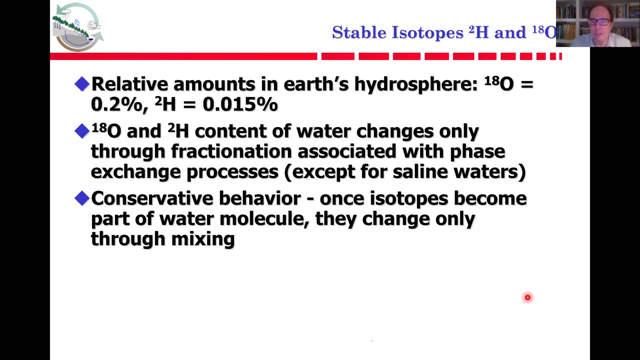 increasing the number of neutrons, going from 016 to 018.. These are the isotopes we're going to talk about, But just remember, they're atoms of the same element that have different number of neutrons And their abundance is quite different, whether it's the so-called heavy or light isotope of these. 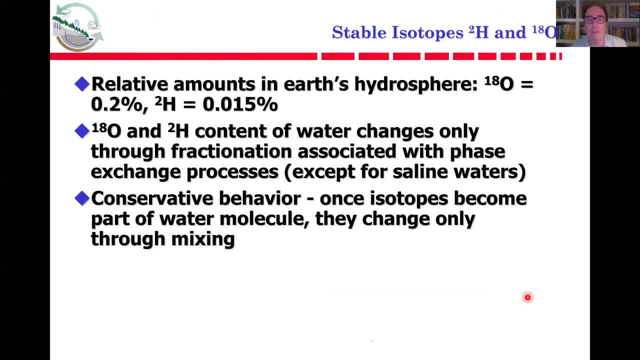 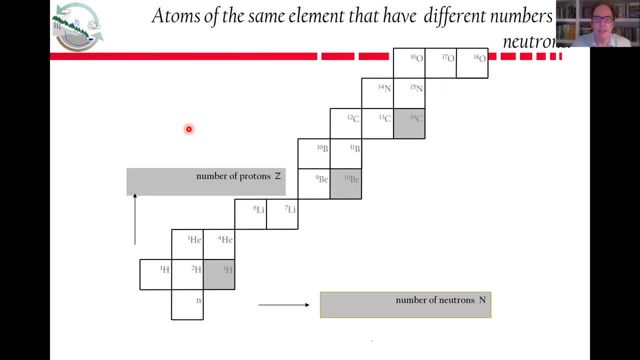 molecules of oxygen or hydrogen. So, for instance, we're going to focus a lot on 018 and deuterium. Let's just go back one slide. These are the so-called heavy isotopes. Why do we call them heavy? Because they have more neutrons. Think of them as physically heavier. So when we talk about deuterium, 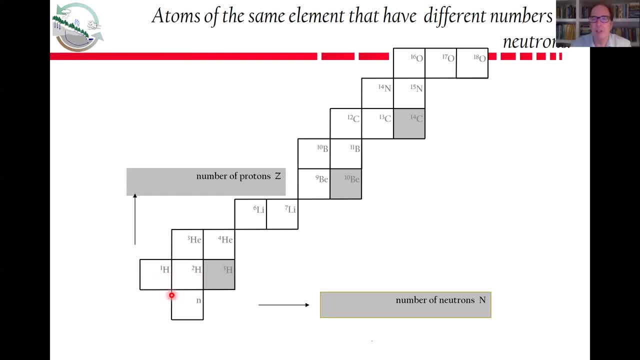 here: 2H, it's heavier than 1H. When we talk about 018,, it's heavier than 016, if you've been around for a while, you can see my cursor showing this here. So that's what we're going to focus on. 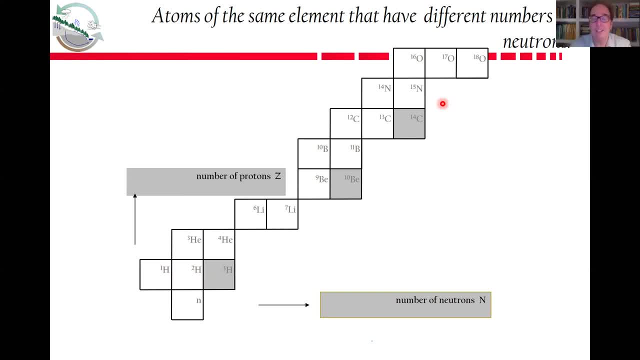 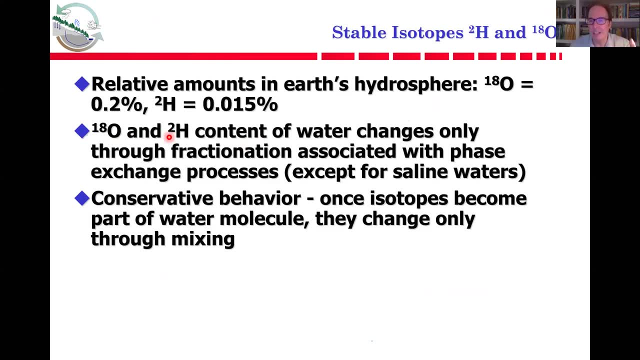 these ratios of light and heavy of these individual molecules and their isotope values And these contents of these heavy isotopes. they change only through something called fractionation. It's kind of a separation that I'll define in a little bit, And they're conservative, as I mentioned before. 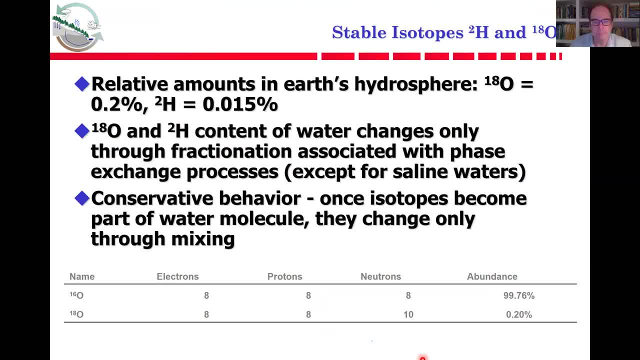 and if we think of the relative abundance, for instance for oxygen, most of the oxygen is made up of 016, 99.76%. Only a little bit is made up of the 018.. And the 018 is what we're going to be focused on. 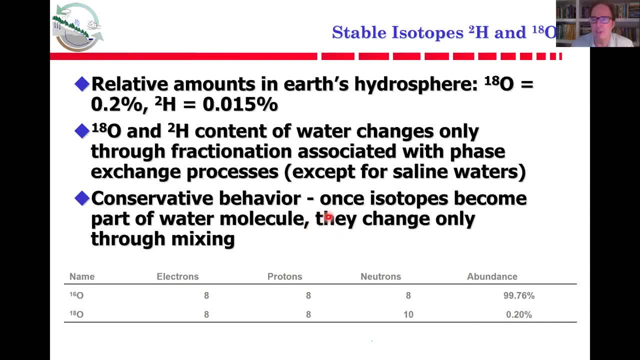 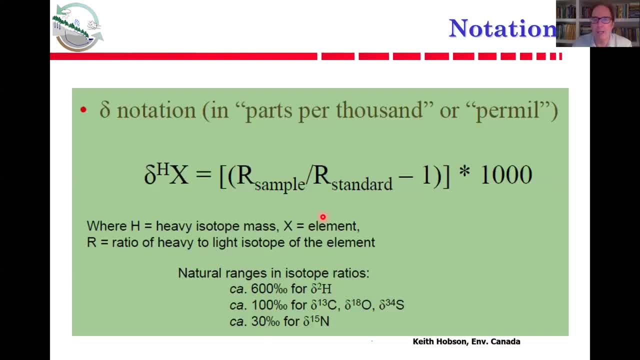 and we're going to be using these as conservative tracers. 018 and deuterium. Now the units are funny to me, I know, but this is because we're always comparing it to a standard, So we get the unit of. 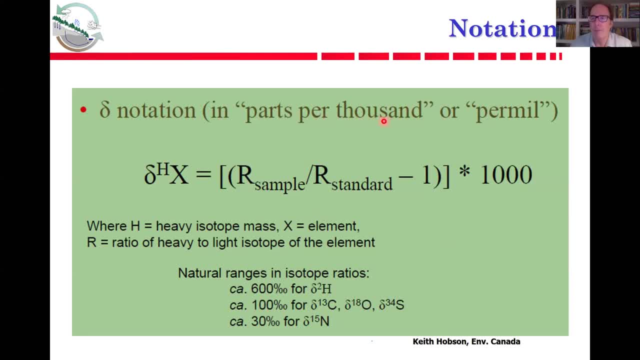 per mil or parts per thousand, the symbol that looks like a percent, with an extra zero or O down in the bottom right-hand corner, because we take our isotope sample and we look at it relative to a laboratory standard And then we multiply it. 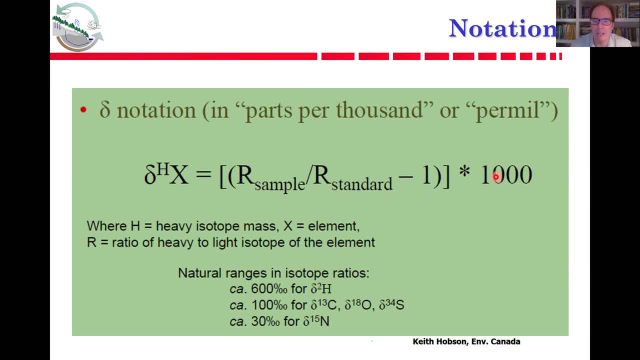 And then we multiply by a thousand to get the number up to a kind of a whole number that we can work with. And these are some of the different ranges for some of these heavy isotopes, if you like: 018, zero to maybe up to 100 per mil and deuterium up to 600 per mil. in terms of the range in natural. 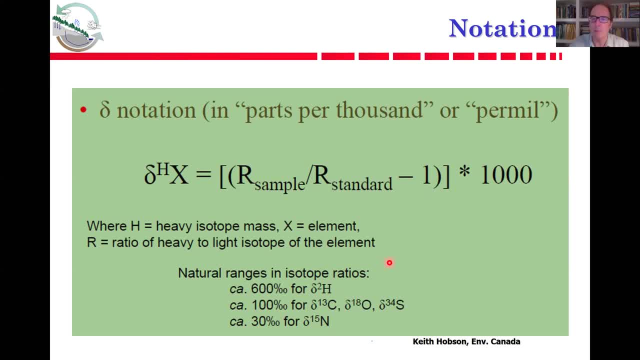 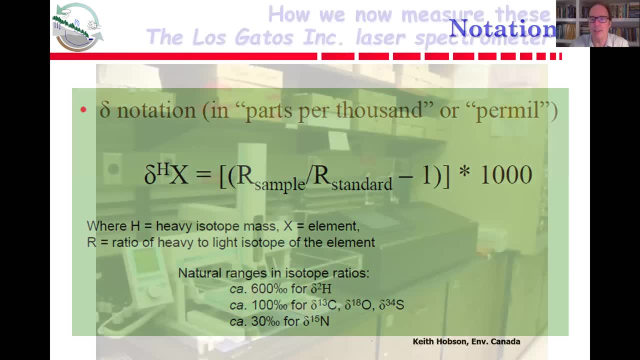 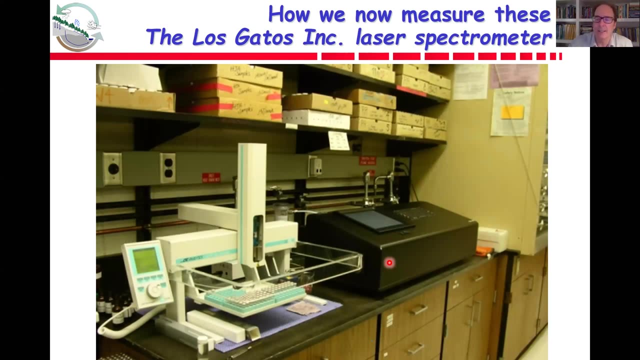 systems. So again, we're going to use this parts per thousand or per mil notation To look at these, these values and everything's made relative to a standard, And these standards are distributed by the UN's International Atomic Energy Agency And then local lab standards are made. 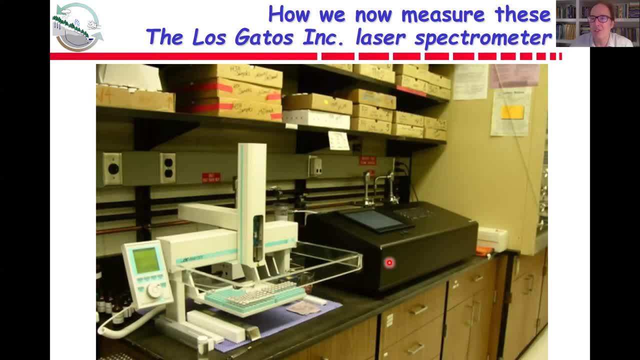 of course, from those precious standards, And the standard is mean ocean water. And here is a laser spectrometer. Basically it's a device. it's got a mirror at either end And it's a laser spectrometer. it's got a mirror at either end, here and here, And it shines a laser between the ends of this black box. 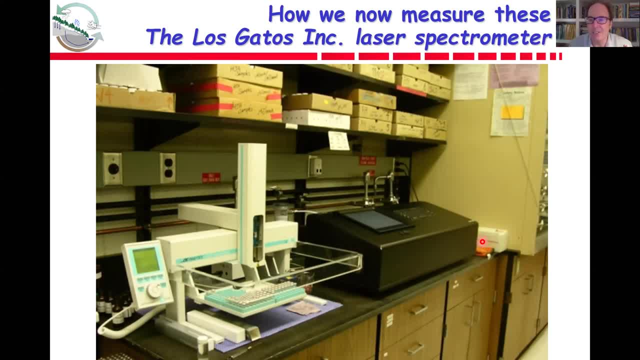 You get about 30 kilometers of laser light set up inside that box And it's able to make very fine measurements of the spectra of these stable isotope signatures And these are fed in through this device, which is simply an auto sampler that's taking some liquid from one of these vials that we're going to use to measure the 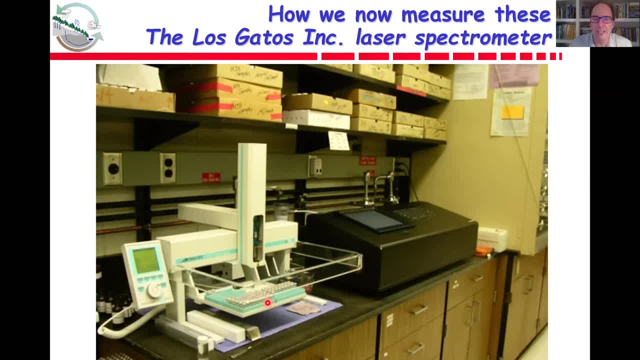 temperature of one of these vials that we've collected, let's say, in the field, and that transfers it into this, this laser spectrometer. These now in US dollars are worth about 60 or $70,000. And that may seem expensive. 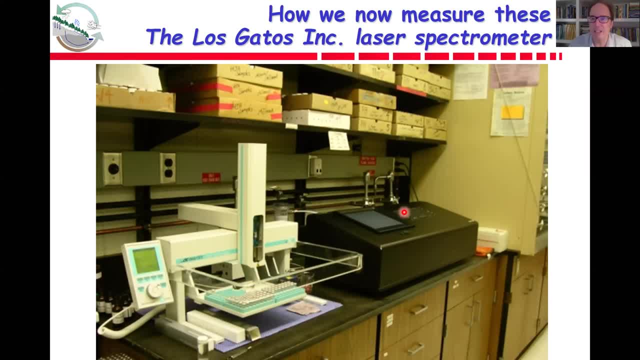 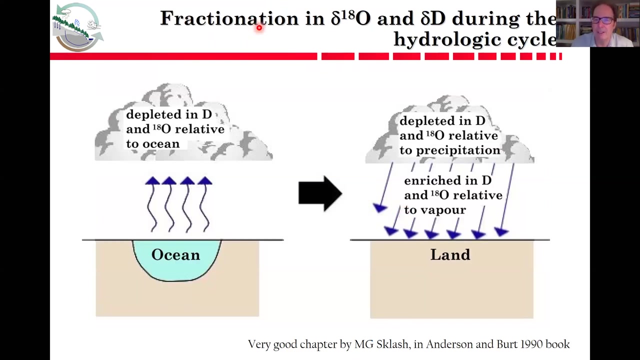 but it's probably 10 times less than a mass spectrometer and 100 times easier to use. So this is really revolutionized the field, And these became available about 2005 or 2010.. Okay, let's go back to this little diagram and think about this thing called fractionation, the separation. 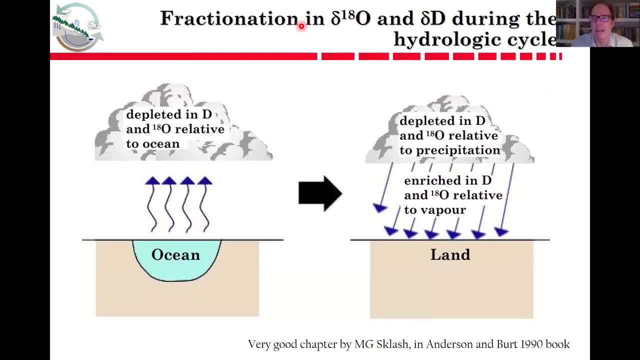 And what we're talking about is the how our isotopes are affected by evaporation and condensation, the so called changes of state that are the things that result in that separation of the light and heavy isotopes. So let's go to our ocean. we have evaporation. 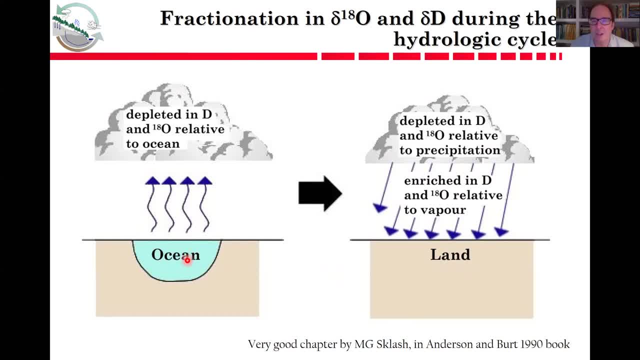 What happens. The lighter isotope is evaporated preferentially and the heavier isotope stays behind. Remember the difference in weight, different number of neutrons, let's say for 018,, 016, or deuterium and hydrogen. So that means that when we have evaporation the cloud water becomes depleted in the heavy isotope of deuterium or 018, relative to the ocean water. 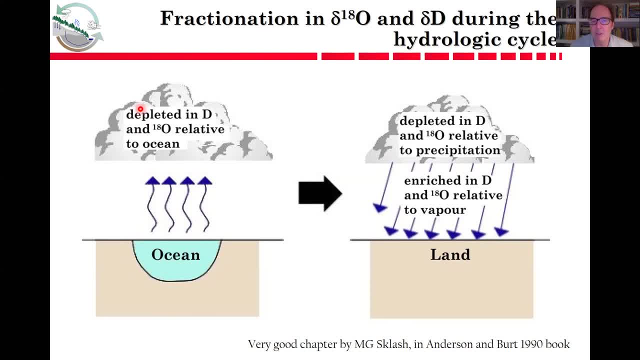 So that means that when we have evaporation, the cloud water becomes depleted in the heavy isotope of deuterium, or 018, relative to the ocean water. Then, when this moves on land and rains out, what happens? The opposite: The heavy isotope falls out first and the light isotope is retained preferentially in the vapor in the cloud water. 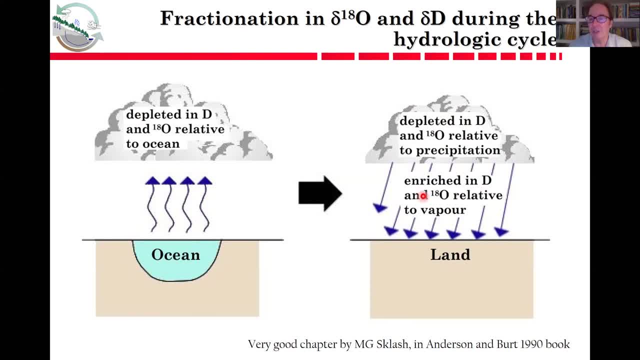 So what this means is that the rain is enriched in the heavy isotope, deuterium and 018, relative to the vapor. So this is like distillation. This is like evaporation and condensation. This is like distillation. This is like evaporation and condensation. 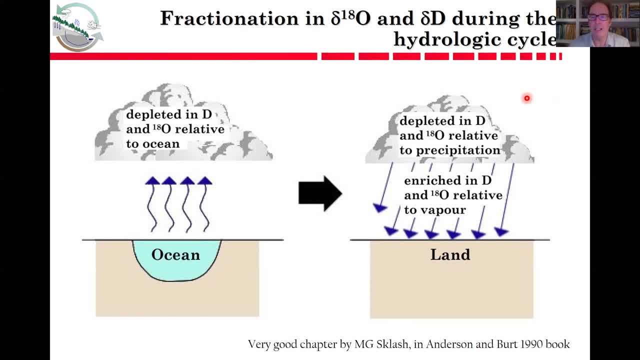 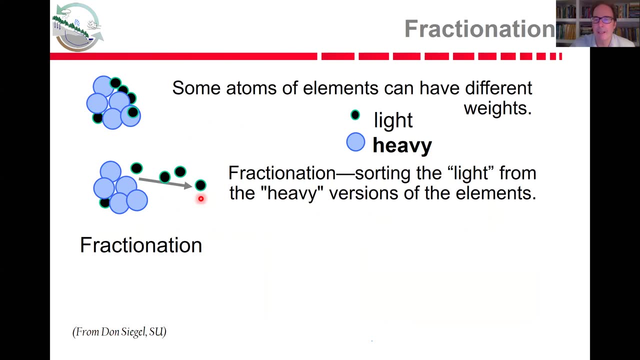 Changing these ratios of light and heavy just because the heavy is easier to fall out, to rain out of the cloud mass and the light is easier to evaporate into the cloud mass. So think of it literally as light and heavy. So this is fractionation. 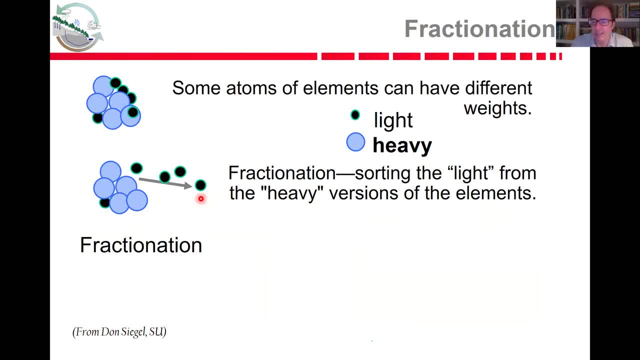 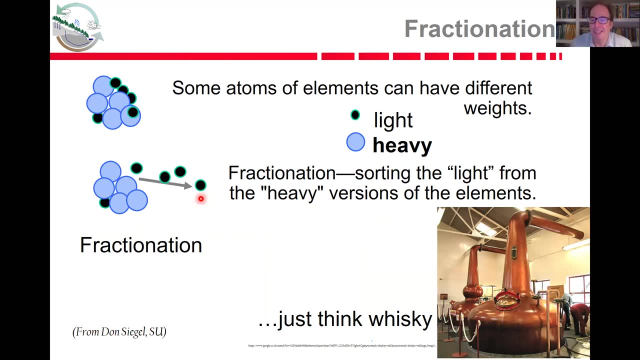 It's just sorting the light from the heavy, And I'm a big fan- I think Pan might be as well- of Scottish whiskey, And this is the same process as this kind of alcohol production- distillation, if you like- where you have the light vapors rising in the still. 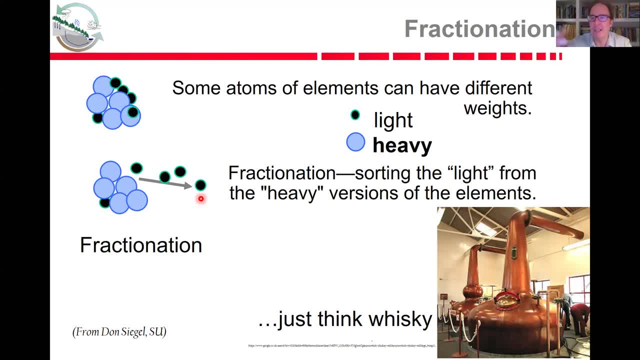 And then they're cooled and they condense And this is a way to separate water or alcohol from the kind of the watery substance in the still. It's the same kind of process And if you've done chemistry courses, you've probably done- you know- work that looks at distillation. 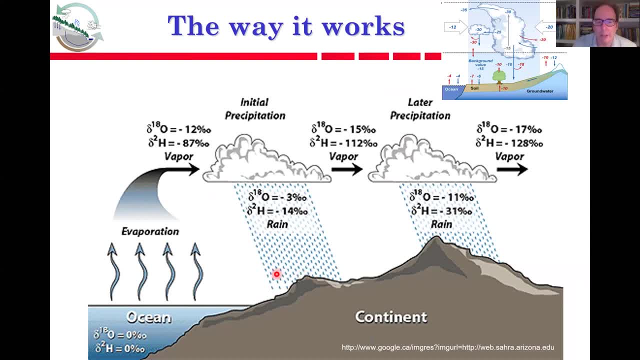 So, going back to this diagram, then now what we know is we have a standard mean ocean water, zero per mil. We have evaporation. What happens? It gets lighter because we're preferentially evaporating the lighter isotope, The heavier isotope stays behind. 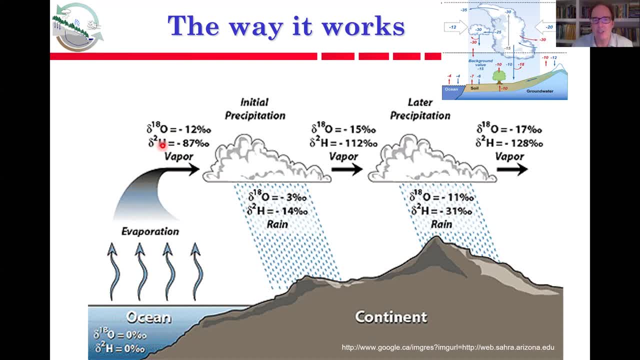 So now the signature of the hydrogen and oxygen are more negative. They're lighter than the water from which it came. Now this forms the cloud water. And what happens? The rain that falls out of the cloud water. look at how it compares to the vapor from which it came. 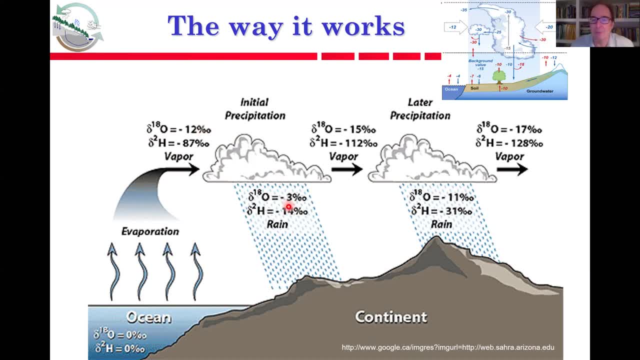 It's now heavier, closer to zero. So O18 is minus three per mil, Deuterium is minus 14 per mil. Now that cloud continues to move. Well, continues to move on land. What happens? It's getting lighter and lighter and lighter as it moves on onto land because we're raining out the heavier isotopes. 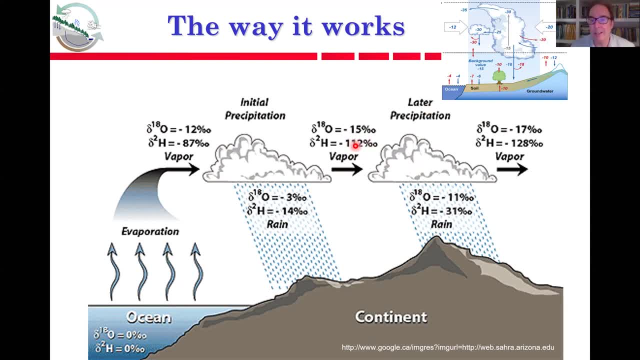 And not only is the cloud water getting lighter, even the rain is getting lighter. It's still heavy relative to the vapor, But it's you can see that this rainfall here at higher elevation, farther inland, is lighter than it was closer to the coast. 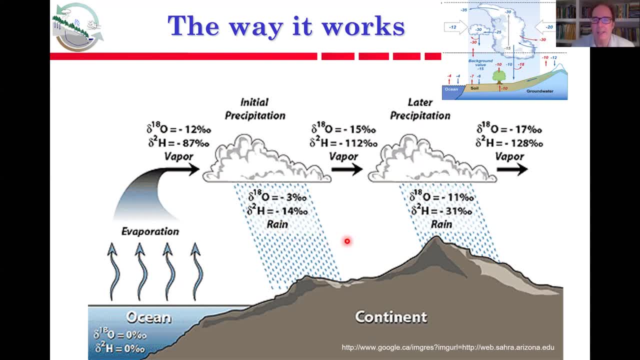 These patterns now are well known globally And they vary from equator to pole, They vary from sea level to Mount Everest or up into the Tibetan Plateau, And these patterns are really important because it helps to understand what the input is to your system. 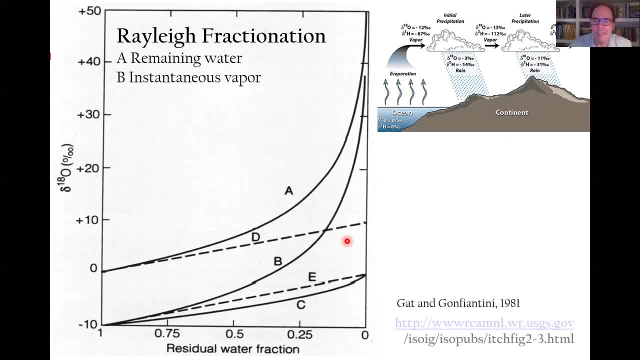 And here's a reference from 1981.. For many decades now we understand these processes. I'm just going to show you this one. I'm just going to show you this one last graph, just to talk about these basics. So let's say we have a glass of water. 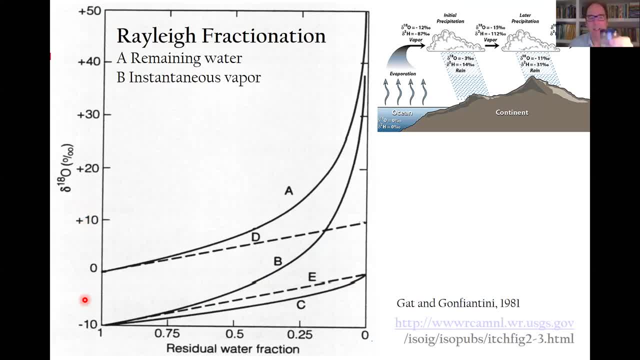 So a glass of water- if you can see my water glass, it's full, And full means residual water, fraction of one here on the x-axis, And if it was empty it would be zero, meaning all the water would have evaporated. 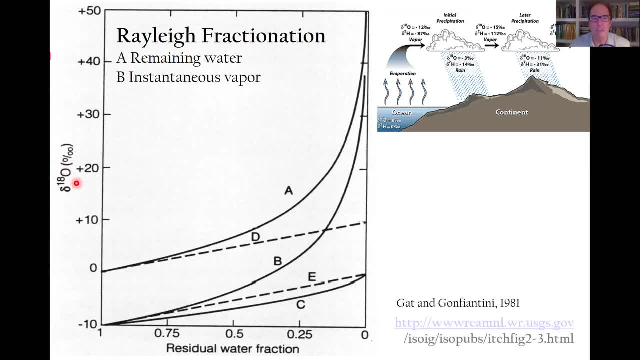 And on the y-axis is the O18 composition in per mil. So only look at lines A and B. So let's start off with the water. I took this out of the ocean. let's just say: And it's zero per mil. 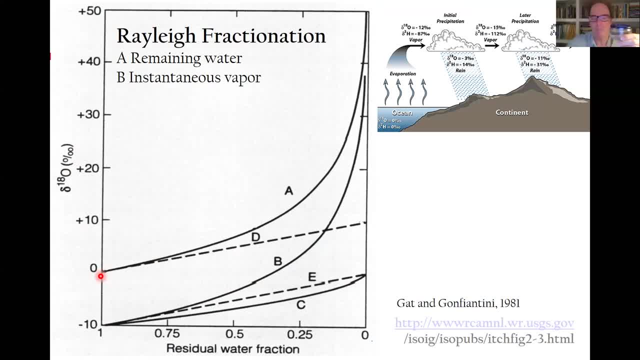 And the vapor that's forming above this glass is already minus 10 per mil. This is a fractionation factor that's known for different systems at different temperatures. Then, as the water disappears due to evaporation- and I'll just form an experiment here- 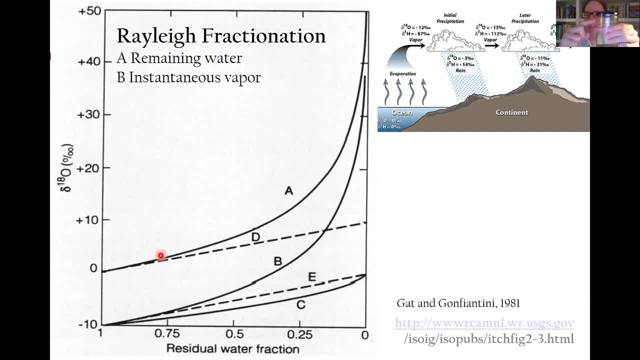 So now the glass has lost water to the atmosphere And let's say it's half full, 50%. Now the water is here in: A, That's the residual water fraction, And B is the instantaneous vapor above it. It's tracking perfectly. 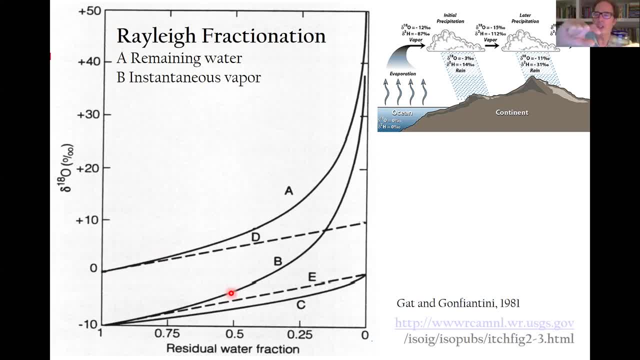 So it's maintaining that 10 per mil difference all the way through. So these relationships, this is for an open system. You can track in both directions And these things are able to be modeled mathematically And there are equations for how things change through evaporation. 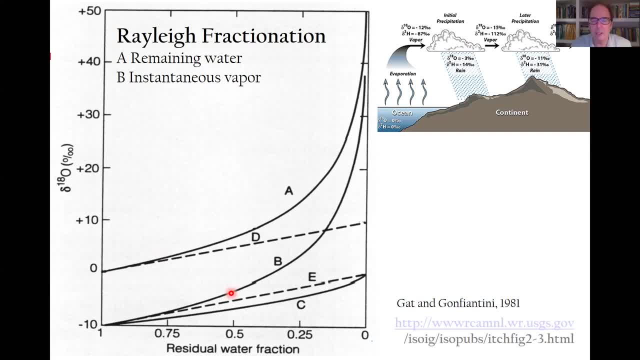 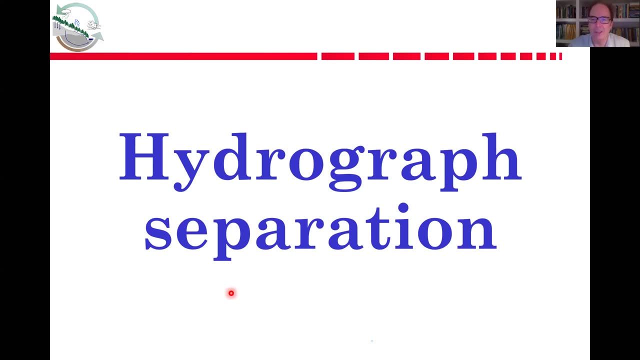 If some of you are working in this area, you'll know of the Craig and Gordon model and other quantitative approaches to understand these so-called fractionation processes. Okay, so back to hydrology. Why are we doing this? Well, hydrograph separation. 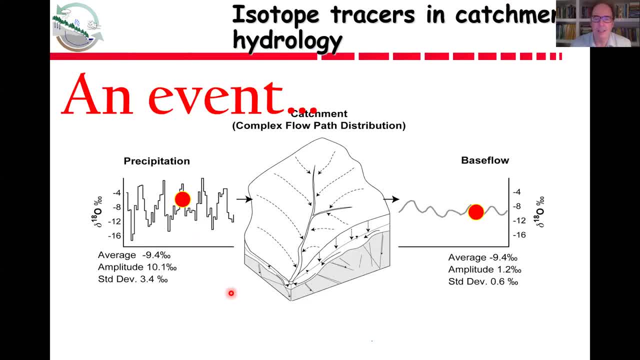 This is the thing that we want to do. Let's say we have a single event. Remember this was a multi-year time series. It's light in the winter, It's heavier in the summer, So this is showing you six or seven years. 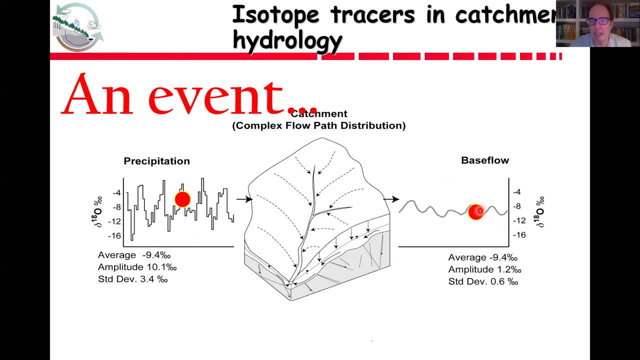 Let's take one event, And we want to understand for that one event, in terms of stream flow, what was the blend of water in terms of the rainfall that generated that event and the water that was somehow pushed out of the basin in this pressure, wave-like manner that I talked about earlier? 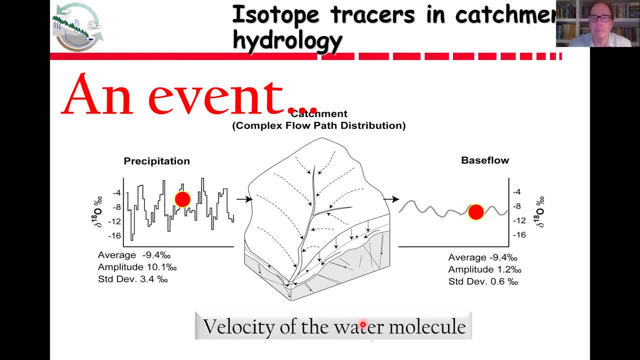 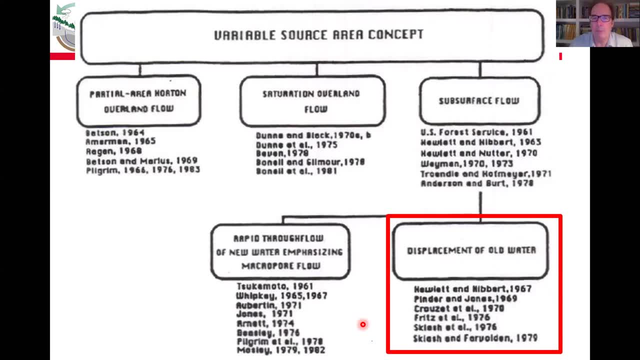 So this is what we're going to do now. Look at one event, And we're going to think about this in the context of what we talked about last class. Remember, we're in the context of the variable source area concept. We talked about infiltration, excess overland flow on partial areas. 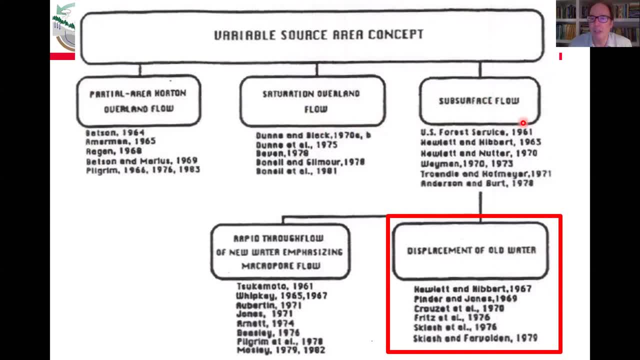 We talked about saturation overland flow, We talked about subsurface storm flow, But there are really two schools of thought in terms of the rapid generation of through flow, with rainwater moving through macropores, or these papers that started to think about the displacement of old water. 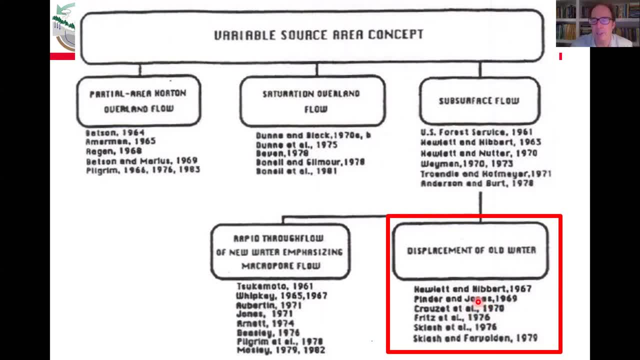 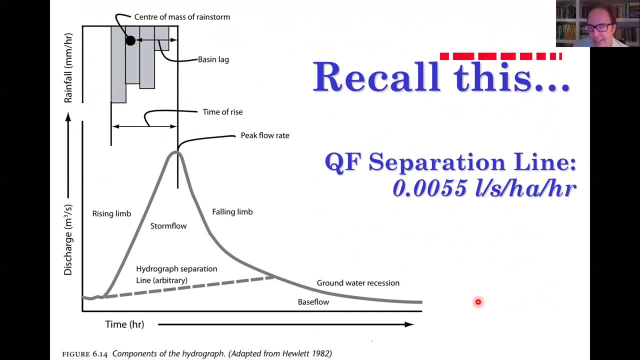 This is what we're going to explore with our hydrographs. So remember the hydrograph. I talked about this last class. This is the storm hydrograph. of course, You all know this discharge versus time. Here's rainfall. And remember Hewlett and Hibbert gave us this thing called the quick flow separation line. 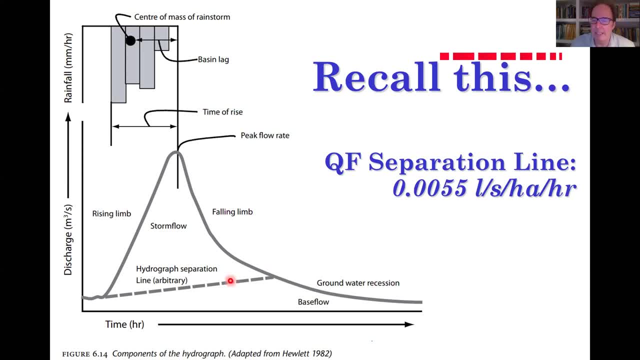 But it's a graphical separation. It doesn't really have any physical meaning. It's just a line projected at a certain slope until it intersects the following line And we call this quick flow, We call this delayed flow or base flow. Isotope, hydrograph separation or separating with tracers is different. 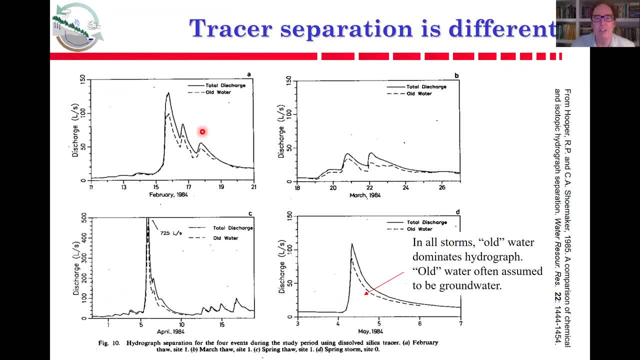 What that does is it takes the hydrograph. Here you're seeing four different periods from a classic paper of Rick Hooper- back in the early 1980s, I believe- And what you're seeing is the hydrograph is now separated and all of the water below that dashed line. 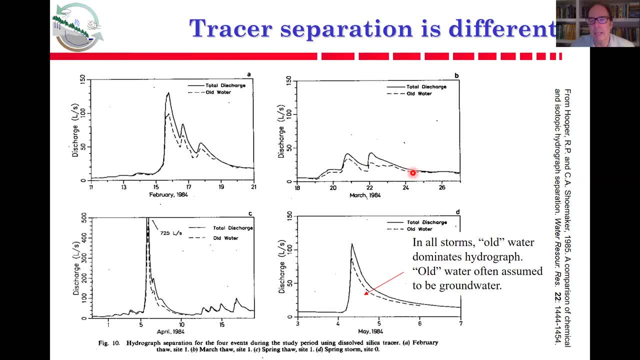 is water that was stored in the catchment before it started raining. It's often called old water And the water above it, meaning between that solid line and the dashed line, is the new water, the water that was contributed by the storm rainfall event. 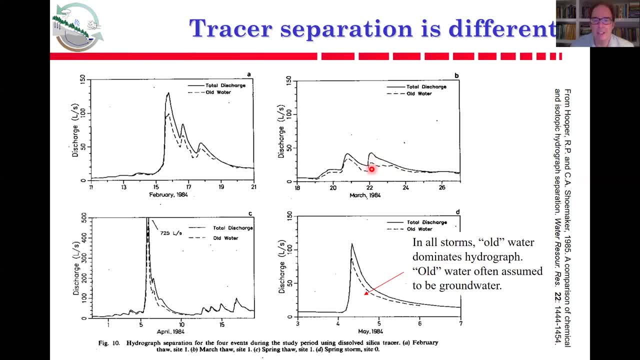 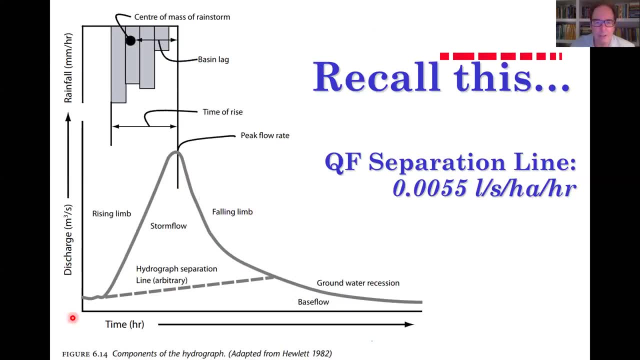 And what you're seeing already is that these lines look very different to the kind of quick flow separation line. This is saying, wow, there's a lot of quick flow And there's a little bit of base flow. But if we did that same separation here, 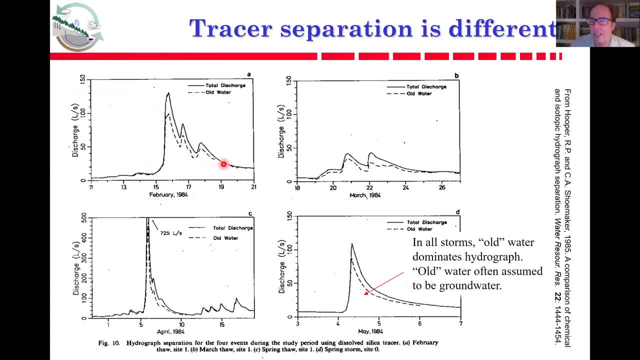 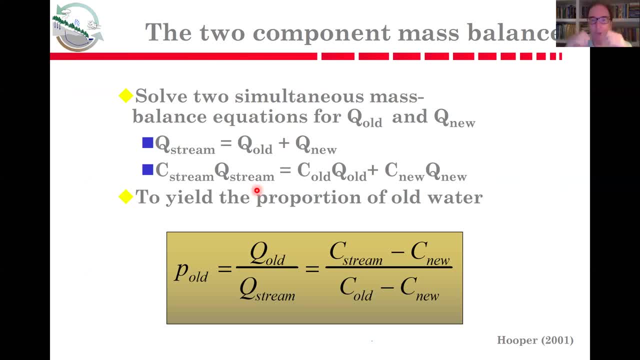 we would say that of that quick flow gosh, most of that looks like old water. What's going on? So the way we're doing this is using a simple two-component mass balance mixing model. We have stream flow. The volume of stream flow is the volume of the old and new water. 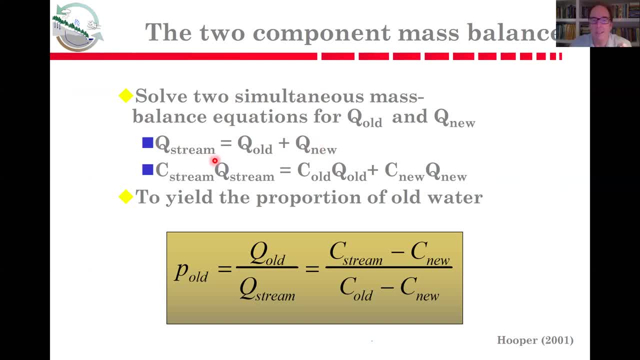 And because now we understand what isotopes are and we can sample them and we can analyze them on a laser spectrometer. we can get the concentration of stream flow simply by taking a sample. We can take the concentration of the old water by taking a stream sample before it starts raining. 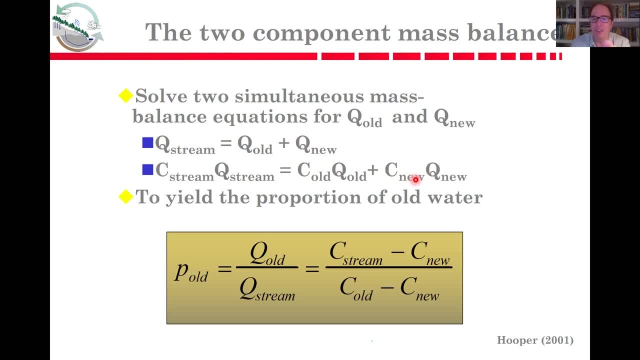 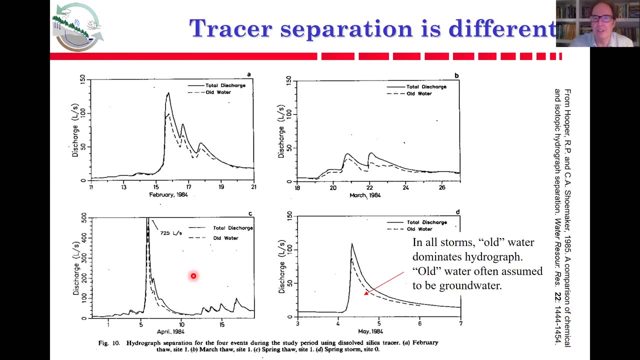 And we can take a sample of the rainfall and we can do these same samples all through the event, And we're simply solving a very simplistic mass balance mixing model that says the percent of old water. then, as I was showing here in these examples from this classic paper by Rick Hooper, 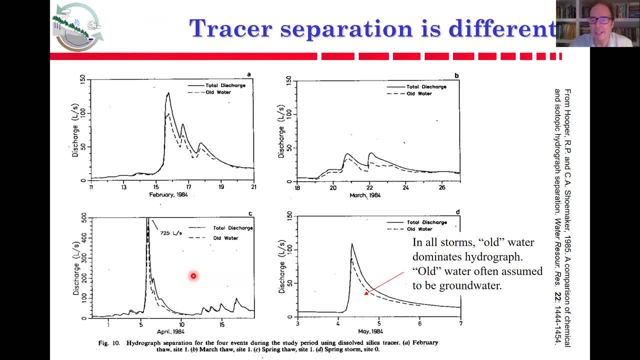 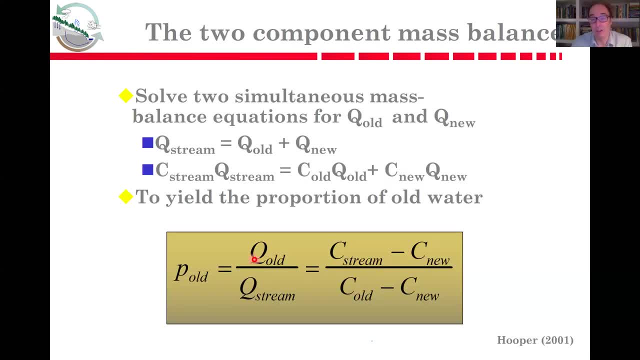 the percent of that old water below that dashed line, that red line is pointing to here. that is the percent of, or the ratio of, the stream water minus the new water over the old water minus the new water, the signature of that. So this is giving us a simple way to take the hydrograph. 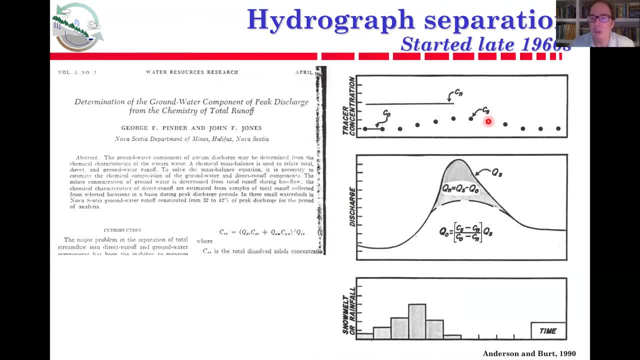 collect some tracer information like the isotope data, and to separate it then into these new and gray and old components. One of the first papers to do this was Pinder and Jones. Pinder was a groundwater hydrologist at Princeton and this was an early paper in 1969. 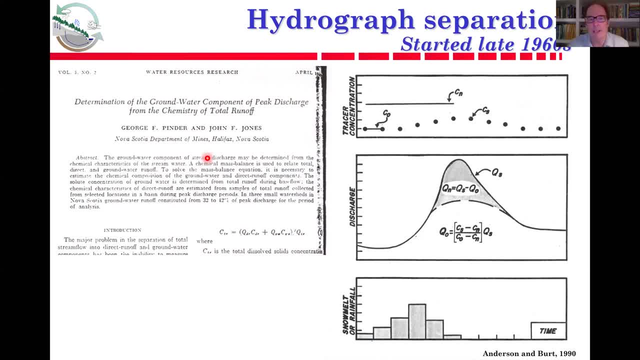 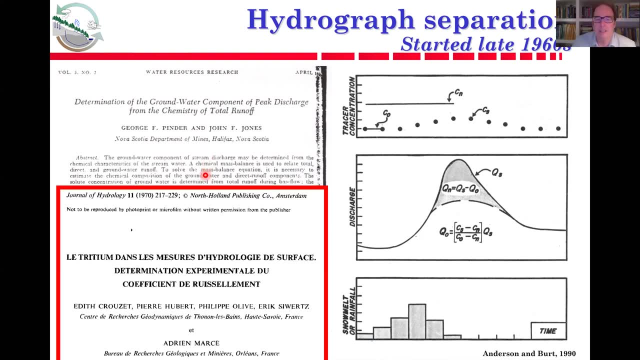 This isn't using isotopes. It was using mostly electrical conductivity and other chemical tracers. The first real isotope hydrograph separation was done by this group, Crouzet and Hubert Pierre. Hubert was the secretary general of the IAHS- International Hydrology. 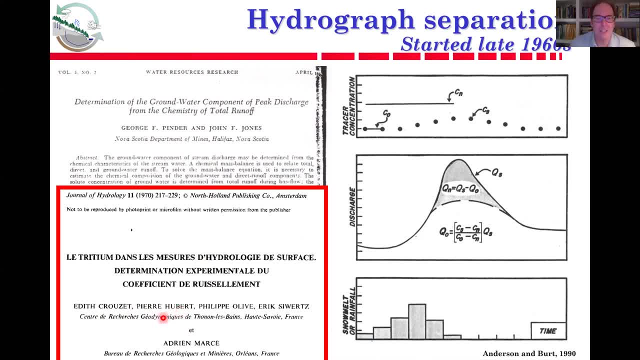 Association of Hydrological Sciences and this was a paper in Journal of Hydrology in 1970. But by 1975, now, several papers were being published and again just showing this kind of ratio. So if it seems confusing, just look at this for a minute. 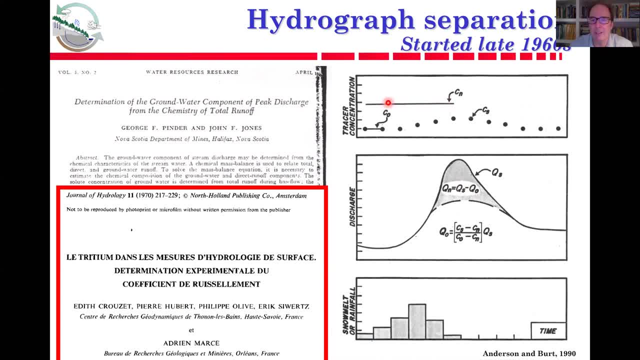 Here's the new water. This is the rainfall. Here's the old water in the stream before the event starts. So all we're talking about is, if we sample the stream water here, here, here it's deflecting towards this rainfall signature and then back again. 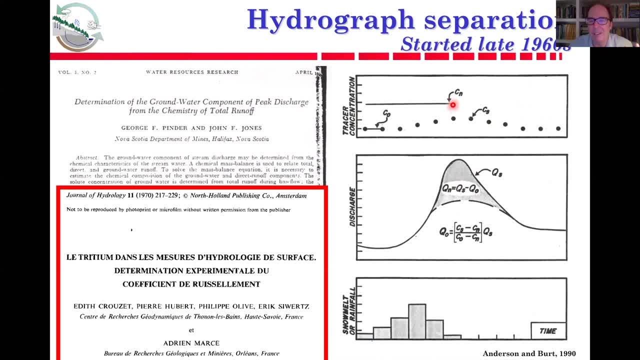 If it gets all the way to touch the rainfall, then at the peak of the event we would say the percent of rainfall is 100%. at the peak of the event, if the stream flow got all the way up and touched here, If the stream flow stayed horizontal the whole way, 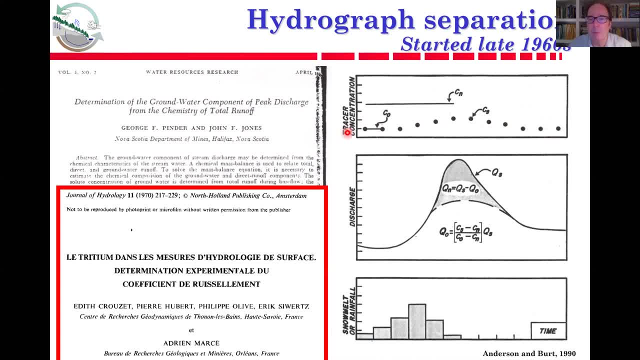 then what would we say? We'd say the opposite. We would say that the stream flow, even at the peak discharge, was 100% old water, And usually it's somewhere in the middle. So that's what this hydrograph separation is. 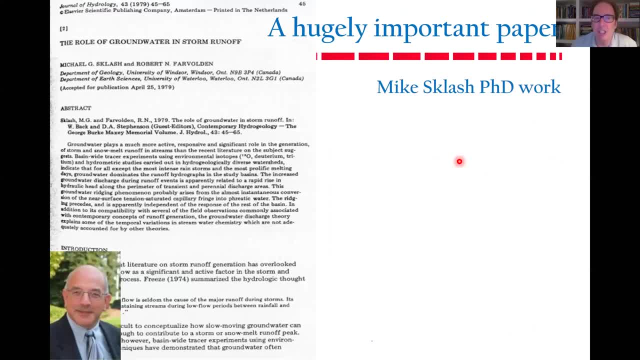 Now, one of the most important papers in this field was this one in 1979 by Mike Sklash. This was his PhD work, published in Journal of Hydrology: The Role of Groundwater in Storm Runoff. Because what he did was not only show hydrograph separations. 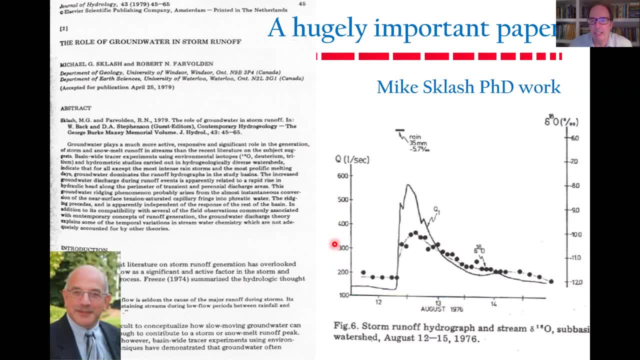 just like I've shown you. So here's one of his sites. This was actually in Canada. This is discharge on the y-axis covering a few days of sampling. Here's the hydrograph And these dots are the 018. composition And the separation of the hydrograph showed that most of the water 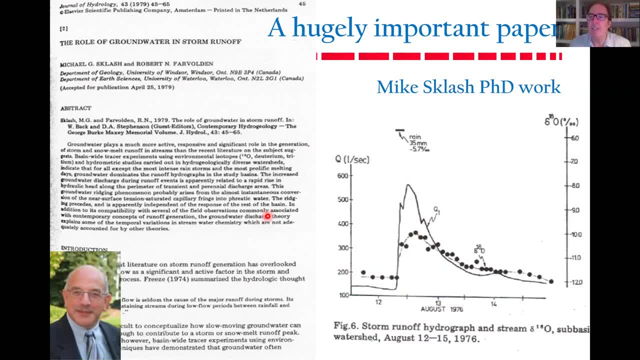 making up the storm hydrograph, even at the peak of discharge, was old water, what he called groundwater water, that was in the catchment or in the hill slope before the rain started. And this was quite important because, in addition to showing this, 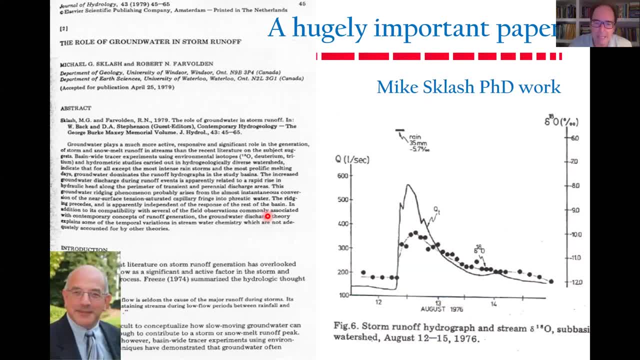 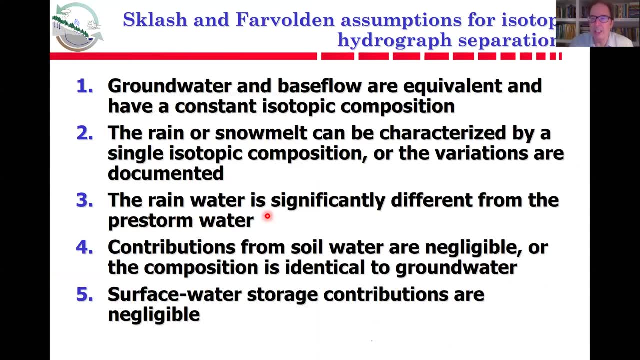 in a very compelling way for many storms, many catchments. he also laid out many of the assumptions we continue to use today in doing this: hydrograph separation, The idea that the water in the stream and the groundwater are equivalent at the start of the event. 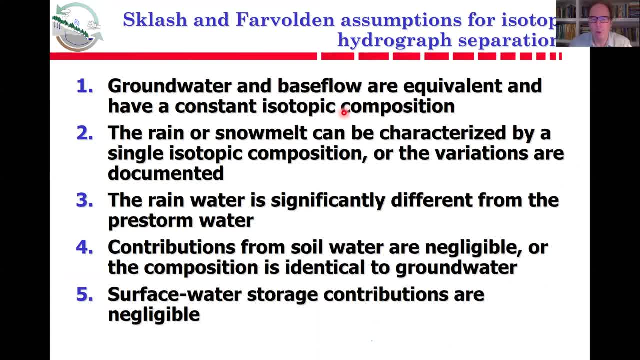 So that's why we can use the old water composition as equivalent to the stream flow before the rain starts falling. The rain or snowmelt can be characterized by a single isotope composition or variation they're documenting. So this means that if you have only one sample of precipitation, 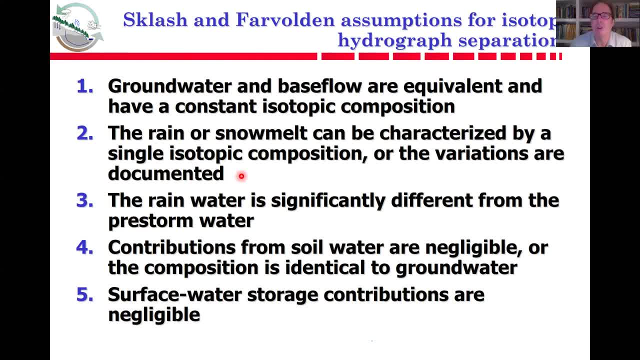 it's representative of the whole event. Of course, this varies a bit through the event and in some cases quite a lot, And I'll show you an example of that in a minute. A key assumption, in fact really a requirement for the whole thing. 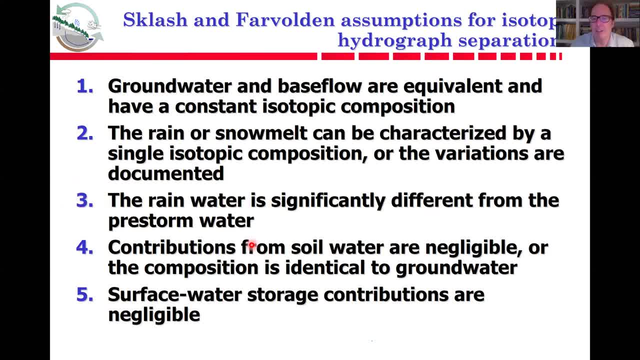 is number three. The rainwater is significantly different from the pre-storm water And, in fact, very nice work on uncertainty of these hydrograph separations. that was started by a paper in Water Resources Research in 1998 by Dave Gennaro. 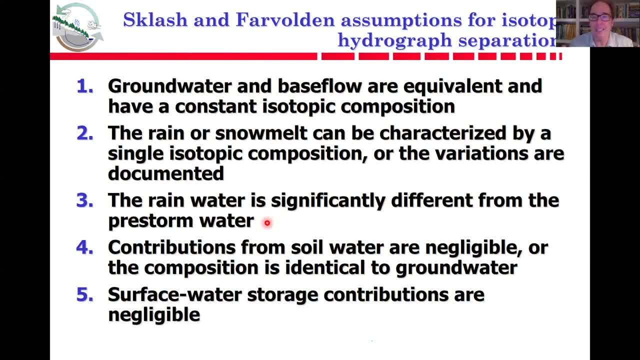 He showed very nicely that basically the uncertainty decreases the farther away the rainfall is from the pre-event water. So the greater the difference in the signal, the better. for this technique, Contributions from soil water are negligible and surface water contributions are negligible, And we'll talk more about this number five in the lecture number four. 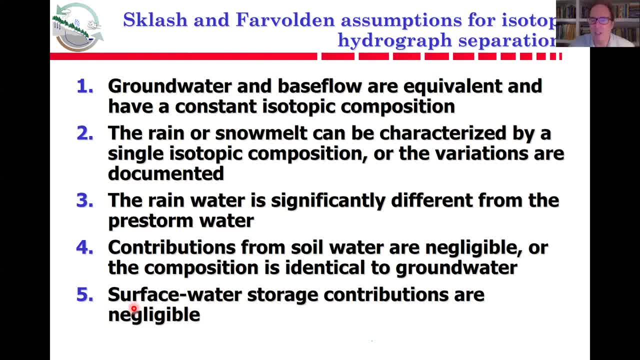 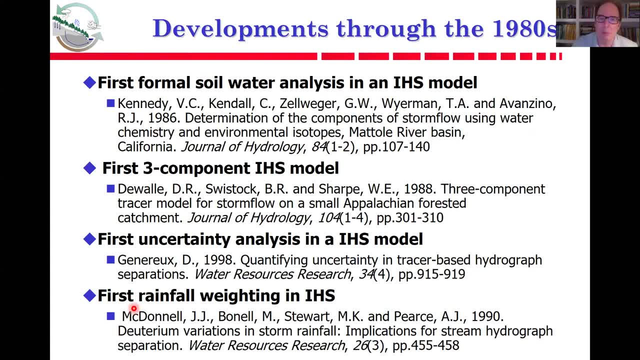 This is due to evaporation and some of those fractionation effects I talked about earlier. Now I won't burden you with much more detail, but if you're interested, there are- and you're doing this work, possibly there is a large literature that I can kind of help guide you through. 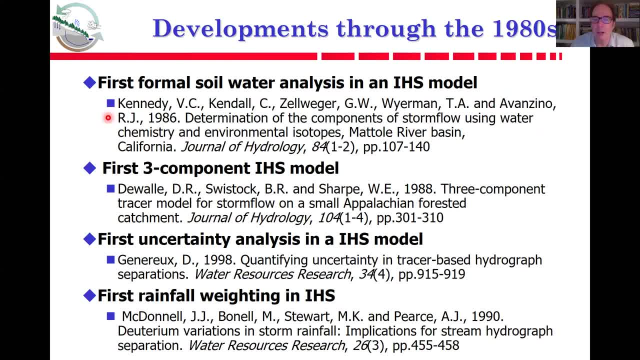 But some early work started to think about the role of soil water in a hydrograph separation. This was the first three-component model in 1988 by Dave DiWally in the Journal of Hydrology. This is that uncertainty paper I mentioned, and then some of the first rainfall weighting. 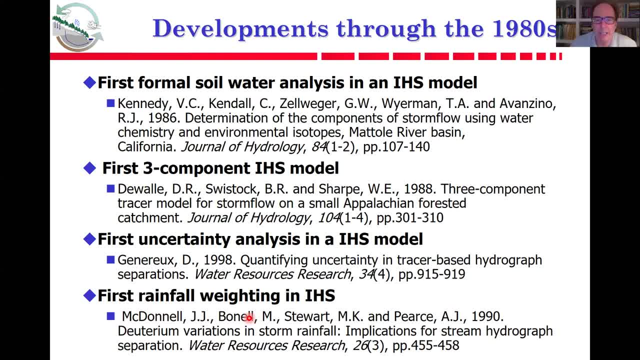 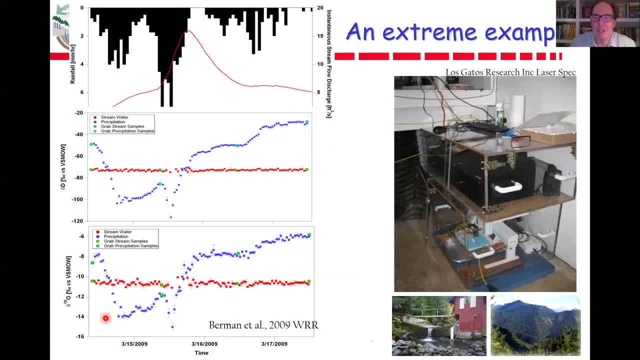 of the varying rainfall signature. I worked on that in my PhD many, many, many years ago. Okay, let me show you an example, And this is from a site in Oregon again, And here this is one of the first applications of in situ sampling. 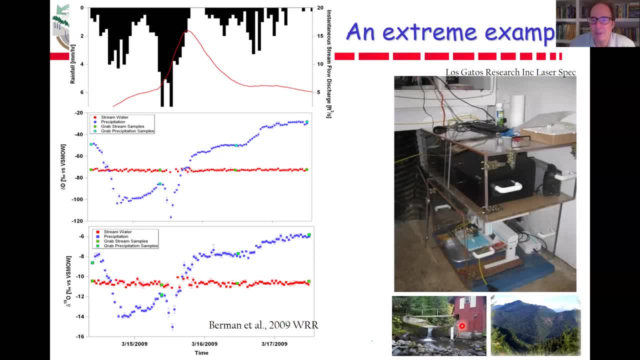 So this is now 2009.. And we went to this catchment and we brought the laser spec with us And our objective was to sample in high frequency And you can see here those dots in blue and red. they're every 20 minutes or so through this three-day period. 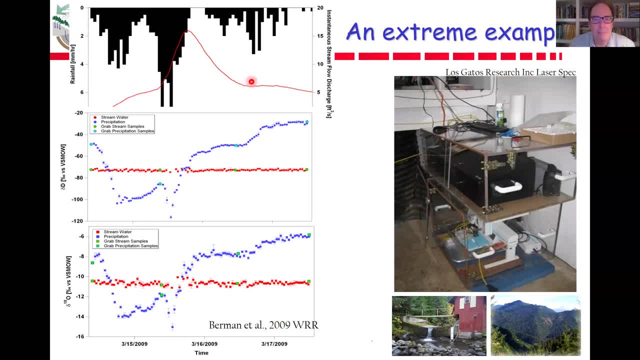 So here's the rainfall in black, Here's the runoff- if you can see my pointer- in red covering these three days, And then on the left or the middle plot, that's the deuterium and the O18 is shown here. 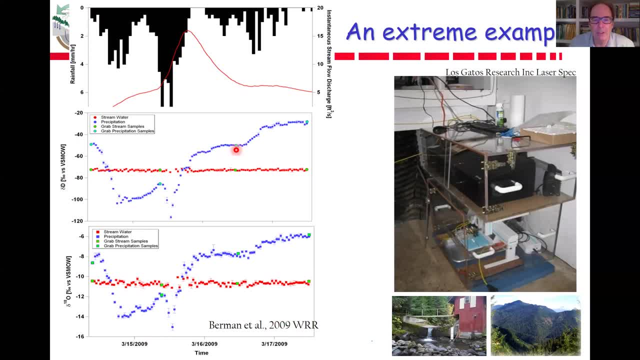 The rainfall is in blue in both of these plots and the streamflow is in red, And this is what we see in this wet, steep area, with a very high runoff ratio being expressed. What do you think this is saying? Going back to what I said about the rainfall, 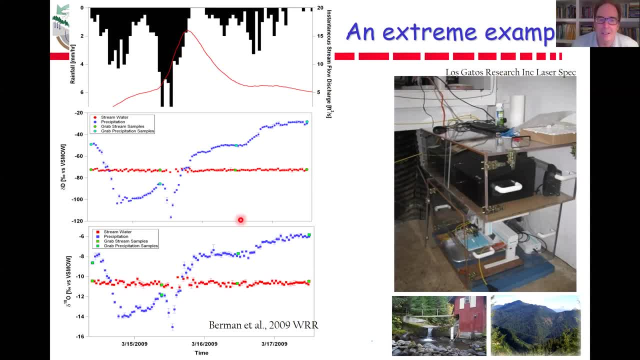 being touched by the streamflow sample or not. What this is saying is something quite disturbing in the sense that we're still trying to understand this even today, not just in this catchment, but all around the world. What this is saying is that we have a hydrograph. 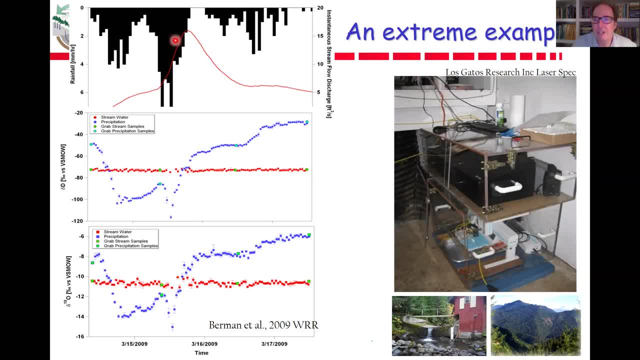 that's going up and down with a fairly high runoff ratio, meaning the amount of runoff relative to the amount of rain input. But look at the stream isotope signal: It's unchanging. What that is saying is that even at the peak of the runoff, 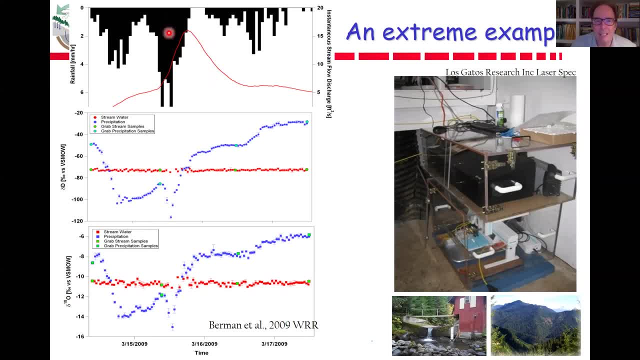 there's no detectable rainfall in the stream. All of this water is this displaced water that was in the catchment before the rain event started. This is that old water paradox. but of course it's not really a paradox, It's just those very different expressions of velocities. 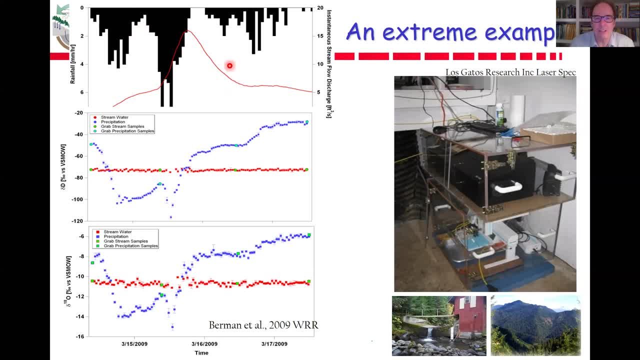 in terms of the celerity that represents the hydrograph versus the water, the water particle velocity as expressed by the stable isotopes. Now, if you're a hydrological modeler, I dare you to try to capture this in your model. 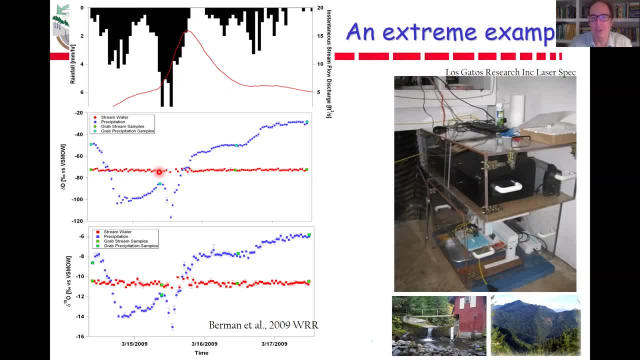 You really need to have both of those pieces to be able to capture these two signals And, of course, these two signals are quite important for many of the modern environmental problems that we're concerned about. So we're going to be looking at how the current use change impacts. 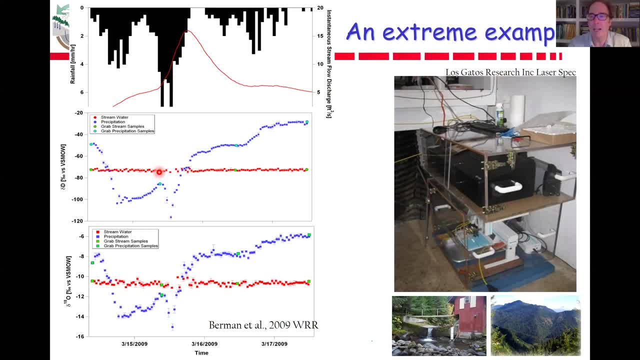 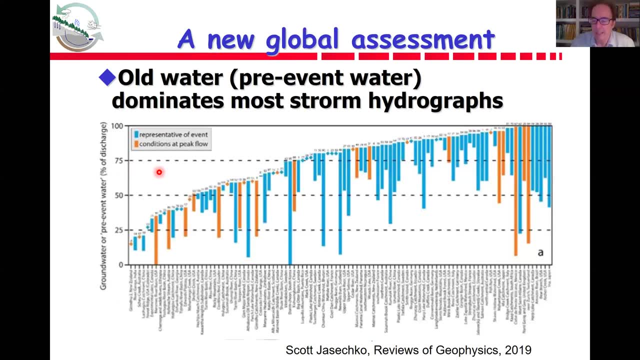 how nitrate moves through a landscape and when it will appear in the stream That's affected by these velocity of the water molecule, not just the celerity, the hydraulic potential, And if we do a global assessment of all the papers that have done hydrograph separations. 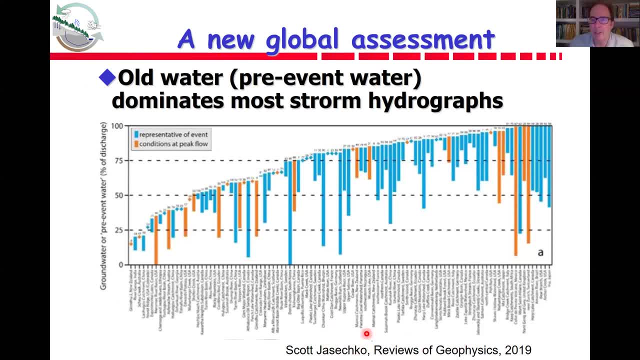 this is a really lovely paper in reviews of geophysics and the results of the studies And it's a really interesting paper. It's called the CECO. This is what it shows If we look at the pre-event water on the y-axis. 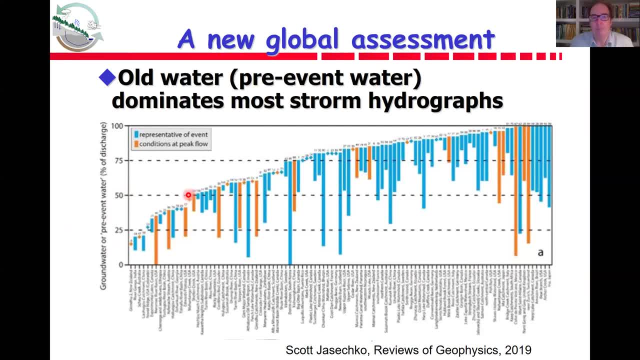 and we look at all these studies. what this is saying is that most of the studies, half of them, have pre-event water dominating. Half of the studies are showing 75% or more of pre-event water in the storm hydrograph. You know, look at all of these studies. 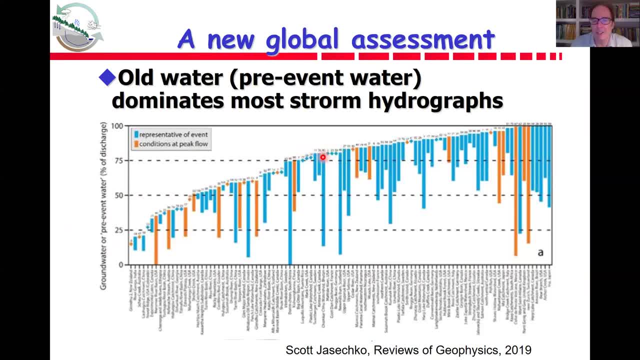 showing these very, very high old water fractions. This is saying that it's very common to have this dominance of old water. now, in the decades of work that's been done since the mid-1970s until this review was made, Old water dominates most of these hydrographs. 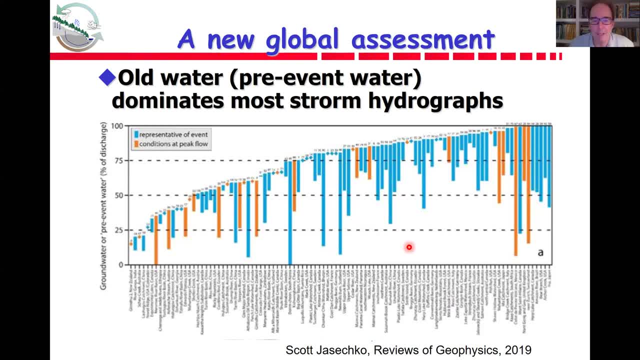 Now, of course, there are exceptions. In Canada, where I am, we get snow melt onto frozen ground That runs off the surface And we see 100% new water or no old water, And the same would be true on a parking lot. 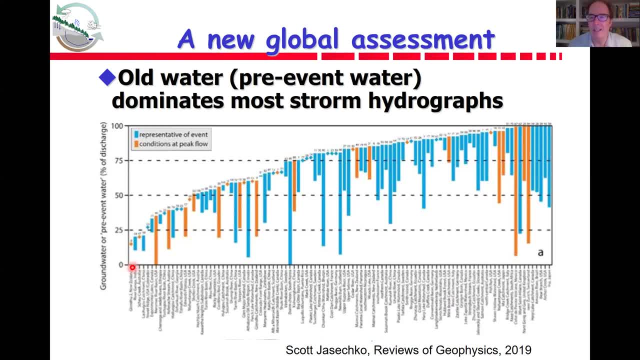 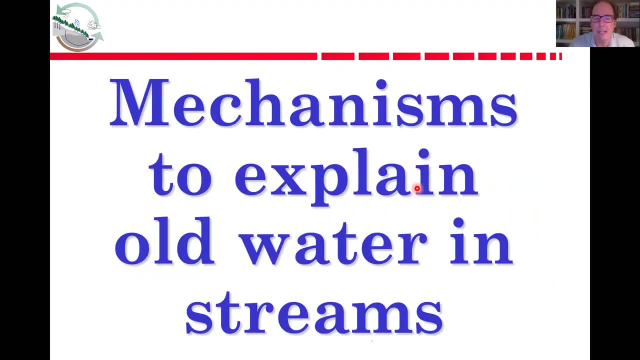 or maybe in an urban area in Beijing where you've got a lot of paved surfaces. But these are natural catchments for the most part, showing that under this collection of studies, most are showing dominance of old water. Now, the last thing I want to cover is 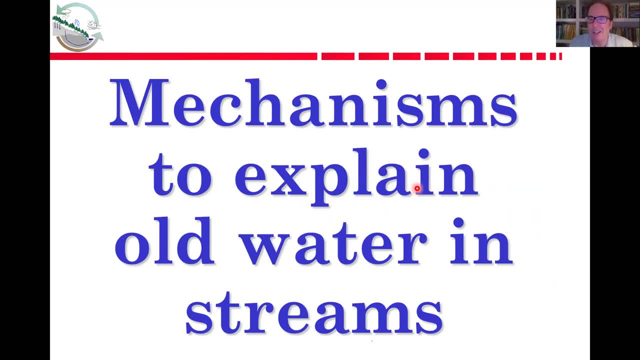 how does this work? How do you get all this old water out so fast? This was what people were asking even in the mid-1970s, when these first data were being shown, because it made no sense to anyone. You think of rain falling on the surface. 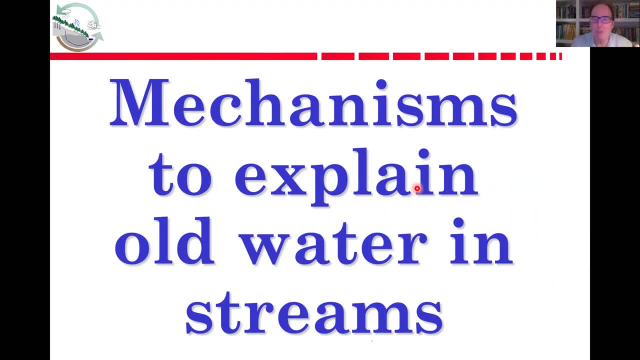 like Horton's early work and you look at the overland flow velocity. Of course Professor Pan looks at overland flow velocities for soil erosion work. It's very fast, But groundwater moving through a porous media, these are much, much slower. 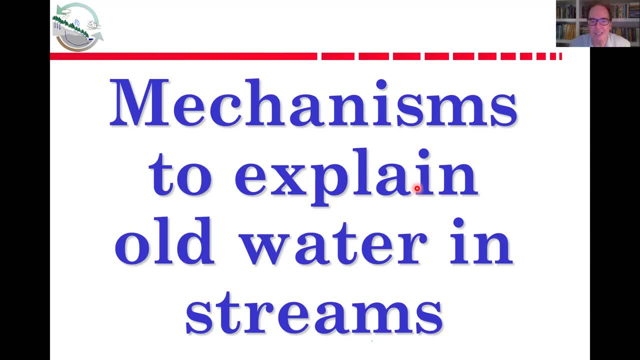 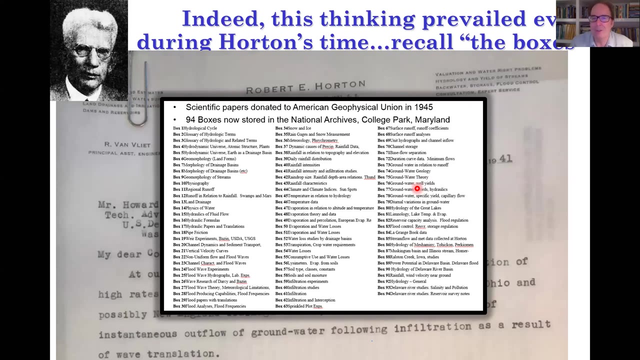 Think of saturated hydraulic conductivity of soil or rock or glacial till. These aren't meters per second, These are more millimeters per day. How does this work? Indeed, this was even something Horton was concerned about- not in terms of isotope data. 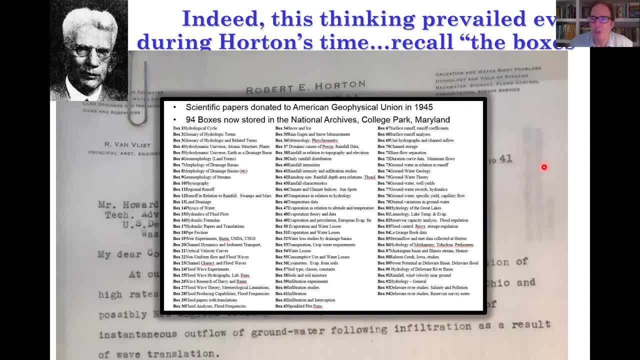 because back in the 1940s people weren't doing isotope tracing in hydrology. But this is a letter that I found in these boxes I mentioned Again. there are these 94 boxes of Horton's papers at the National Archives just outside of Washington DC. 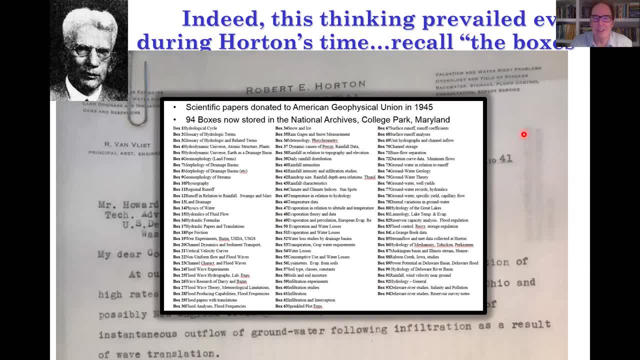 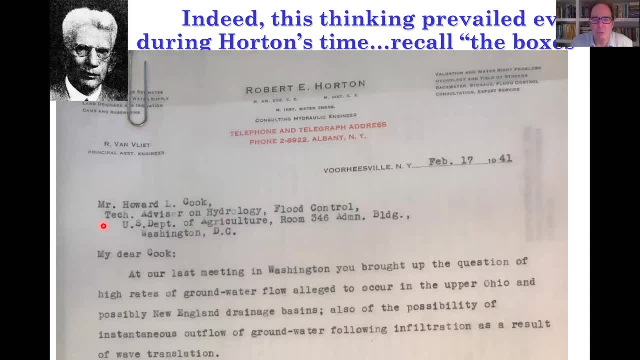 And this was a letter I found in his archives and it was addressed to this Howard Cook. This is the same Cook that we read from in Keith Bevan's paper last class, when talking about the era of infiltration. And here is Horton on his stationary. 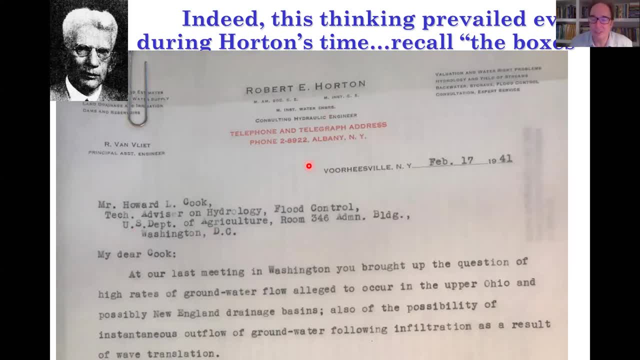 He was a consulting hydrologist and researcher and probably our most famous hydrologist ever in the field, And he's writing: Cook in 1941, and he's saying: at our last meeting in Washington you brought up the question of high rates of groundwater flow. 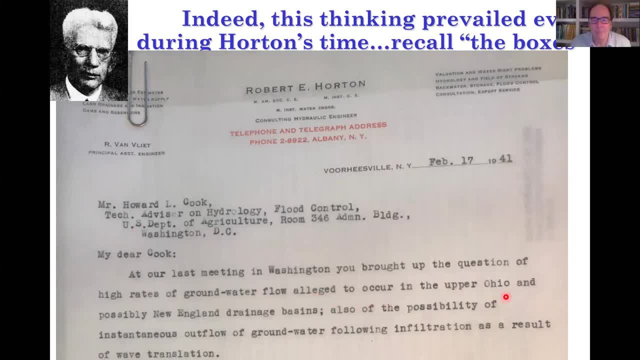 alleged to occur in the upper Ohio- this is a river basin- and possibly New England drainage basins and also the possibility of instantaneous outflow of groundwater following infiltration as a result of wave translation. So I'll just look. This is now going on to page two. 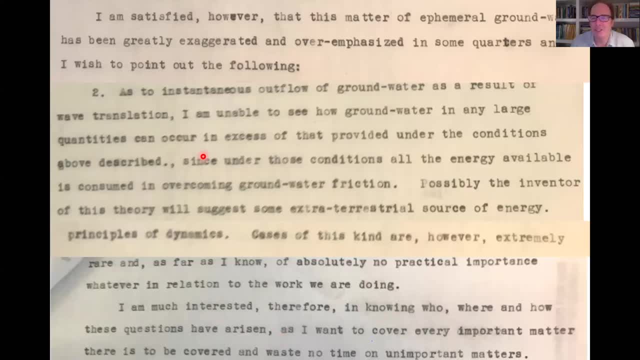 where I grabbed a couple of sentences just to show you. So here's Horton saying. I am satisfied, however, that this matter of ephemeral groundwater has been highly or greatly exaggerated and over-emphasized in some quarters, And I wish to point out the following. 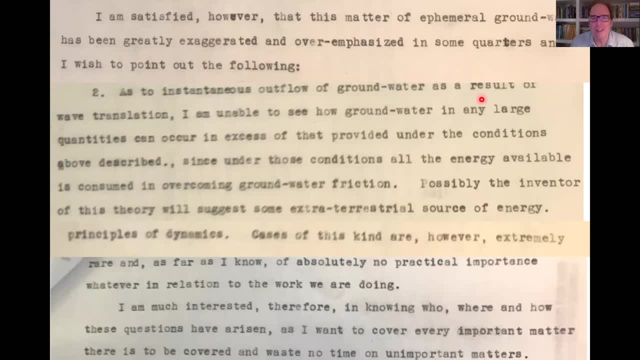 As to the instantaneous outflow of groundwater as a result of wave translation, I am unable to see how groundwater in any large quantities can occur in excess of that provided under the conditions above described, Since under those conditions, all the energy available is consumed in overcoming groundwater friction. 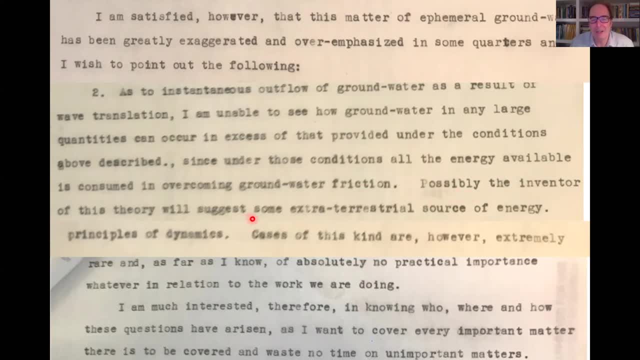 I love this sentence. Possibly the inventor of this theory will suggest some extraterrestrial source of energy. And here's he's saying: cases of this are extremely rare, as far as I know, and of absolutely no practical importance whatsoever in relation to the work we're doing. 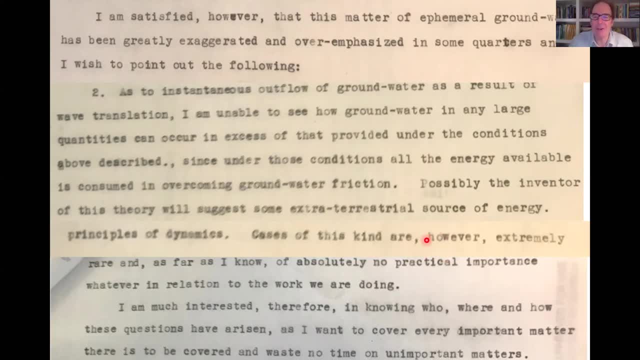 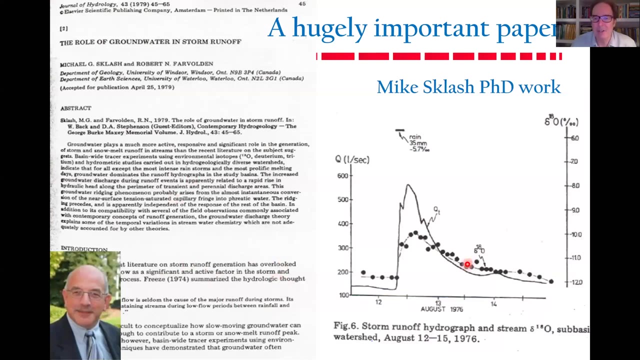 So this is strong words, Strong words from Horton on a topic that was to become probably the topic in hill slope hydrology in the last couple of decades. Because again we go back to this work of Sklash and the hydrograph separation work. 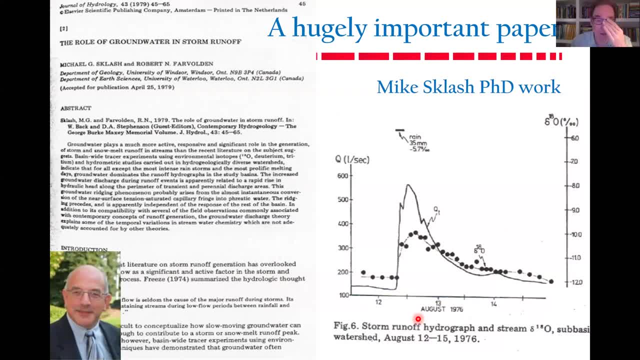 How is this happening? How is groundwater being moved so quickly into the stream? It's still mysterious, And it's certainly mysterious to Horton in that letter. So let's read from this abstract here in this paper: I just wanna- I'm gonna increase it so you can maybe see it. 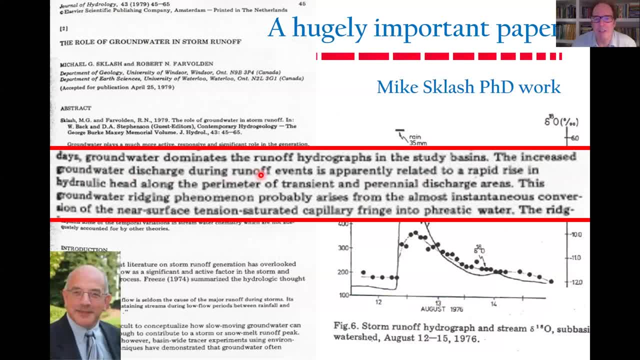 The increased groundwater discharge during runoff events is apparently related. So here he's explaining it. It's related to the rapid rise in hydraulic head along the perimeter of transient and perennial discharge areas. This groundwater reaching phenomenon probably arises from the almost instant instantaneous conversion of the near surface. 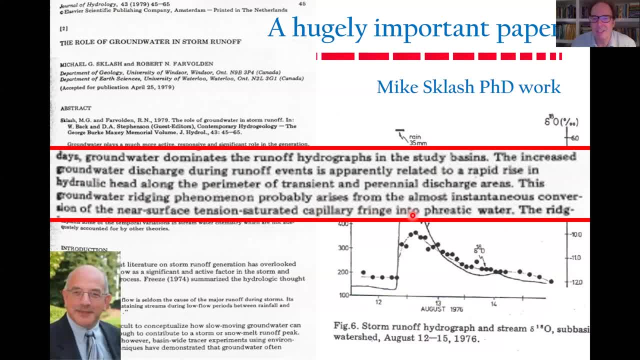 tension saturated capillary fringe into phreatic water. So there's some big words there. Let's try to understand what he's getting at. He's calling it groundwater ridging. What is groundwater ridging? Here's where Sklash was working. 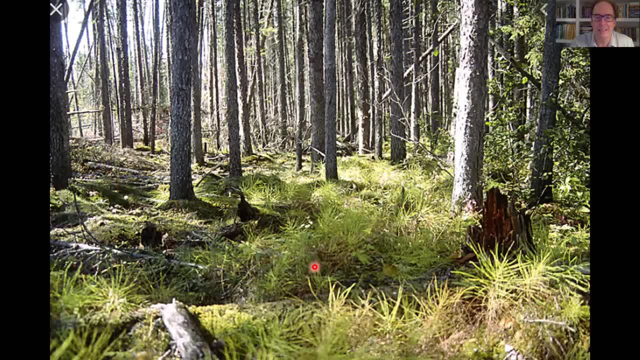 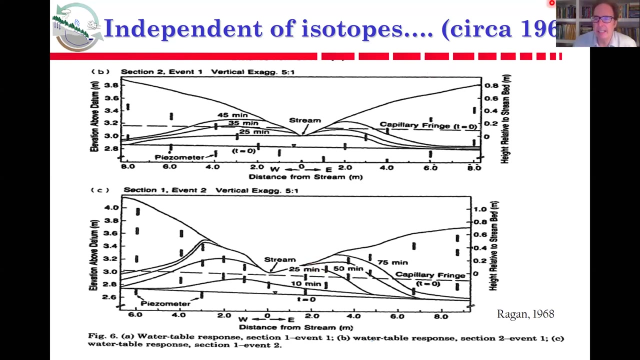 These are forested basins in Southern Quebec in Ontario, Not very steep, poorly drained soils, where largely these are glaciated catchments. So there's soil on top of till glacial, till And before Sklash's work, even in the late 1960s. 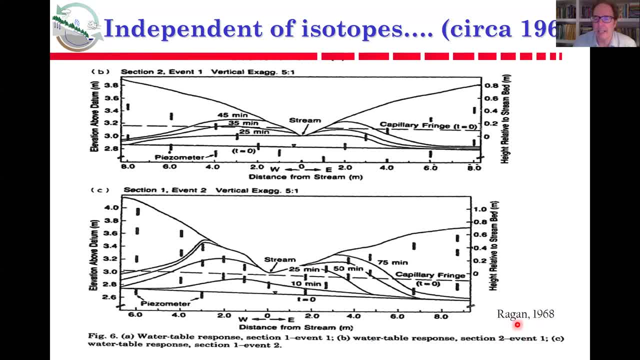 papers were coming out like this one. This is by a Professor Reagan in University of Maryland, And this is showing you a stream, cross section. There's the land surface And time equals zero is shown here where the water table is horizontal, So it's below the stream. 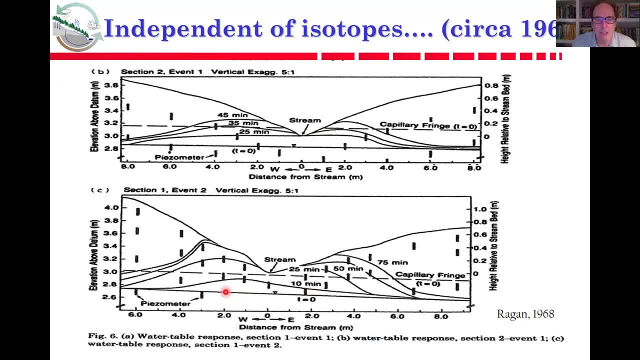 Stream is losing. here And here's time zero. in this other example, The water table is below the stream And what you see is, during a rain event, what happens? The water table starts to rise very quickly, And by 45 minutes. 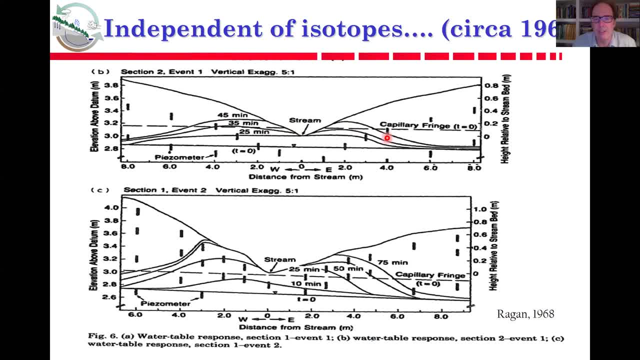 you've got this mound or ridge of groundwater next to the stream And that's because this zone of tension saturation, the capillary fringe. this is derived from the moisture release curve. It means that there's very little storage near the stream. And if this capillary fringe 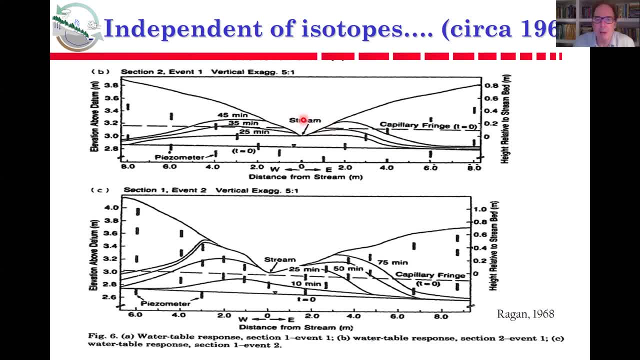 extends to the ground surface. you only need a small amount of water to fall in this area near the stream for the water table to rise And with the rise in water table, the hydraulic gradients towards the stream, just like we calculate with tensiometers. 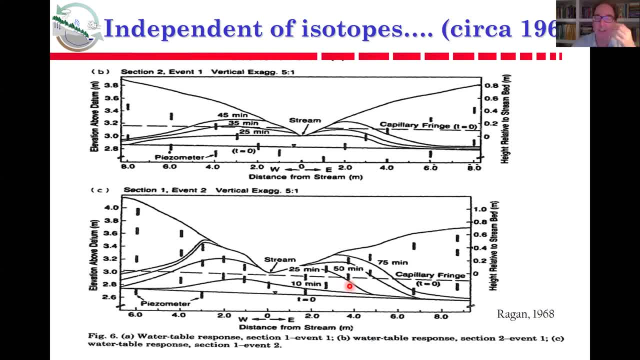 remember hydraulic gradient are the contours, contours of total potential. Total potential is matrix potential plus elevational potential. So what we're doing is providing a mechanism to release groundwater, old water, into the stream quite quickly. So this is what Sklash was talking about. 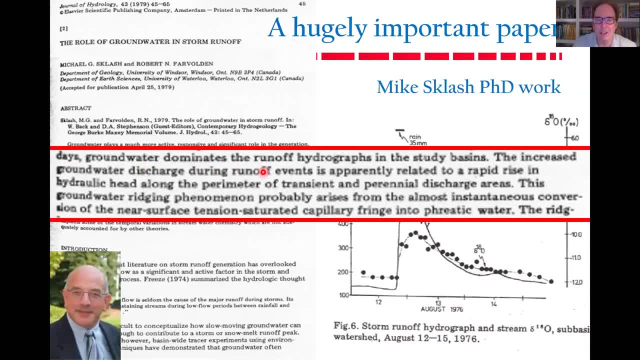 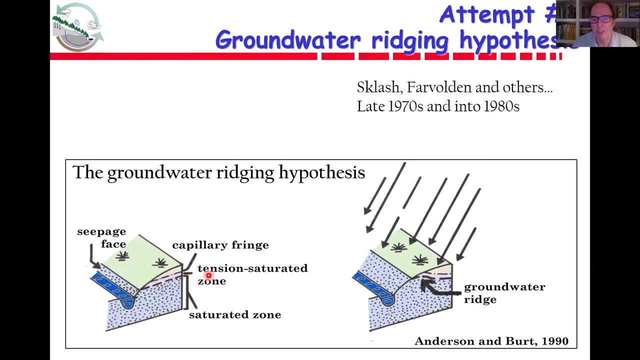 when he talked about groundwater discharge and groundwater ridging around the stream channel. Let's look in a little more detail. This is what we're saying: that next to the stream we've got a water table, and above the water table is this so-called tension, saturated zone or capillary fringe. 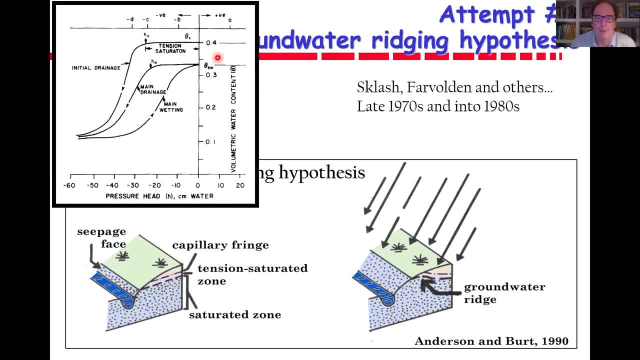 Let's go back to soil, physics basics, Water content here, matrix potential on this axis in centimeters of water. So we're getting, we're pulling tension in this direction. This is at saturation here, or here This flat part of the stream. 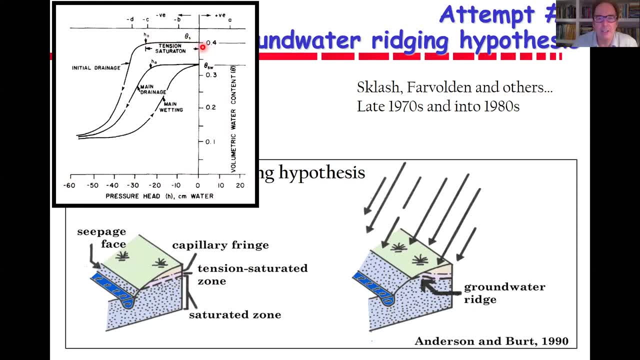 of the curve is the tension saturated zone. So if this is the drainage curve, what this means is we're pulling tension but it's still effectively saturated. Or if we're looking at the main wetting and drying curve or the main, this zone of tension saturation. 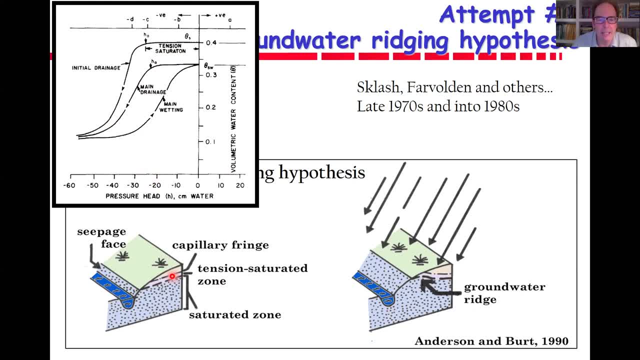 in this case it would be about 25 centimeters or so. That's the thickness, then, of that capillary fringe. So what happens? We get rainfall onto this near stream zone. If the capillary fringe extends to the ground surface, water table rises almost instantaneously. 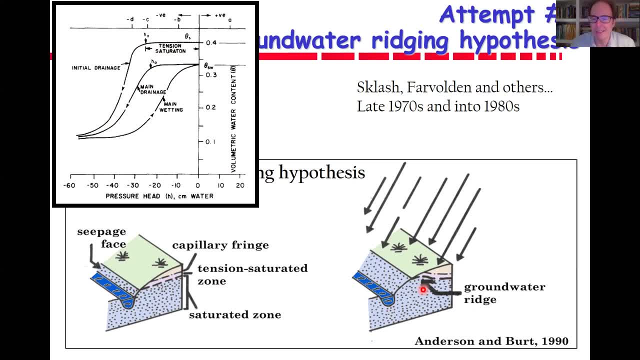 The thing that Horton thought was not possible is because there's no storage And then you create those steepened hydraulic gradients based on that ridging. So this was the first attempt to explain how you could get all of that old water, as it were. 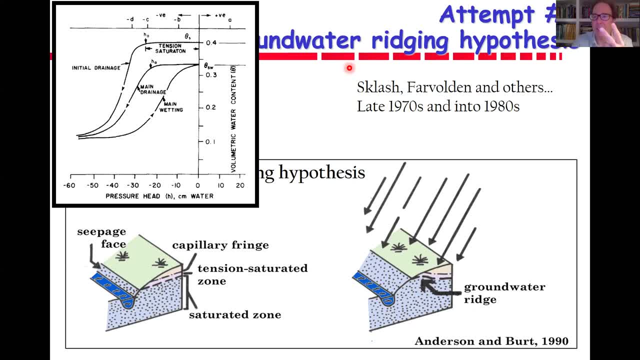 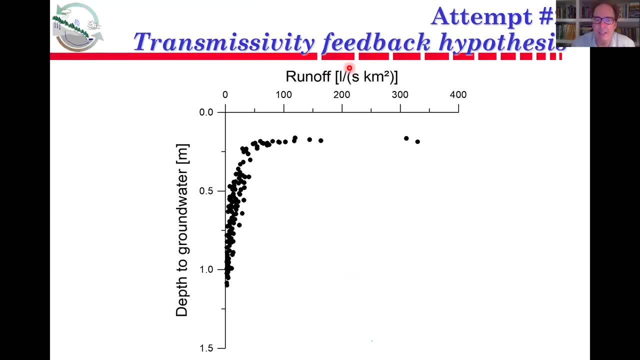 quickly into the stream channel. The second one, early on now- this is in the 70s and 80s- was coming from Scandinavia and Sweden in particular, And this was called the transmissivity feedback hypothesis. So this is another mechanism. 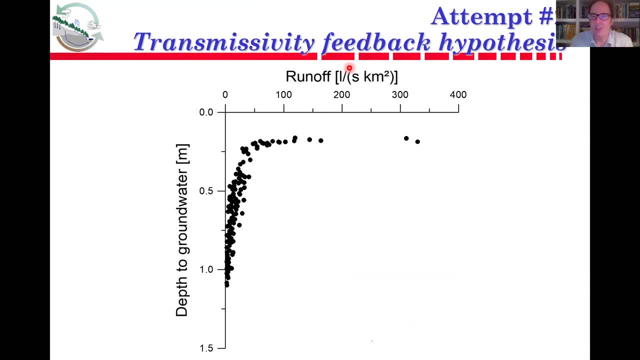 to release old water quickly in the stream. This is some lovely work by Alan Rhoda, who's now retired from Uppsala University, But here's depth to groundwater So zero would be the surface of the soil, and we're going down about a meter and a half. 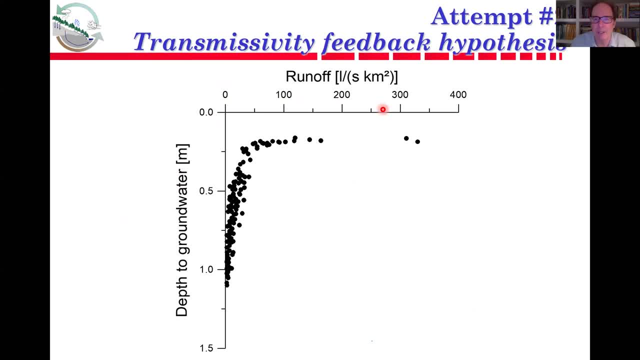 here And on this axis is runoff. So look at this relationship by these dots. These are different events that are being plotted here, Highly non-linear, And what it's saying is that when the water table is low, there's very little runoff in the stream channel. 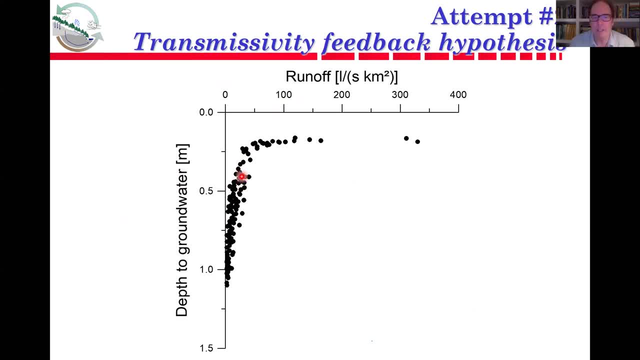 in this small headwater catchment in Sweden. But when the water table gets to a certain height, oh boy, then the stream really turns on. You get very high liters per second per square kilometer flow. Why is that? Well, it's groundwater being released. 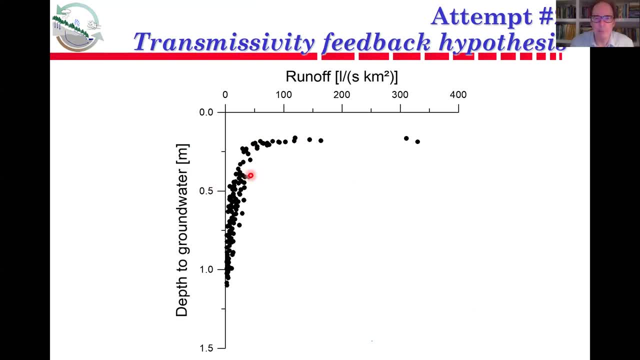 And that's because down here in this part of the subsurface, this is glacial till And on top of that is a much more transmissive, much more permeable forest soil And once the water table rises into that more permeable zone, 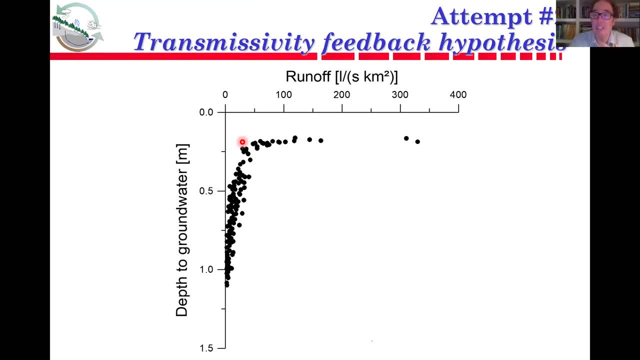 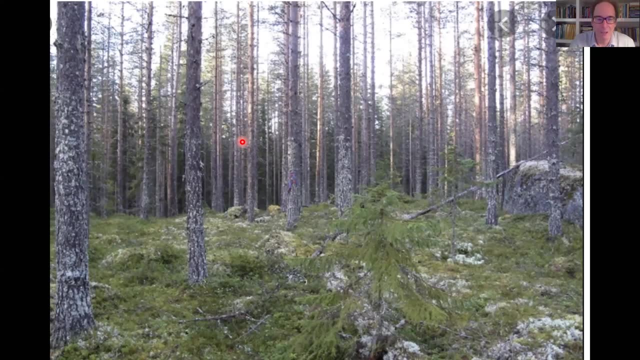 it can move laterally very, very quickly, Basically draining off the top of the water table. Again, these are fairly flat looking areas. This is an area in Northern Sweden where Alan worked, Again glaciated, cold, wet areas And, if we look at a diagram, 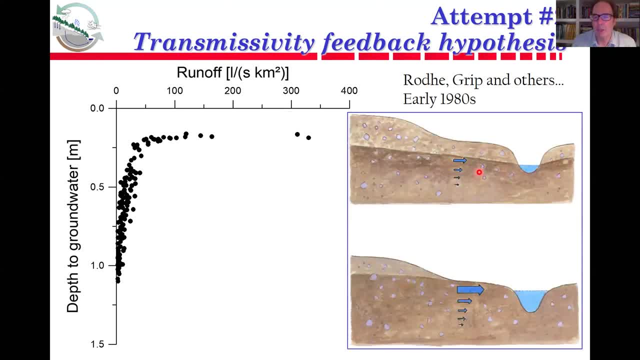 this is the idea that when the water table is low, the flux of water laterally to the stream is low. But when water table rises into this more transmissive mineral soil, then you get very high rates of groundwater transfer from the hill slope to 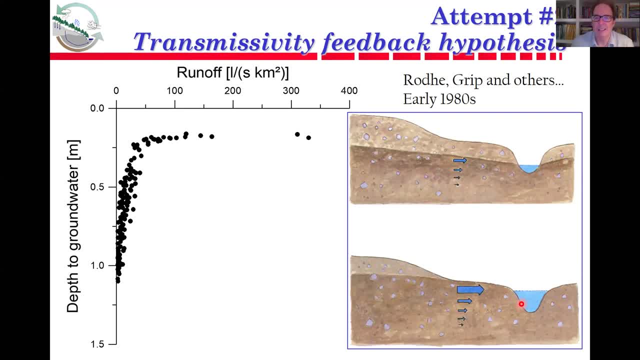 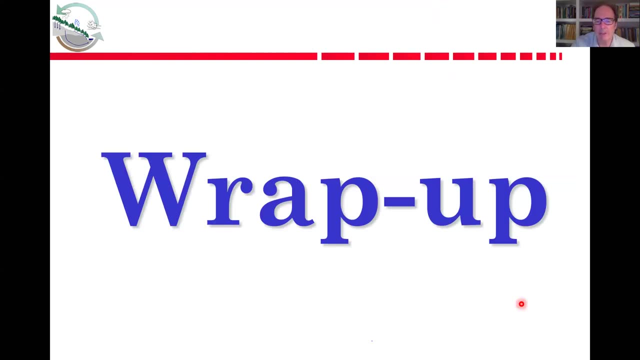 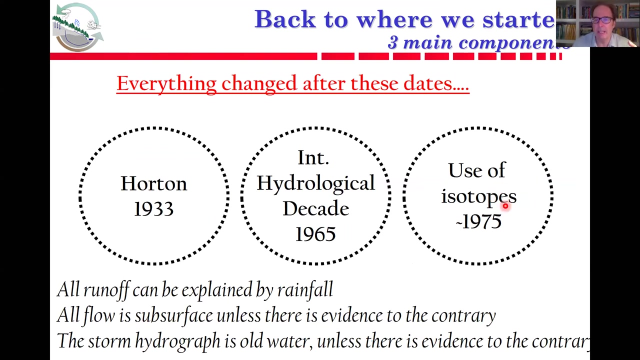 the stream. So this was the second mechanism that was presented when these isotope results were being discovered in the seventies and eighties. Okay, I'm going to wrap up, because this is really the period I wanted to cover, This period of the use of isotopes starting in the mid 1970s. 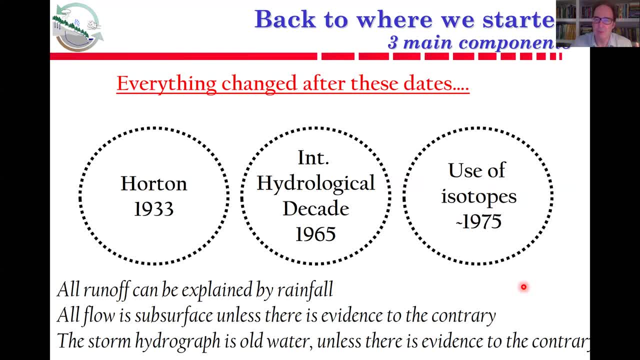 And, as you can see, it has really changed the way we think about runoff, because now it's all about the exfiltration, the effusion, the release of old water to the channel, and much of what we learned, what we thought about during the 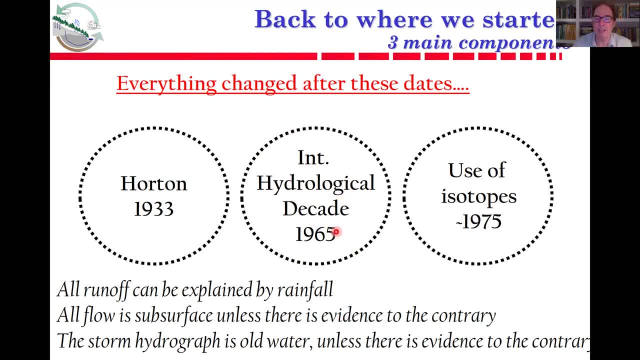 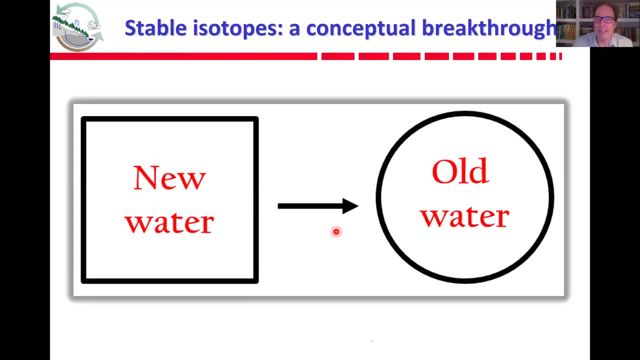 the first international hydrology. the first international hydrological decade was based on rainfall, runoff, hydrographs and wave translation and the celerity of the hydraulic potentials. Isotopes are showing something quite different, And what it's saying is that we've gone from a kind of a paradigm of rain. 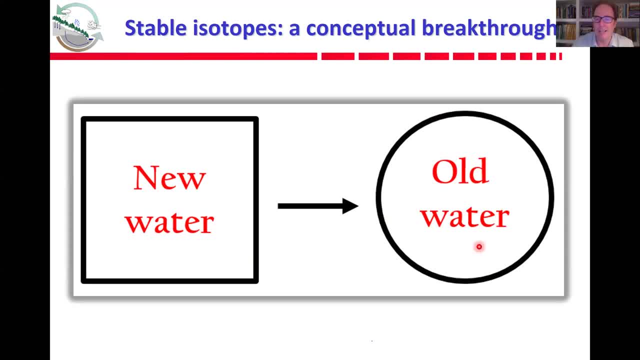 new water to a really a paradigm of old water, And you saw the, the, the, the new review paper by Giusecco and reviews of geophysics, really showing that for several hundreds of papers, The big question still- and this is what we're going to talk about next class is, for many places, 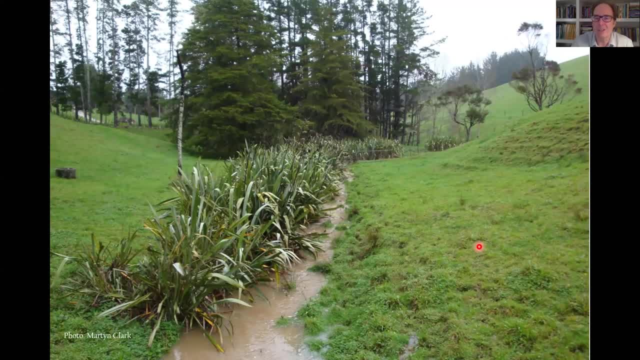 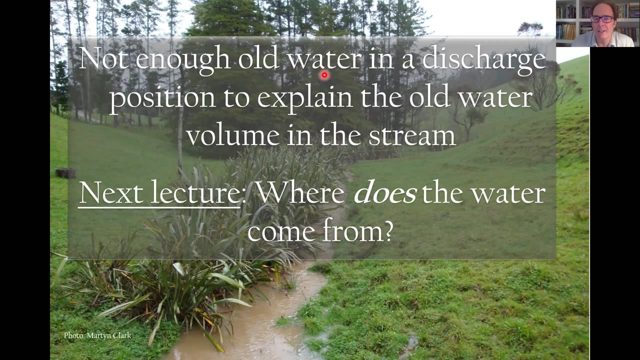 that aren't flat like you saw in Canada or Sweden, and they have some topography. The big question is, where does the old water come from? Because there's often not enough old water In a discharge position, meaning near the stream channel. 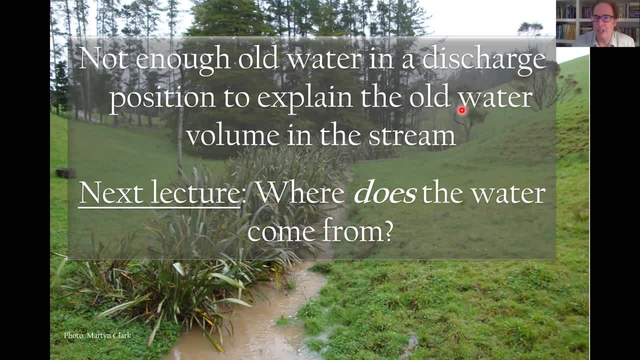 To explain the volume of old water in the stream. So the next lecture is going to get into more modern concepts of rainfall runoff And bringing in also the isotopes And understanding the role of Hill slopes in this whole, in this whole process. 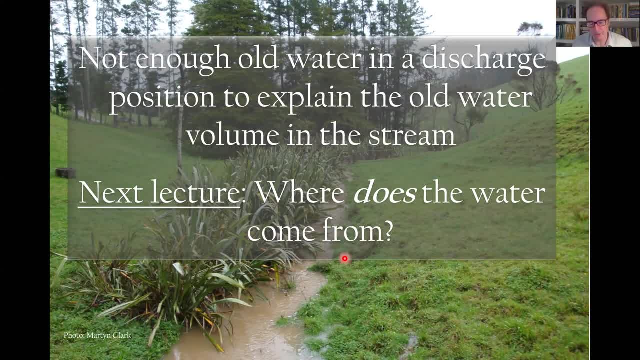 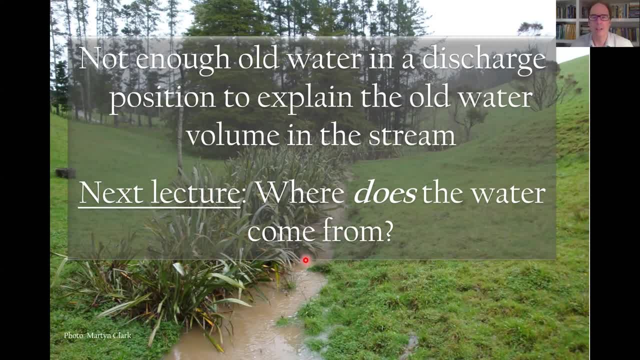 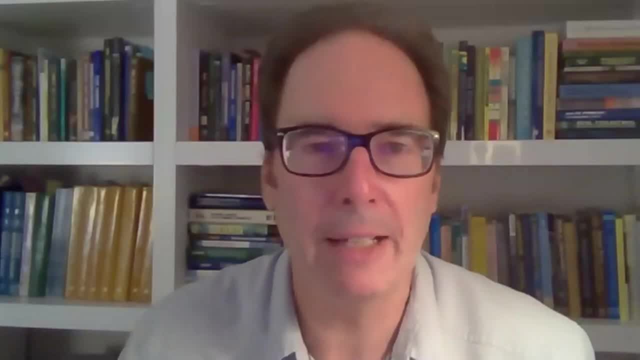 That's. that's pretty much where I wanted to get to. Yeah, Open it up for For questions. I'll stop If you stop sharing my screen, But I can come back to the screen if need be and See if anyone has questions. I'll open the chat. 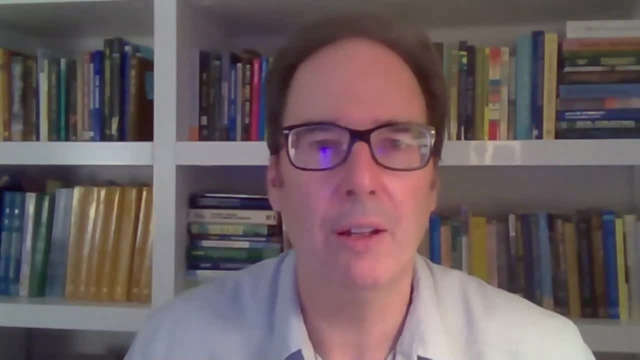 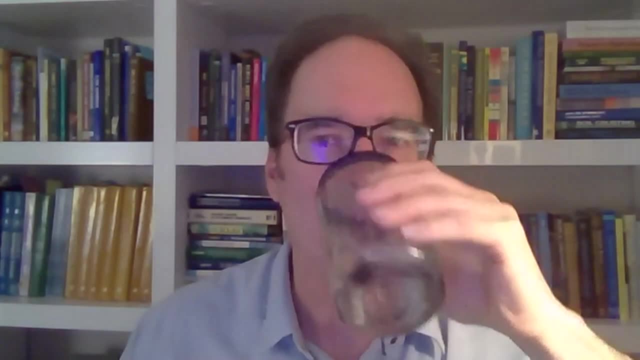 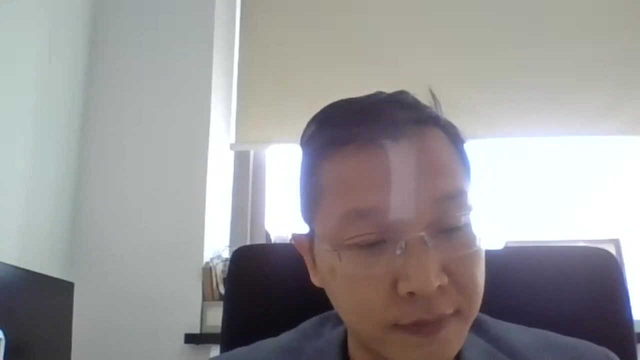 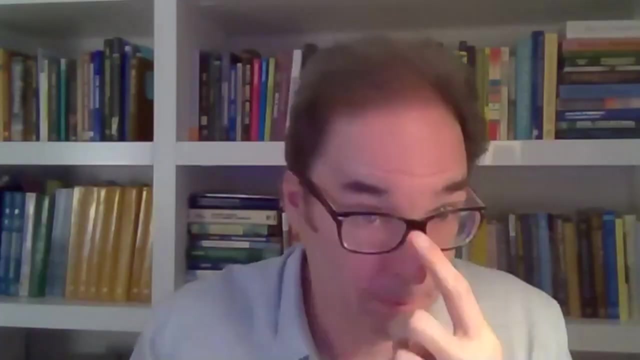 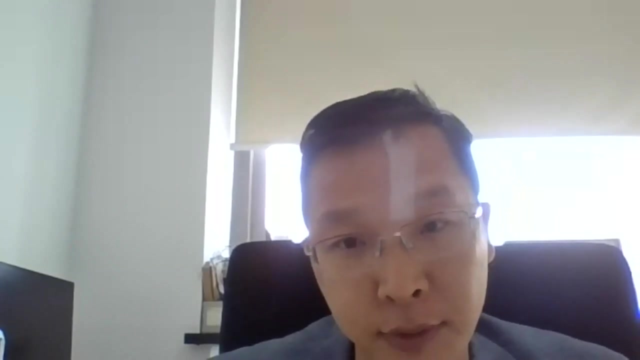 But you can question. so time for questions. yeah, any questions, jeff? yeah, yeah, i have a question just about your: the separation from the old water and the stream. yeah, you mentioned the heavy oxygen and, like this, mainly related to the evaporation. yeah, there's a constant, because in the 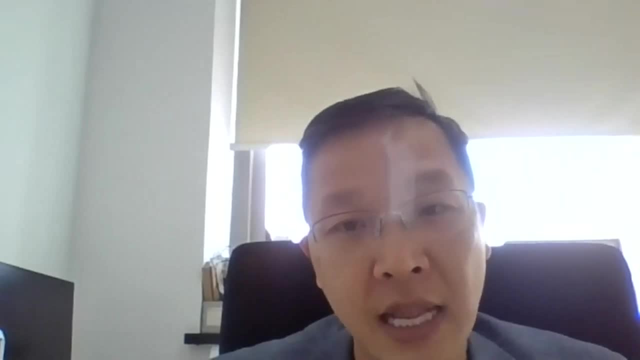 nest potato. uh, you know, the soil layer is very deep. the different layers, maybe the soil, the soil, water, the oxygen, like heavy oxygen, the constant contact is, maybe it's different from the layers to layers. so can we- yeah, can we- do some research on the different layers? and from the 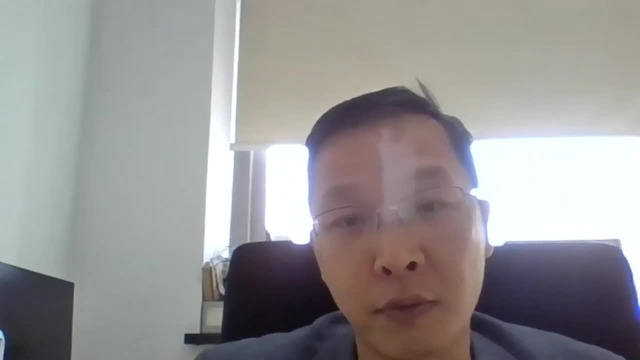 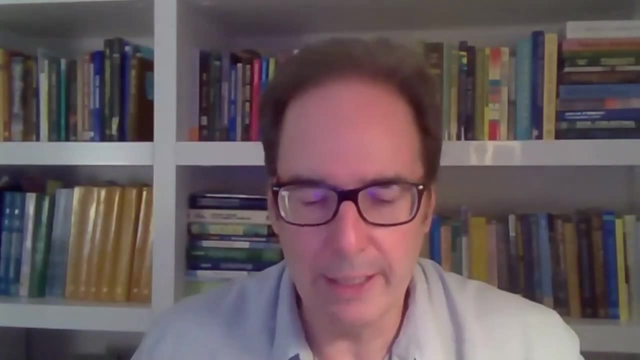 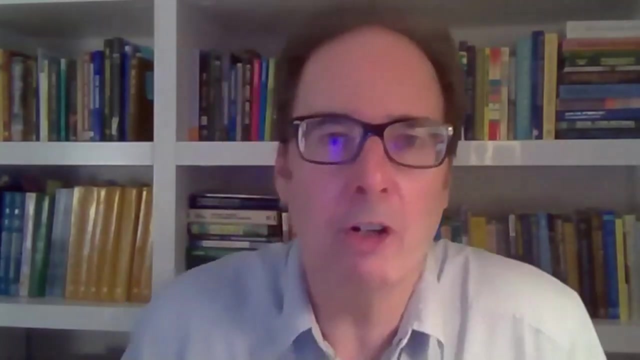 precipitation, soil water, different soil water and right there, the groundwater. yeah, yeah, yeah, you're right that uh in in uh less humid areas and in areas like the loose plateau, with very, very, very, very deep soils, the soil signature may look quite different to groundwater. that was remember. that was one of the 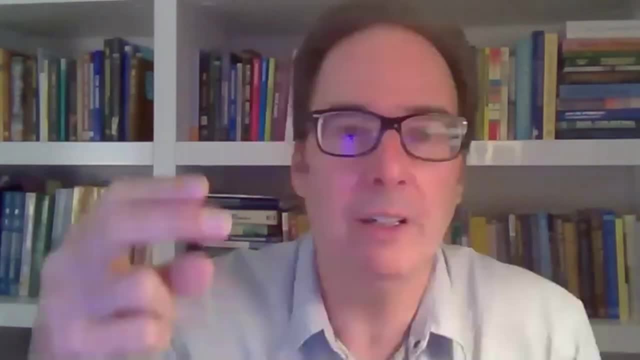 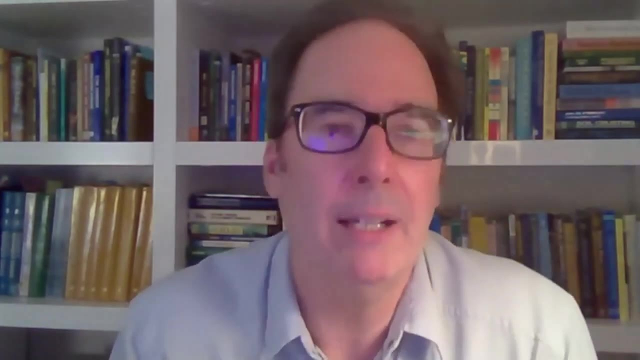 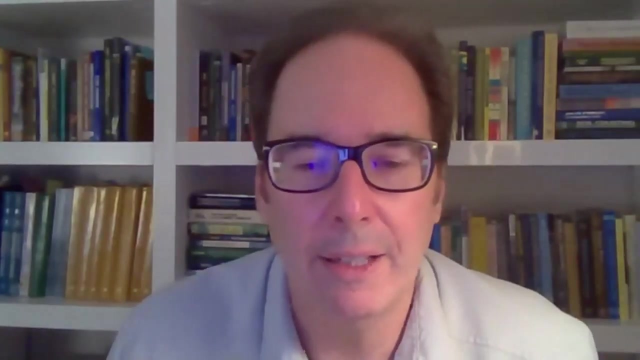 assumptions in the in the sklash and farvolden, five assumptions for hydrograph separation: yeah, one one assumption is that they have to be the same, but in some cases, like you're describing, it's uh, it's probably not the same, and this is both the problem and uh. 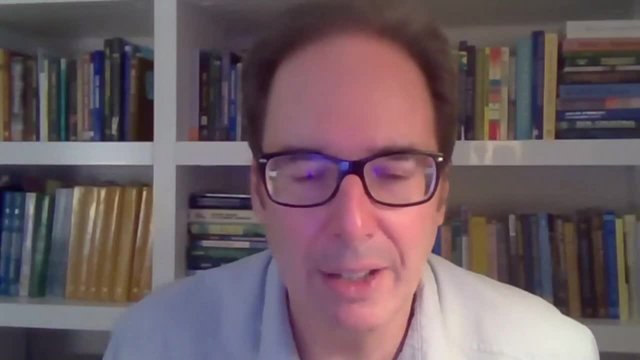 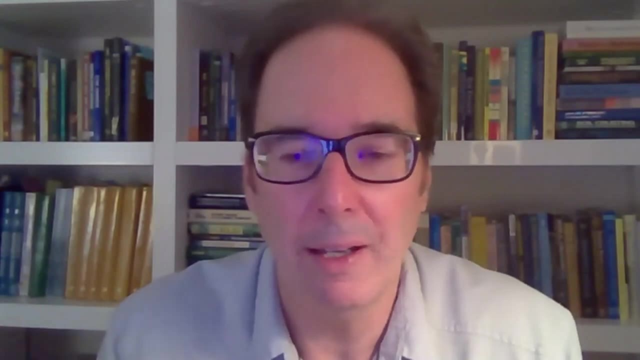 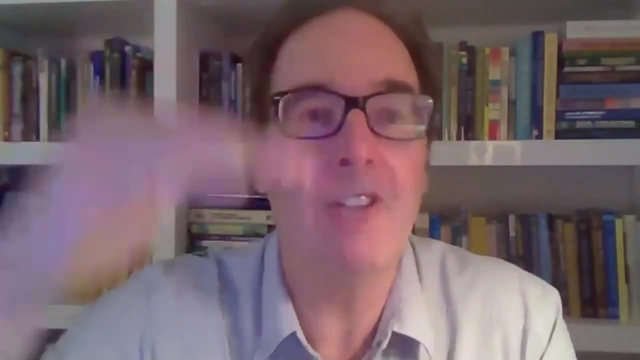 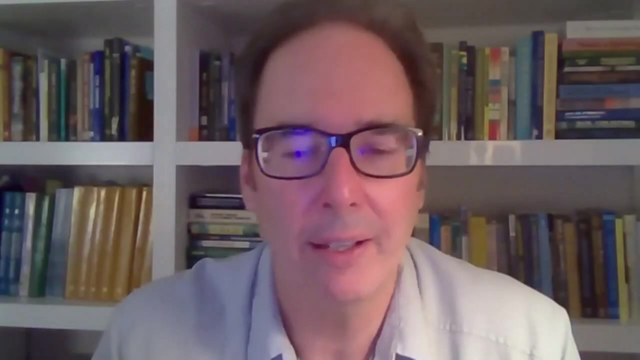 possibly a useful uh thing, because you probably have evaporative enrichment of the soil water associated with uh- a bare soil evaporation, but also diffusion in this very, very deep unsaturated zone. yeah, so you would probably have fractionated looking soil samples and we're going to look at some of these. 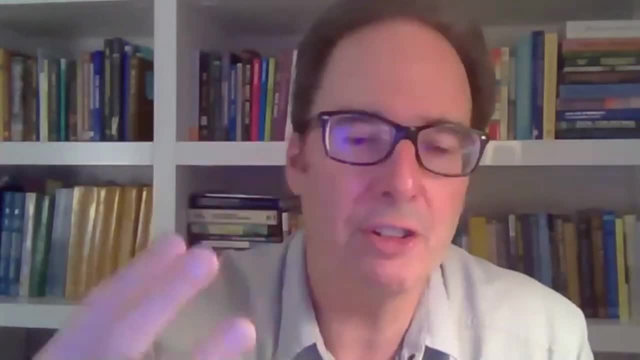 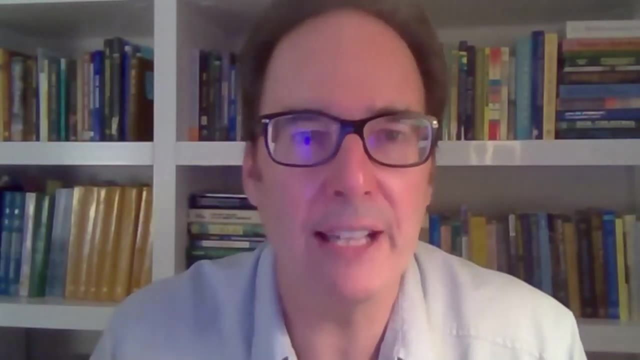 examples on lecture four, that starts to think about what happens when you get changes in the soil water signature and how can we trace that into streams and into plants and understanding the eco-hydrology of hill slopes a bit better. but you're right, you, i think you would. 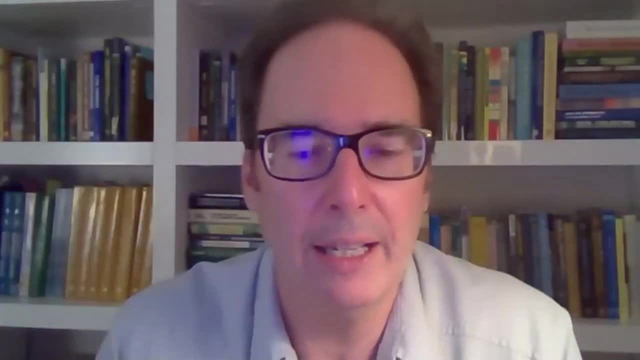 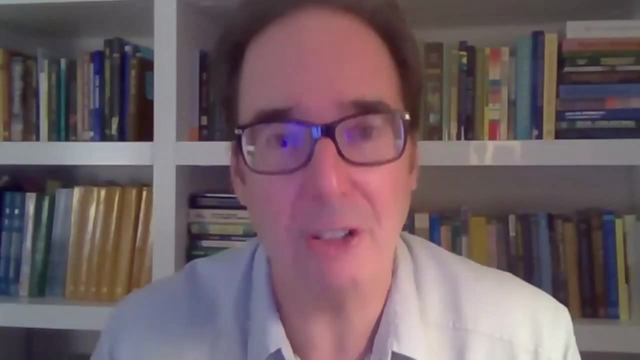 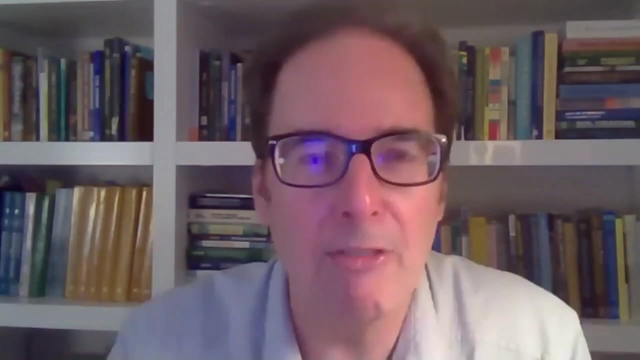 see what you're describing on the loose plateau and it may be it may make things a little difficult for hydrograph separation in the traditional sense, but but it probably creates many opportunities for research and i'll try to make reference to that in the lecture number four. yeah, just as you, you mentioned the 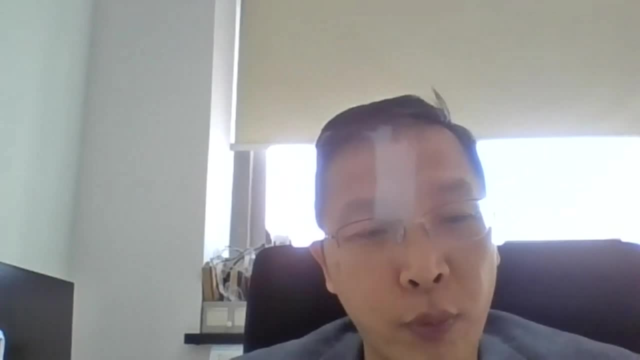 because as uh as we, because, due to my knowledge, the most of the precipitation, the infill, infiltration soil layer is almost uh, one or two millimeter, two meter, two meters in the last plateau. so maybe the plant, the soil, the just uh, from the zero to two, just about uh the up. 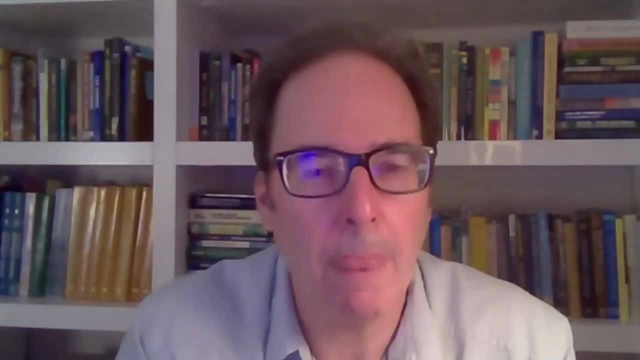 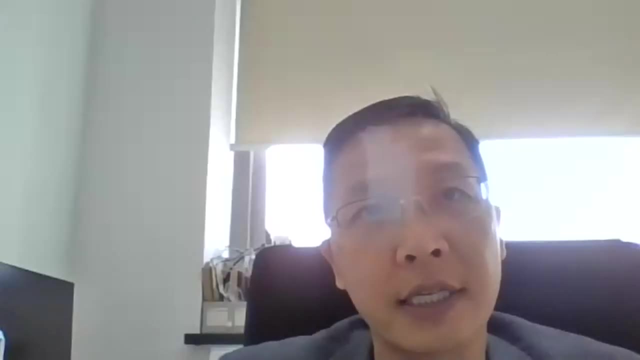 two meters soil layers is very important for the, for the plant growth. yeah, yeah, so maybe the different, especially for the ups up soil layers, you're very uh different. uh, uh, so uh, oxygen, like as heavy oxygen, the constant, because because of the uh plant, plant growth and the soil, the infiltration and the 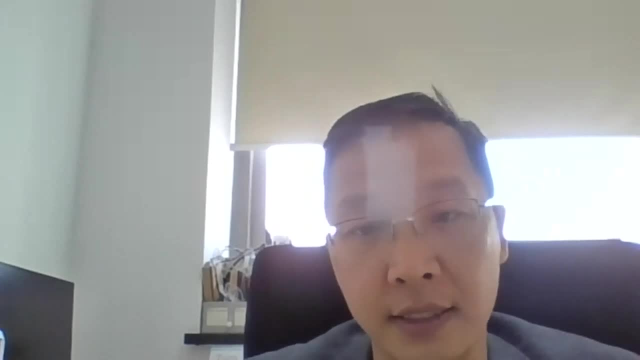 some of this soil, uh, physics like this, so maybe it's com complete complicated for the soil make soil water, how to uh move, how to move from the from the upslope to the downslope, from the opposite layer to to the, the deep layer. yeah, yeah, i think. 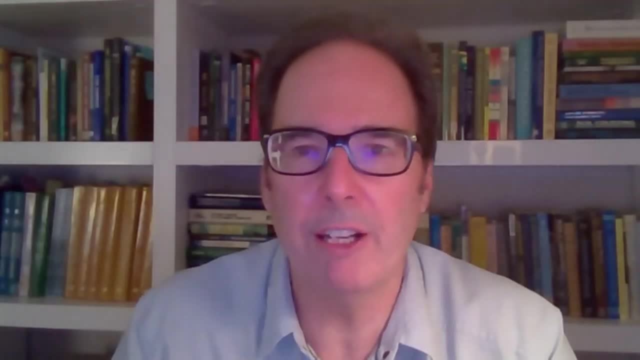 you're right, let me, let me just let me just try and find a slide real quick, if i can. uh, if, since we're on this topic of the loose plateau, um, hopefully i can pull it up. uh, you can't see my screen right, or can you? 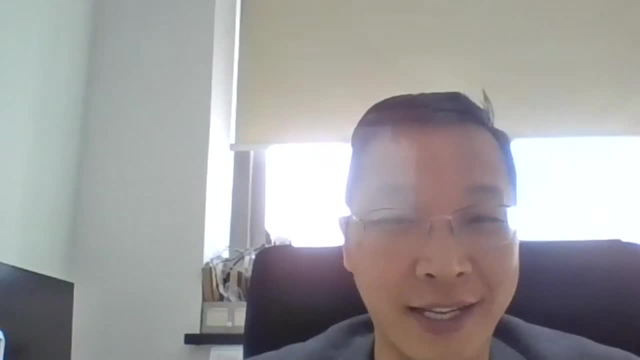 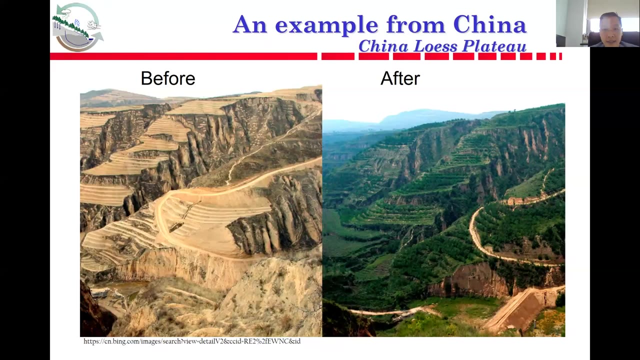 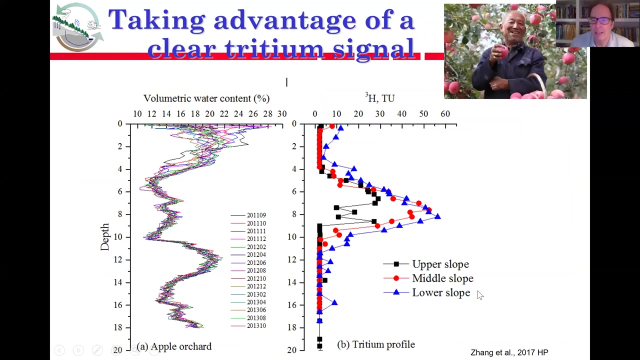 no, yeah, i cannot see it here. okay, do you see it now? yeah, yeah, yeah, okay. so here we are on the list plateau and, uh, this is. i don't know if you've seen these data before, but this is a paper. it came out, uh, in 2017. okay. 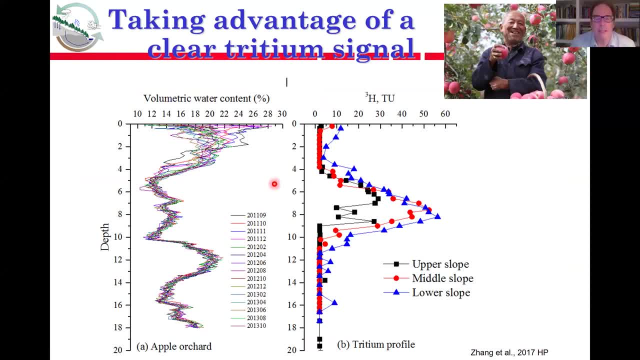 and i'll just get my laser pointer. so here's uh depth. this is work led by the group in in at northwest ag and forestry university: um um li ju and bing si and some of their students. this- yeah, this was a phd student zhang, so here's uh. 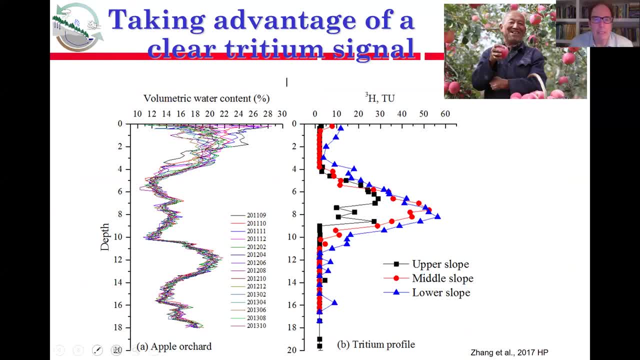 the soil surface here and this is a 20 meter deep. 20 meter deep profile. they've dug, yeah, and they they looked at the volumetric water content, actually taking soil samples and and uh, making measurements with with depth, i think they'll put td or um. 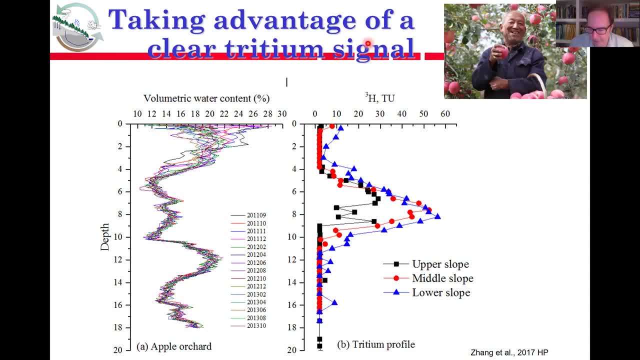 no, they also had, um, uh, yeah, you know, uh, measurements of uh- a oyster, i'm forgetting the technique right now- um neutron probe measurements down through the profile. and now, look here, this is the, not the 1h or 2h, this is 3h, this is the tritium, this is the radioactive isotope, uh. 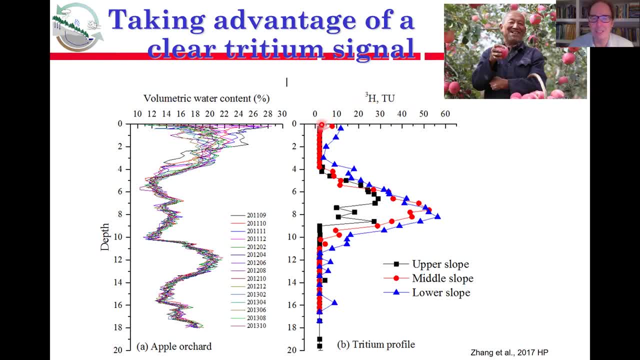 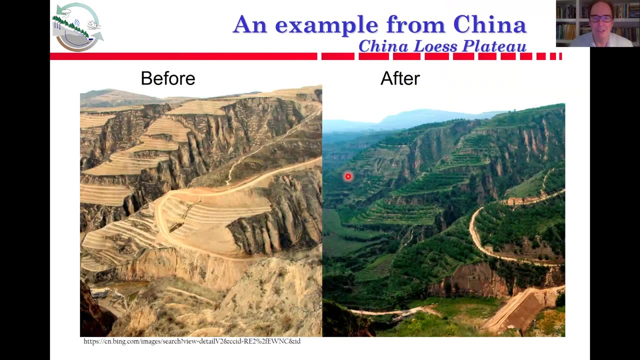 h3. what's really beautiful here is that this is the bomb tritium signal preserved in the soil in these very deep, deep units. so remember that I don't know bomb tritium look like this. this is 1962 or three. this was the peak of the bomb. 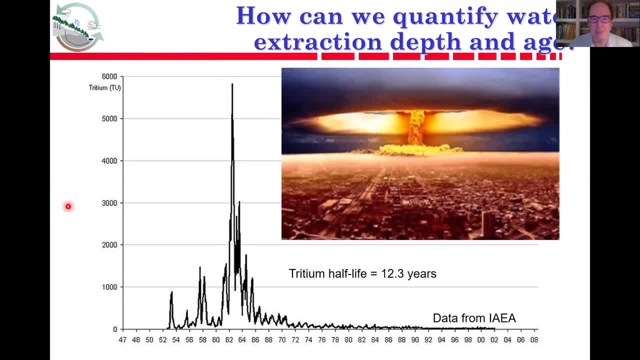 tritium signal globally on the y-axis is tritium units in precipitation and we had the comprehensive test test ban treaty globally, and then the world's tritium started to decline. but look at the shape of this curve. see the shape of this curve. you like that? and now look at the shape. okay, this curve, there's 1963. 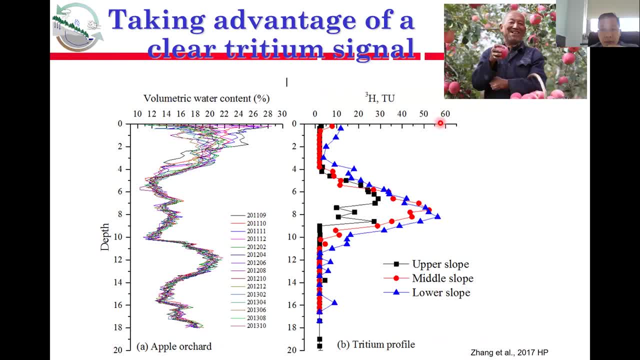 right there. yeah, so it's taken from 1963 until 2017 to go eight meters below 2.1, and chin state التي gran society n. but you can do this to amazing is that they plant apple trees on this area and the apple trees send down roots all the way to 12-13 meters. so what you can do 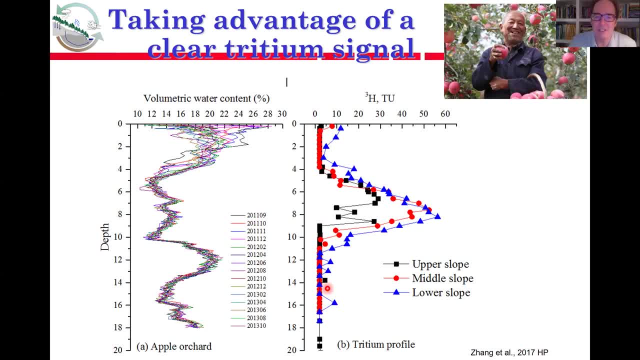 then is: pick the apple, calculate its tritium concentration and then, using a mixing model, say what the distribution of tritium was that the tree roots sampled from through this profile that has the tritium signal in it and- and I think this is something I can work with- 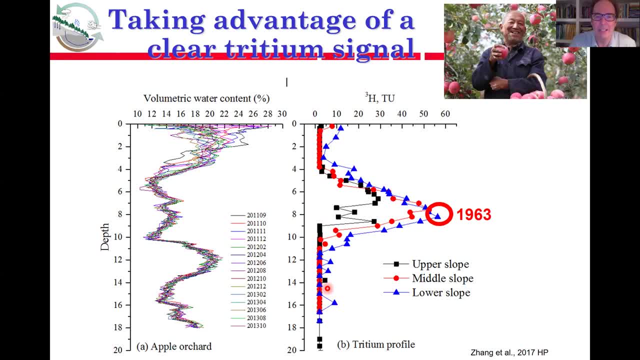 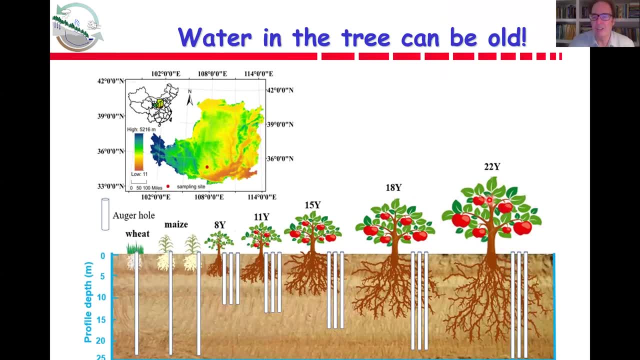 i'm really excited about, because what you can do then is, uh, you know, for different age trees, you can quantify the age of the apple water, and for these older trees that are sending roots down quite deep, 10, 15 meters, the apple water is on the order of 30 years old, and you get this with a kind 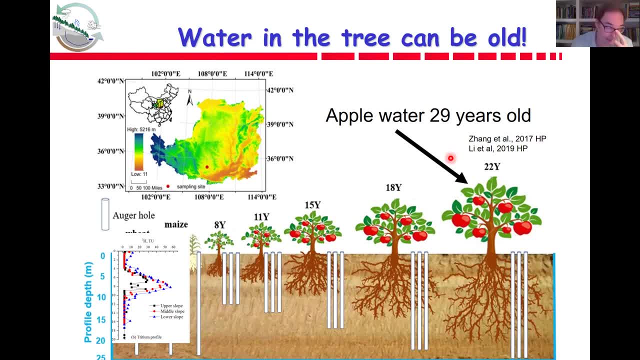 of a bayesian mixing model that the group at northwest ran. but there's, there's so much that can be done, i think. um, not just with the stable isotopes, but also the, the radioactive isotopes. that's very exciting, yeah, yeah, so excuse me, maybe you can turn to the last slide. yeah. 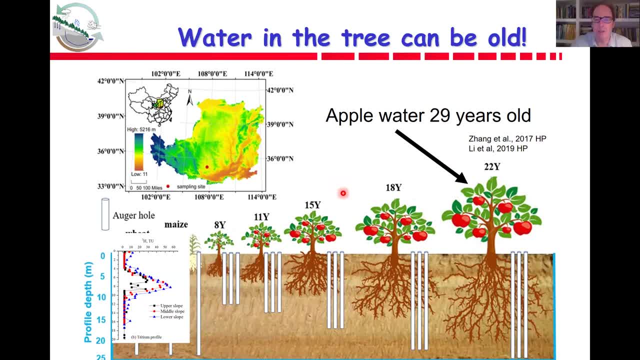 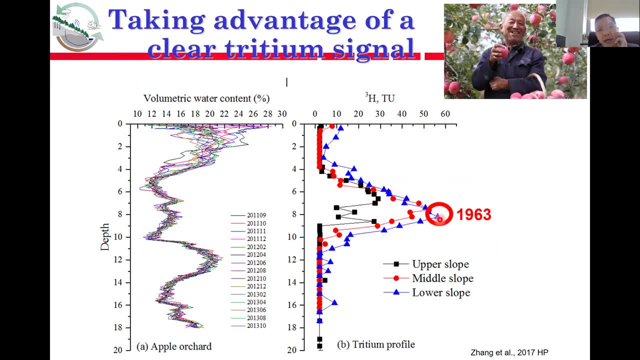 this one last time, just uh, yeah, this one, just so. you mean, the 19, 1966, we got the, the peak, the, peak, peak value. yeah, yeah, this, yeah, when did you do the? just uh, mayor, the, the, the, the, what, the, what's come? uh, this, this value? you mean, these are the trend 2011 or 2000? yeah, maybe, i think it was. 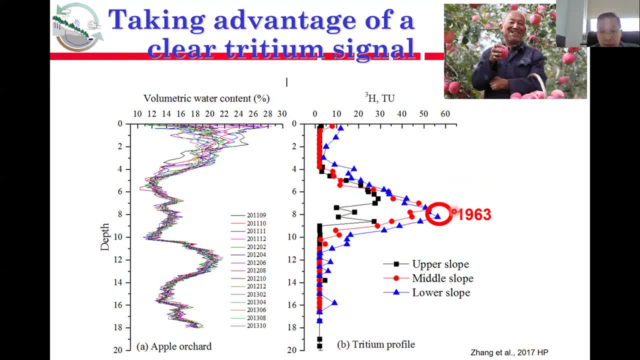 measured in 2016.. of course, this is radioactive, so it has a half-life of about 12 years, so we're we have to take the half-life into account. so these these values here are are greatly diminished in terms of tritium units. look, it's 50 or 60 compared to 6 000 or 5 000, right? so 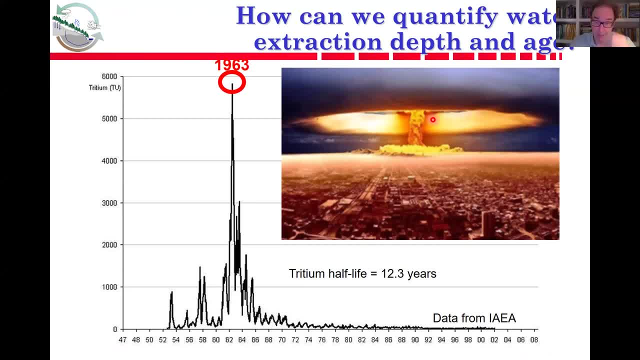 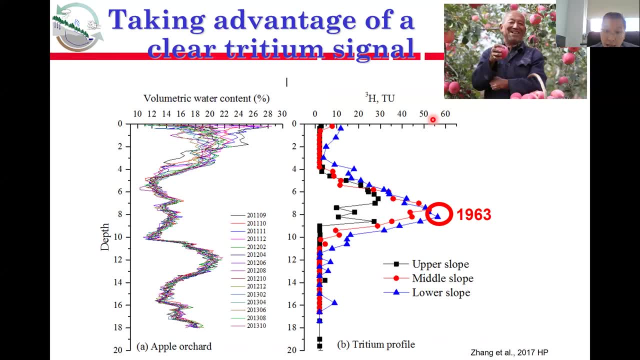 we have. we have radioactive decay as well as mixing to contend with. okay, so just it means that we the the soil. this is the eight millimeters the soil as a soil water maybe come from the uh, maybe the 50 years- yeah, took 50 years to for the uh, for the. 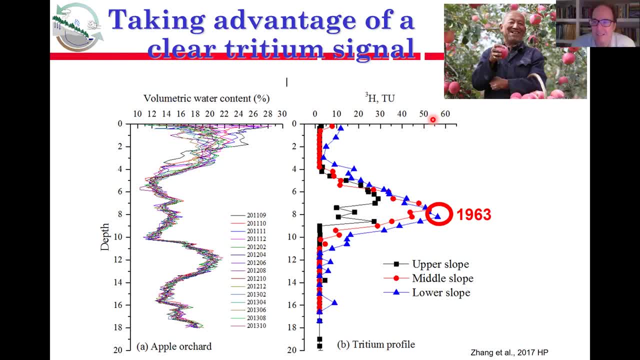 precipitation, yeah, yeah, yeah, can, can infill, infiltrate the deep soil layers in the apple, in the apple, ultra, yeah, well, yeah, so think of, uh, the differences between soil water movement and groundwater recharge, which could also groundwater recharge, could be affected by preferential flow processes. so this 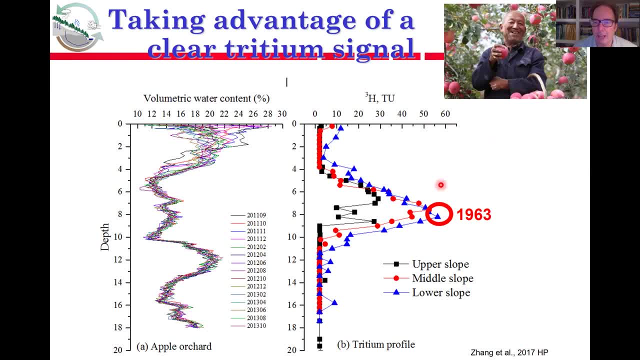 is the- uh, this is kind of the the poor velocity, if you like- of the small pores. there could still be cracks or macropores that mean that some water could penetrate deeper over 50 years. so these are some of the, some of the different species that we're looking for. 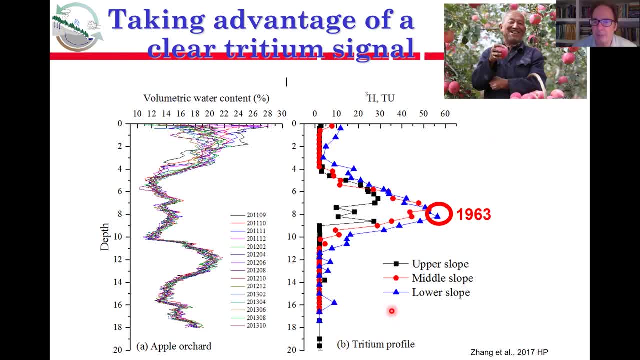 yeah, i'd like to take a look and i i agree with jim and his presentation. uh, i don't know, with many of the species that we're looking for, look, you know where do we have to look around during this: the, the, the trees that are. you know, it's, it's, it's, it's been there for a long. 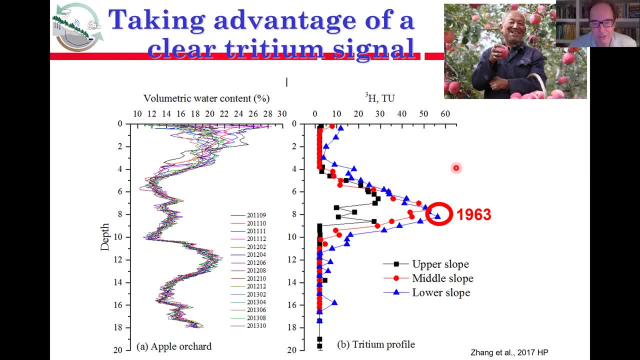 time, the trees and the the water that's being used by the trees, that are being used by the trees. the trees that they're using are. there are trees that grow from some of the surface areas of the ocean, or some of the surface areas of the ocean and the soil right, so that's a nice way to get into some of the 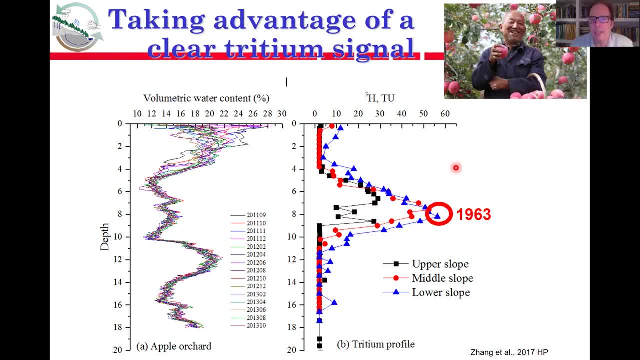 and many follow-on studies are now underway trying to understand this in greater resolution. Each of these samples are soil samples that were taken by augering, and then the sample was brought back to the lab for extraction and then analysis on a device that measures for tritium. 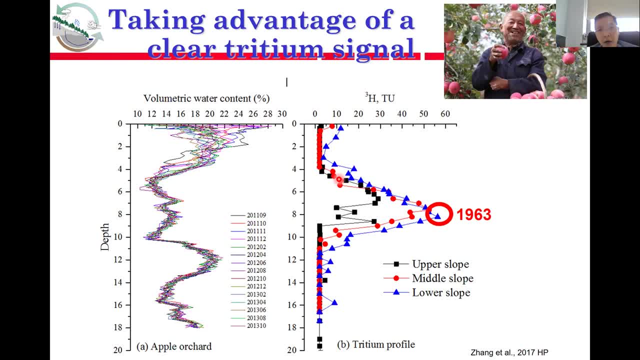 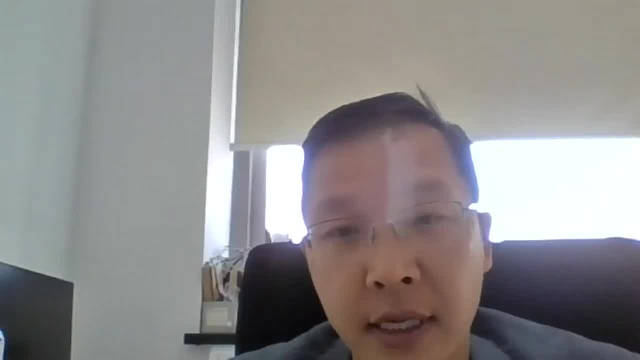 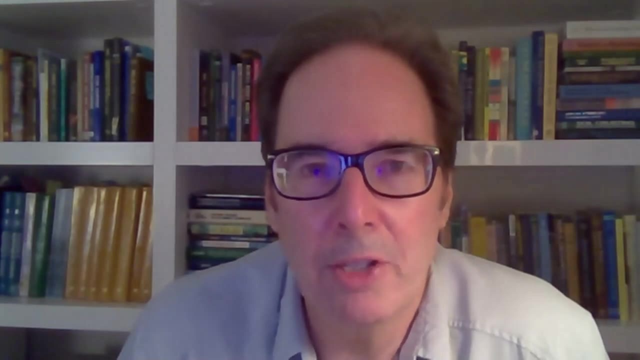 Yeah, maybe I think we can also do the, I think, for the natural forest. Maybe it's more meaningful for this. Yeah, yeah, that'd be very interesting. Yeah, yeah, yeah, Thank you, Sure, Any other questions or comments? Things that you didn't understand? 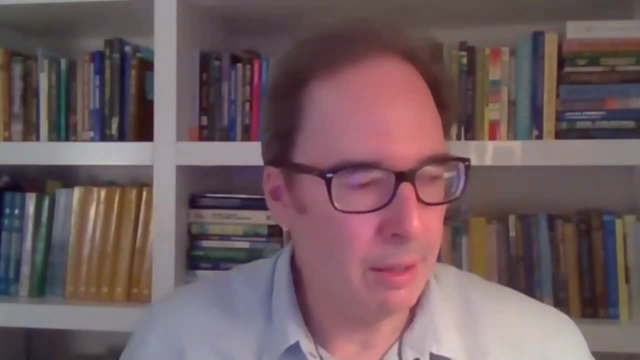 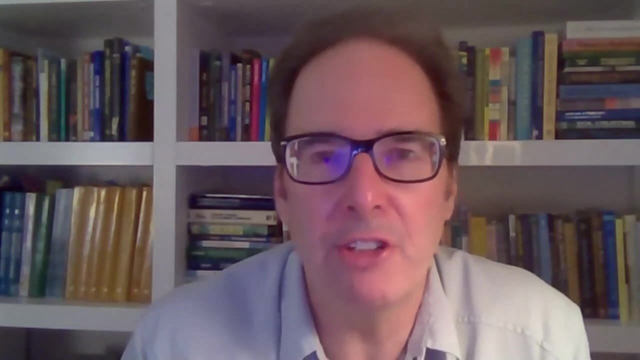 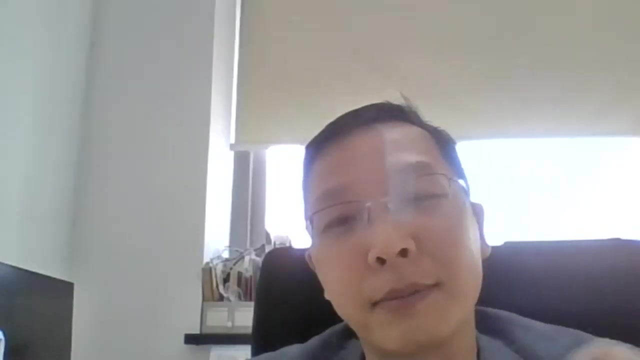 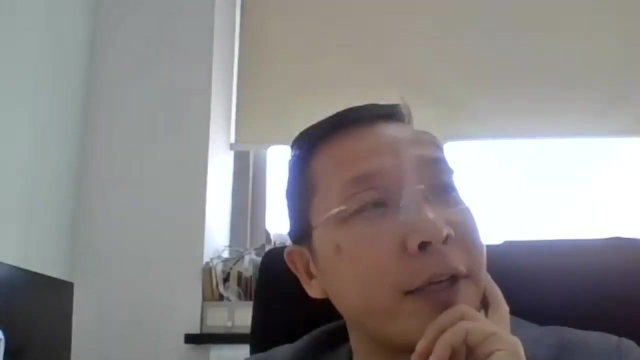 I'm wondering who? are you using isotopes at all in your work in Tibet, On your hill slopes, Tibet? I have not do some research on the Tibet areas yet. Yeah Yeah, Maybe in TMU some professors do some research on that. 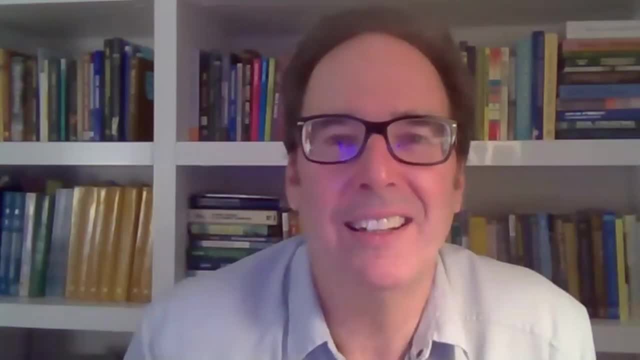 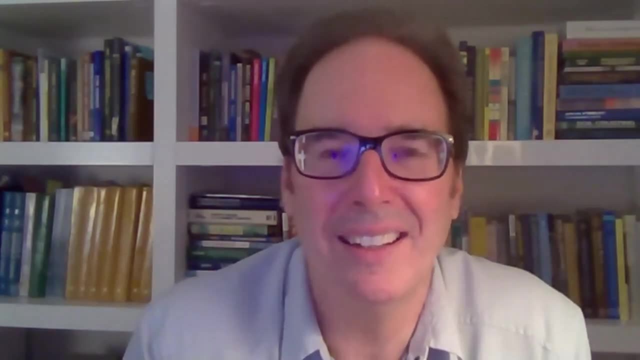 in the same samples. Yeah, maybe in BNU some professors do some research on the Tibet. Yeah, Maybe in BNU some professors do some research on the about. yeah, I was just looking at the Guangrong and I was wondering if he was doing any of that. 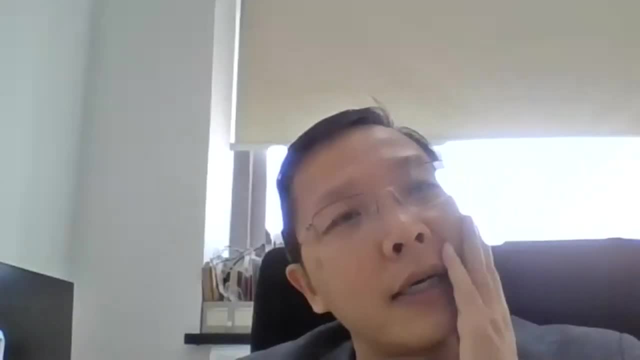 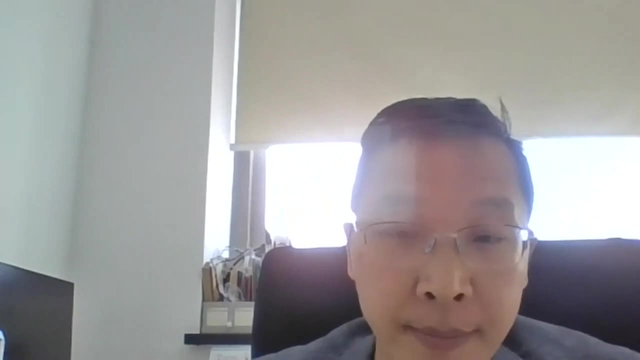 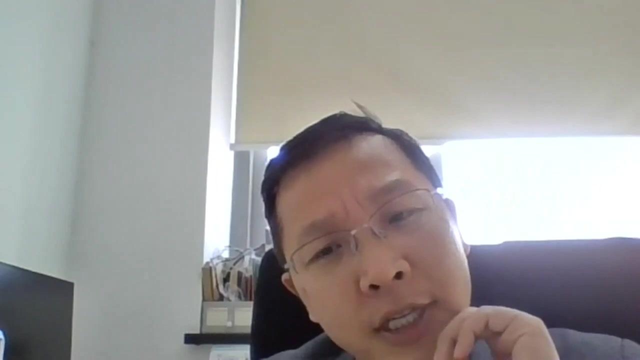 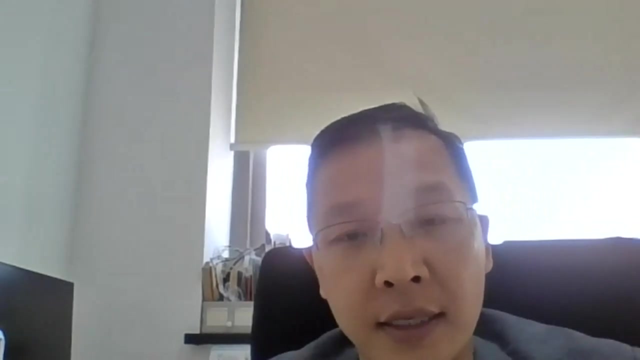 I have also a question on the. just a. you mentioned the. maybe a research paper mentioned the 70% old water dominated the stream, the storm, yes, storm stream. so in from my knowledge, maybe in the last China is very seldom the ground water in the. we cannot find the, the, the base water from the 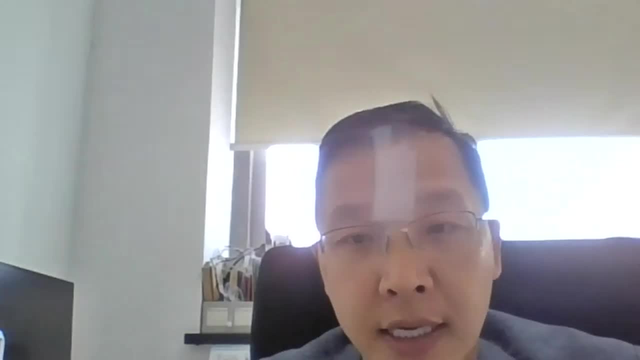 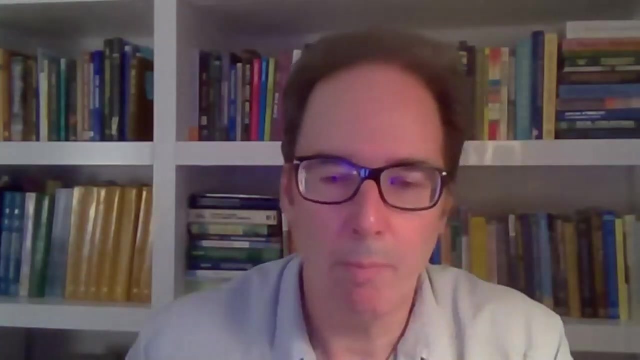 maybe in the middle scale was shed, so maybe this conclusion can. can you give us some suggestion on the lost on the North China in the area of me, middle area areas- do you agree the conclusion can be used in this areas? yeah, I don't know, I'm. 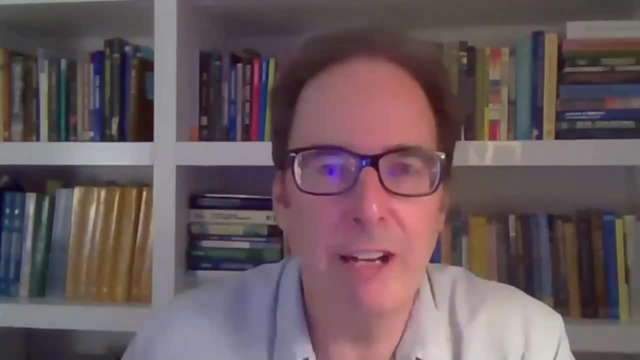 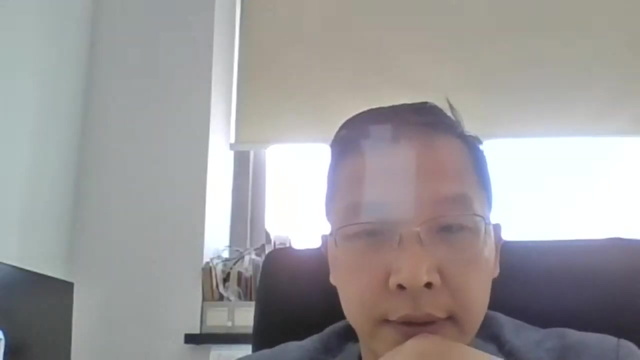 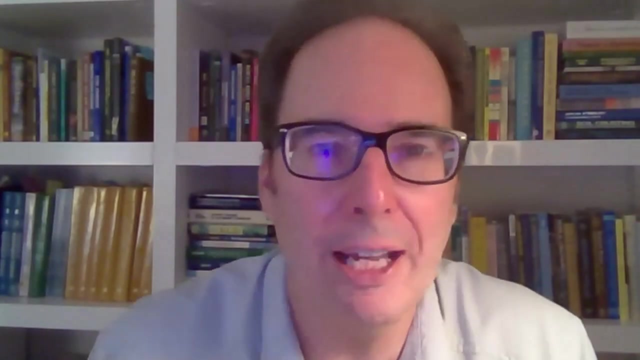 I mean again, it's going to vary depending on climate and hydrogeology. yeah, and as we'll see next class, maybe it's not true groundwater but it's soil water or it's water that was maybe perched water table on hill slopes that then makes its way laterally to the stream, so not. 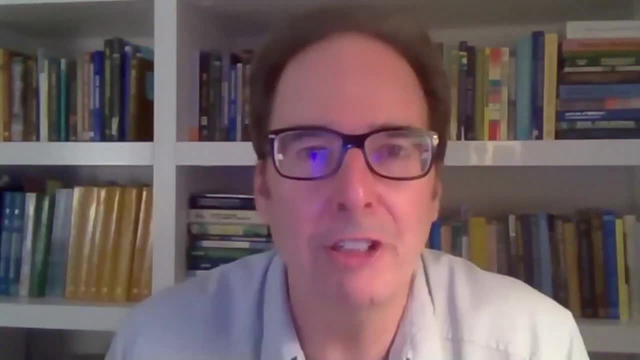 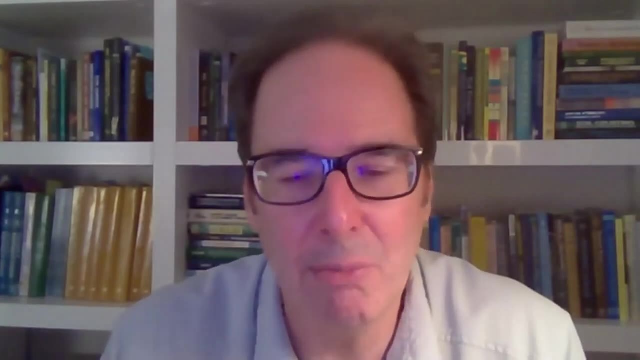 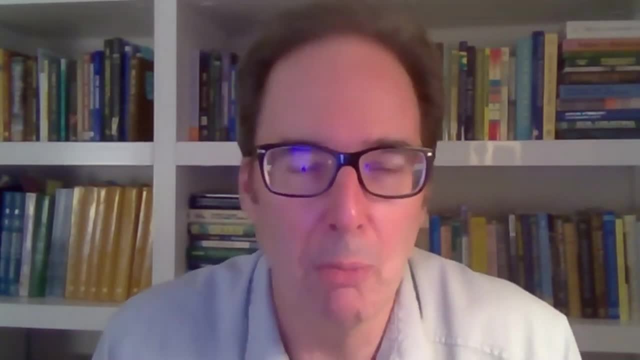 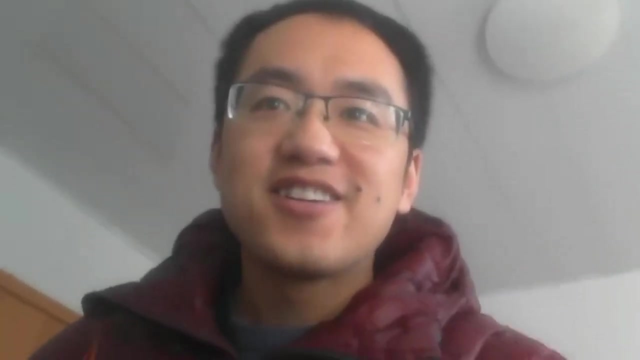 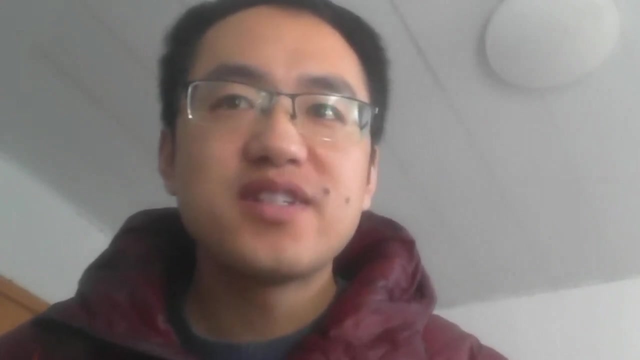 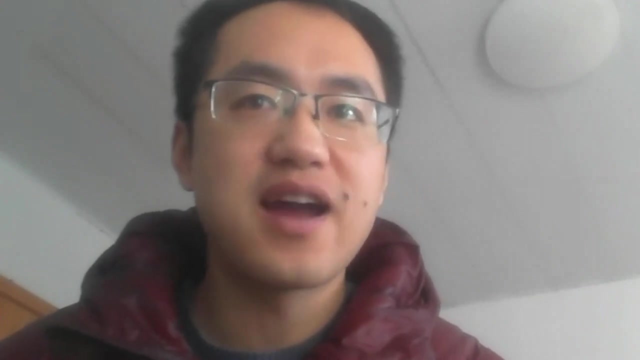 a little it. gastronomy in Ormowe if students. yeah, yeah, yeah, there is something wrong with my hair. so I have a question, sir. um, you think what is the key point that use cancer technology to help us to understand the subsurface flow passes, or health nope release and start a mixture process? your question is what? 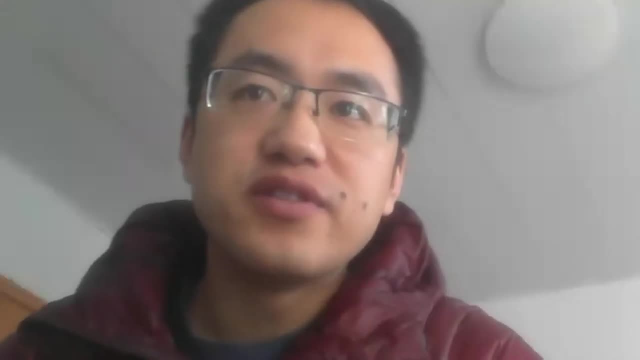 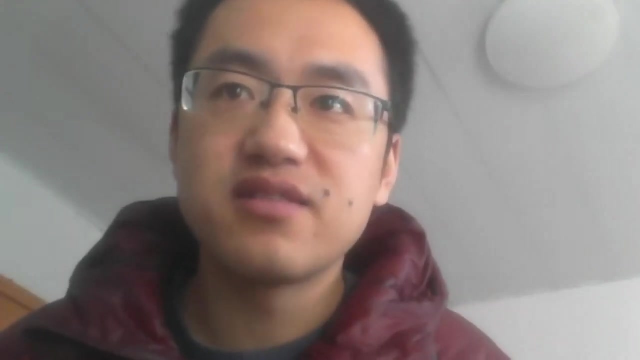 what's the key point? yeah, what is a key point- that's using transfer technology to help us better understand- is a subsurface flow passes, pass way. I'll help us to understand- as a health slope mixture, a release start and release process process. yeah, well, the key point for 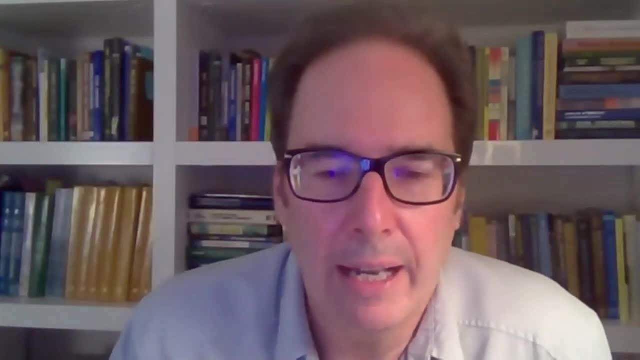 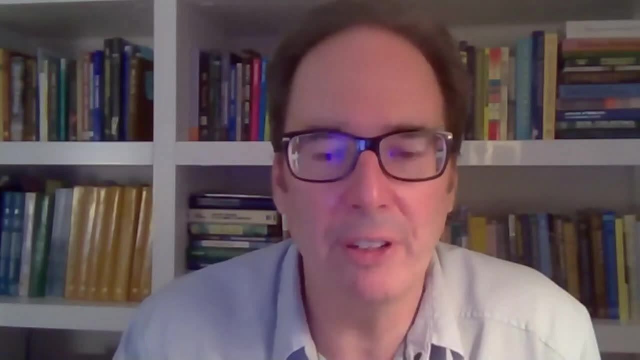 today's lecture is that after we started using stable isotopes, starting in 1975 and until the present, the whole thinking of hill-slope hydrology changed from one focused on rainfall or snow making to a subsurface flow process. and the key point for today's lecture is that after we started, 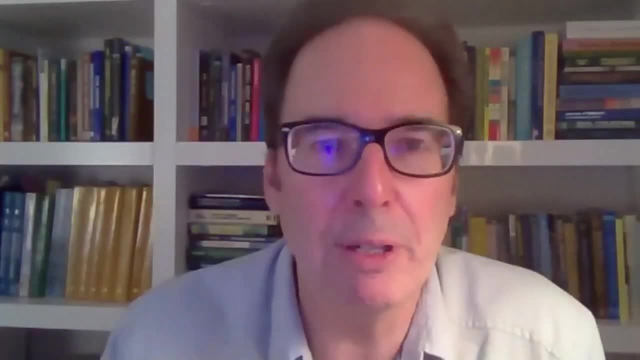 using stable isotopes. starting in 1975 and until the present, the whole thinking of hill-slope hydrology changed from one focused on rainfall or snow making to one focused on rainfall or snow making, to one focused on displacement of the water stored in the soil by that precipitation. so it 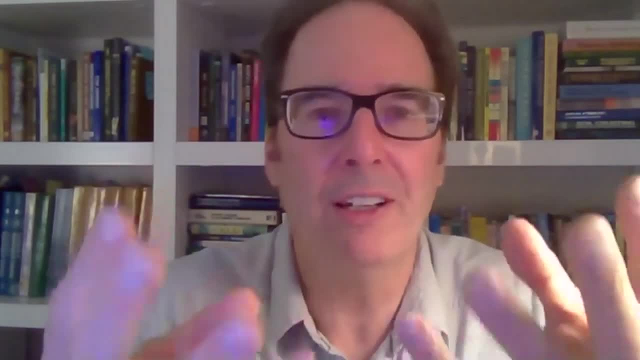 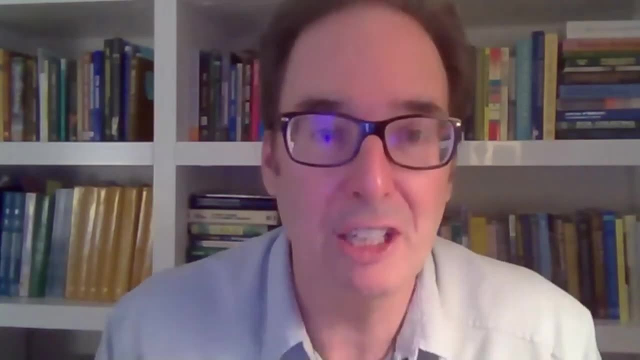 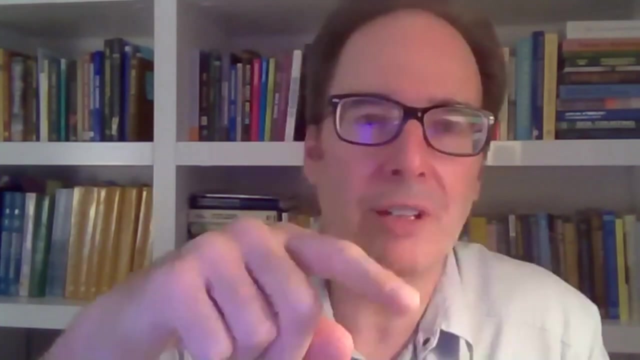 forced a recognition that there are these two different velocities- the celerity of the hydraulic potentials and the- and the velocity of the water molecule, and that they are radically different. so, even though the, the hydrograph is responding very quickly and sensitively to the flow of water. 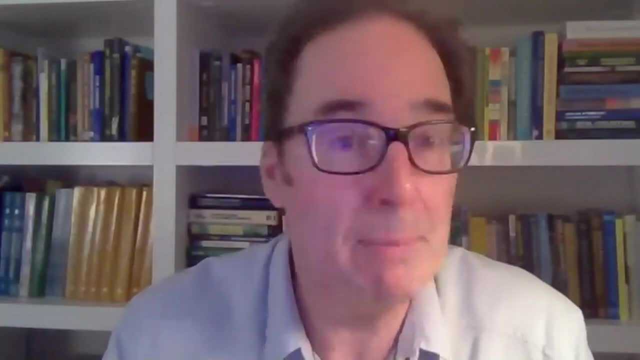 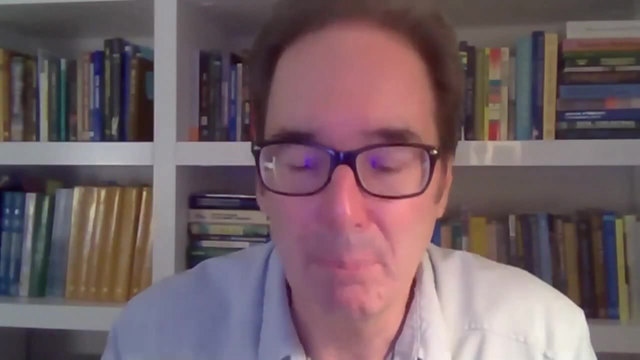 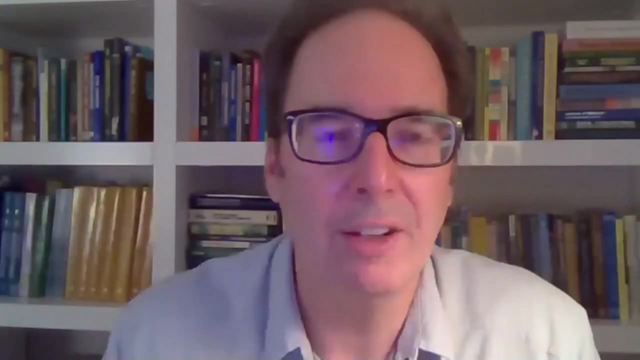 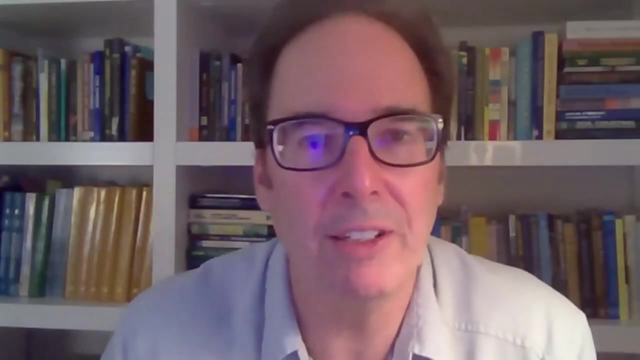 to say, a rainfall input, it may not be any rainfall in the stream when that happens. and that was a big change in thinking, because most of the work leading up to that was thinking that well, surely much of what's in the channel is the rainfall itself, or a large portion of it, so the rainfall is a trigger for. 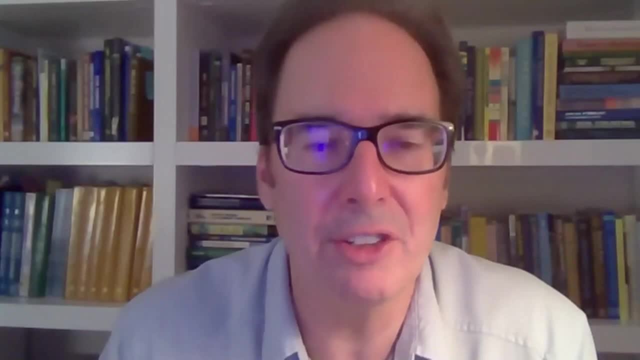 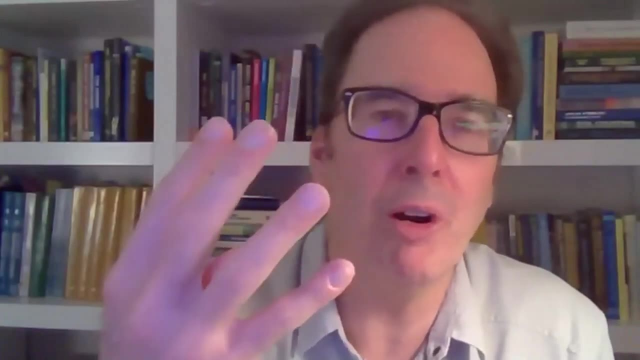 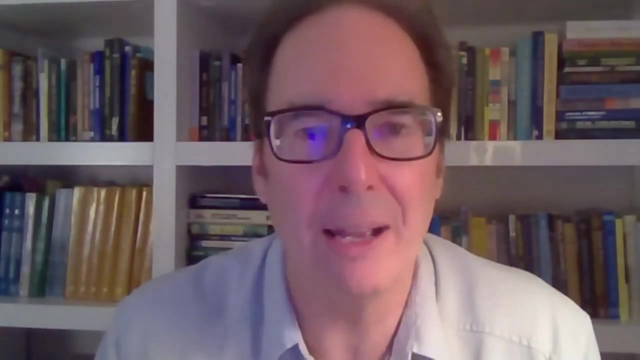 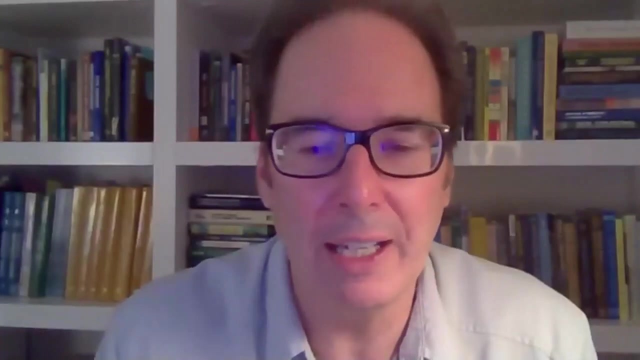 a release of water into the stream and understanding that blending is really the key. and, as we'll get in in lecture four, it lets us get at questions of the age of the water and the so-called transit time of water, and that transit time is so critical for understanding modern problems of, say, nitrate. 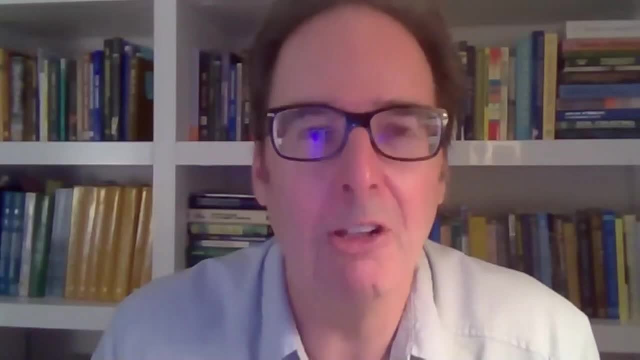 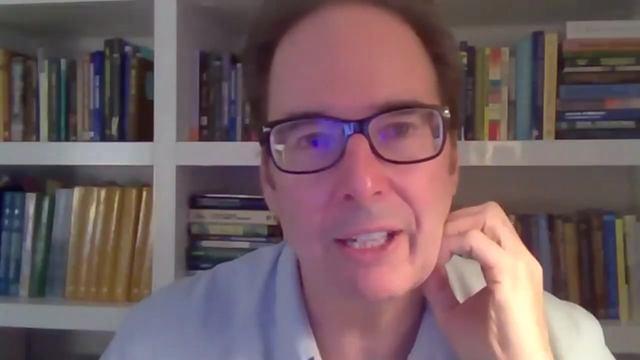 application to a hill slope and then how long that nitrate might take to show up in the stream you saw in the list plateau example. you know it took 50 years just to get eight meters. so in the list plateau they are adding nitrate at very, very high levels but we don't yet. 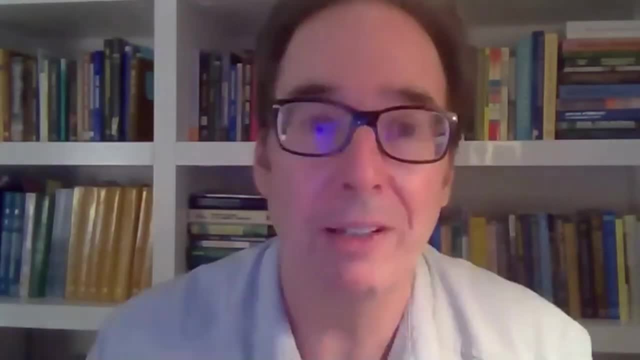 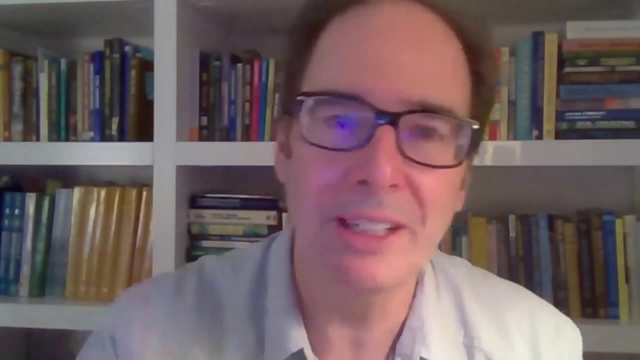 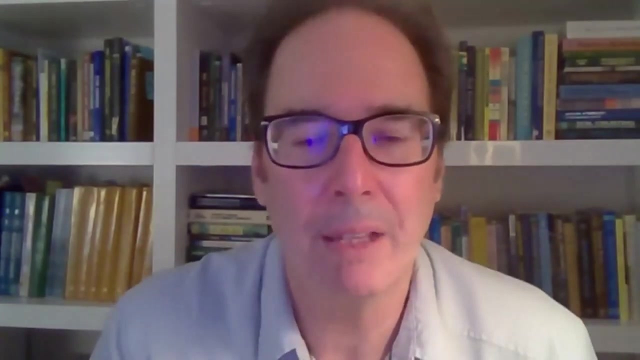 see it in the streams or the groundwater, but we will. so it's like it's a ticking time bomb, this problem, and but we can predict when we will see it, based on the transit time through the soil and into the groundwater. so that's what we'll learn. 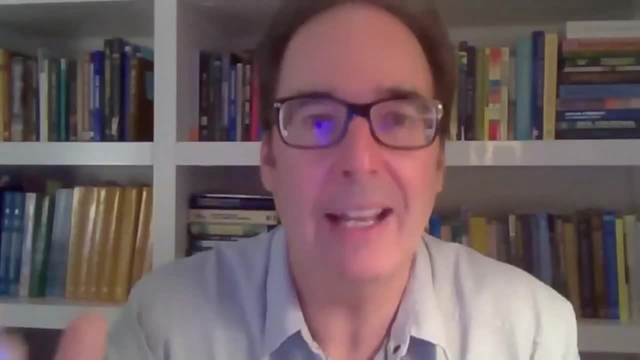 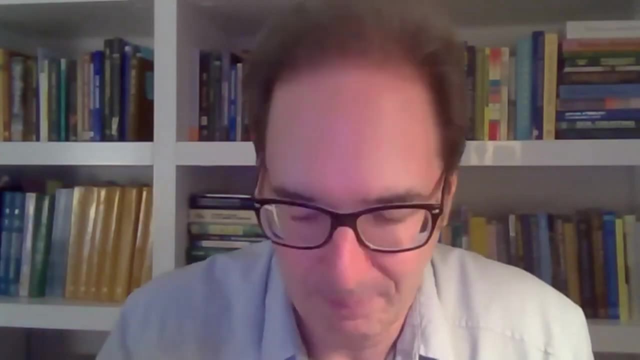 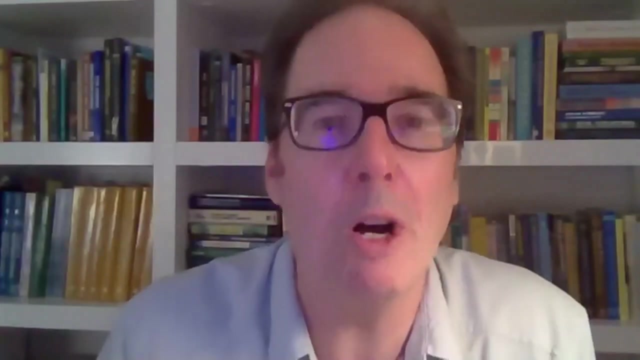 about in the next two lectures. how can we- yeah, now, use this recognition that, holy cow, things are very different and the isotopes help us to kind of follow the raindrops. now, what we? what can we do with that? what can we quantify? and transit time is a very useful thing that many groups around the 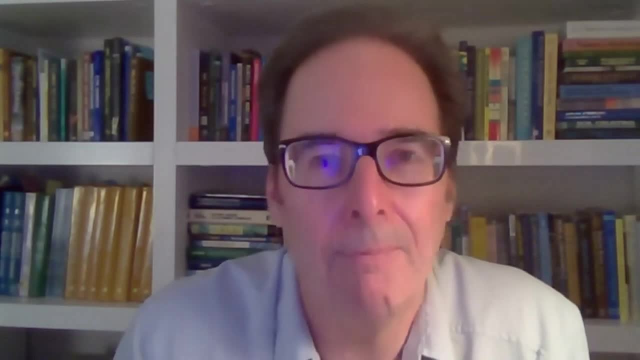 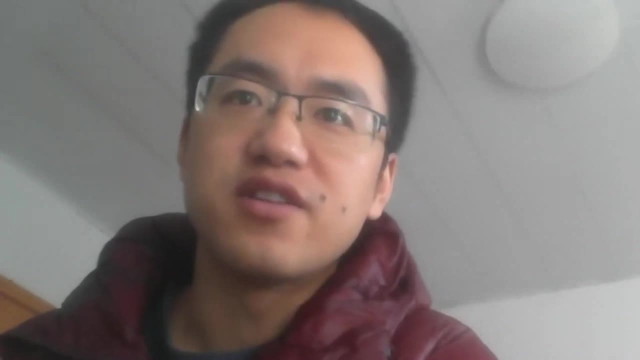 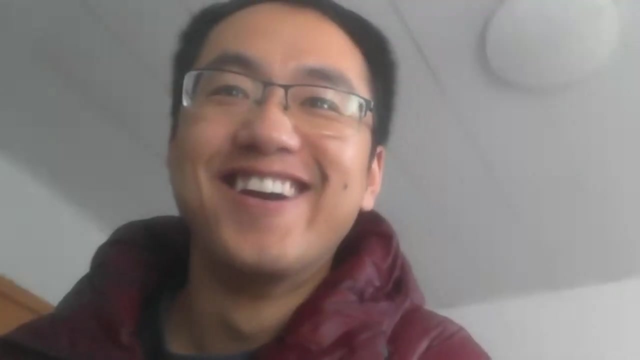 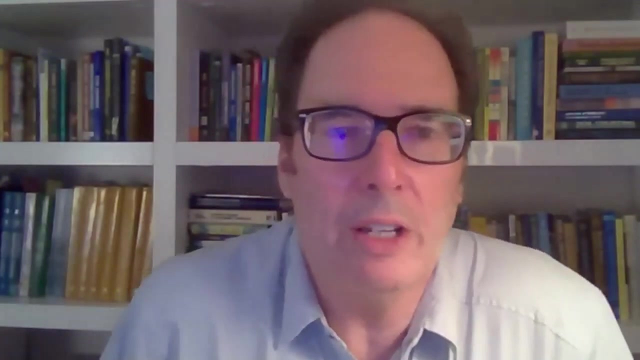 world are focused on now. yeah, yes, yes, thank you. I also do some research about the isotope transfer and geochemical chances. I collect high-frequency date and now has not finished. all right for your same hill slopes, yes, okay, and are you so what? do you still have to analyze them, or? or is what what is? what is what's holding? 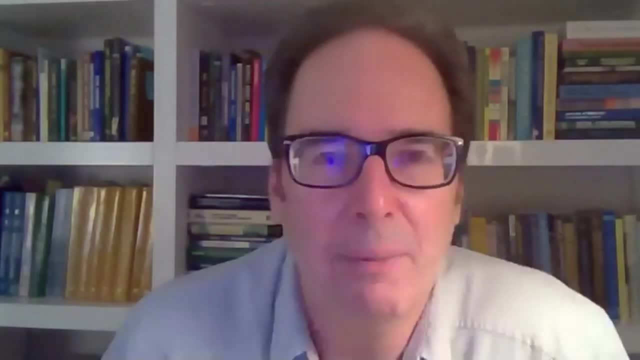 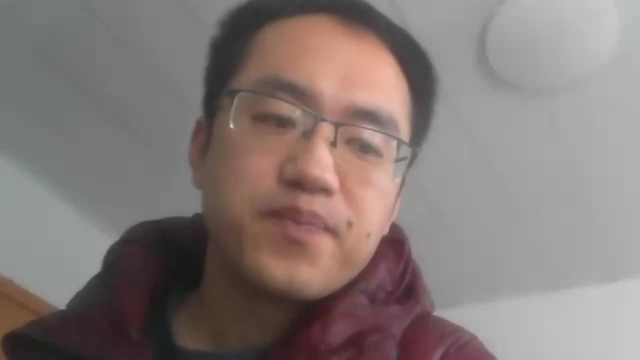 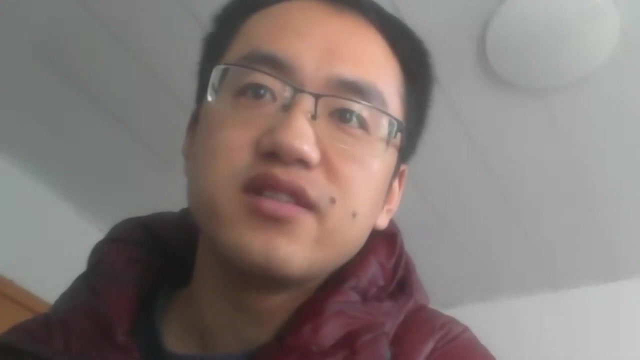 you back with that analysis, just the processing in the lab, or or analyzing the already analyzed samples? uh, last year I have, I have faith, I have finished is an nice Even that okay È, Because the data is not finished to- Uh-huh yeah. 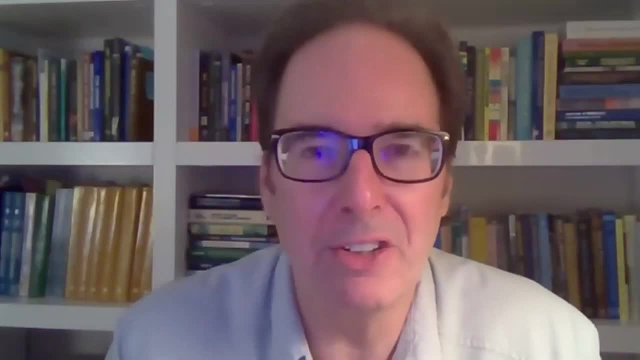 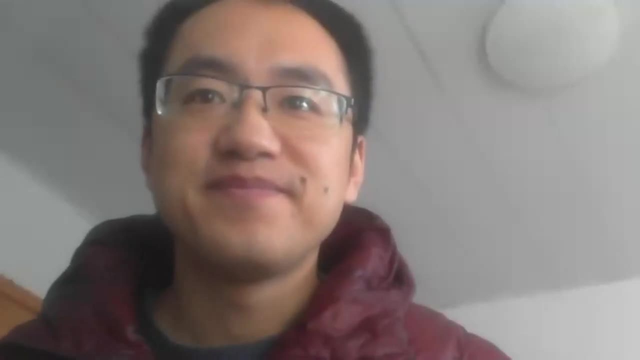 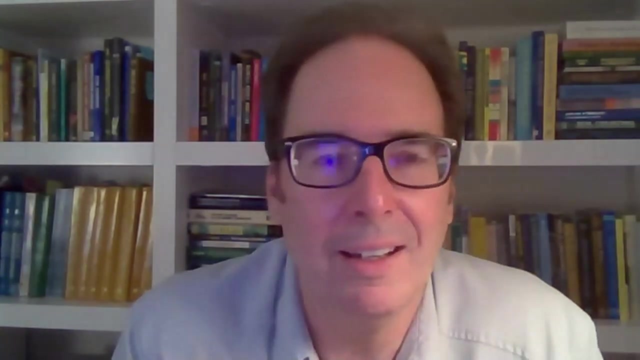 That's great that you have that information. Again, we can talk about that when we have a Zoom call, maybe in a couple of weeks. Okay, thank you, Jeff Yep. Other questions? Hi, Professor, Yeah, This is Mu Zi. 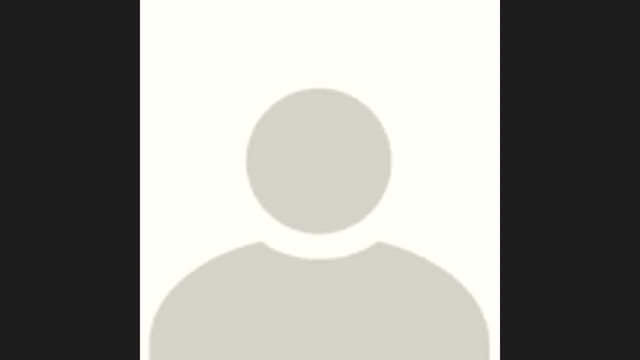 Hi, I have some. hi, I have some problem with my video, so you can't see me. Sorry for that, That's okay. that's okay, Yeah, I'm very interested and thank you so very much for your presentation. 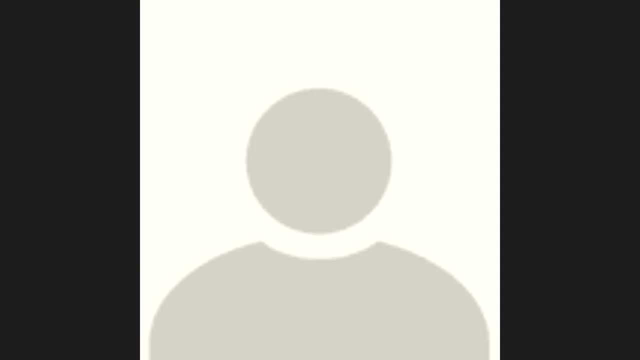 That's amazing. So my question? actually, I have two questions. The first is that: can we get a metaphor that it's like the Earth, the groundwater output to the Earth and the old water? it's just like the digest of the water in our body. 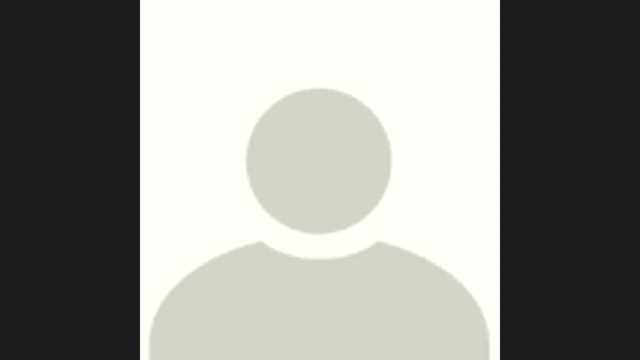 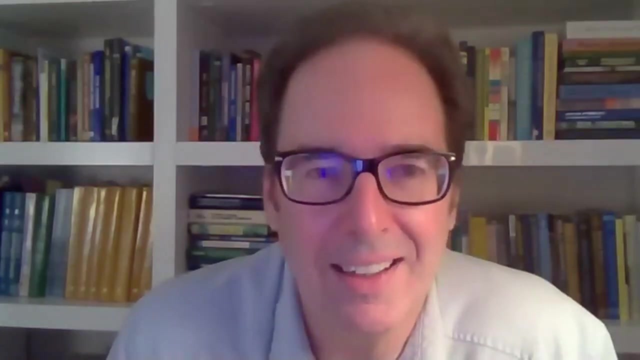 that our blood is always output the old water. Yeah, yeah, When we digest several days before or several years before, it's like that. Yeah, yeah, yeah, I mean I think that's a good example. We take some water, we drink it. 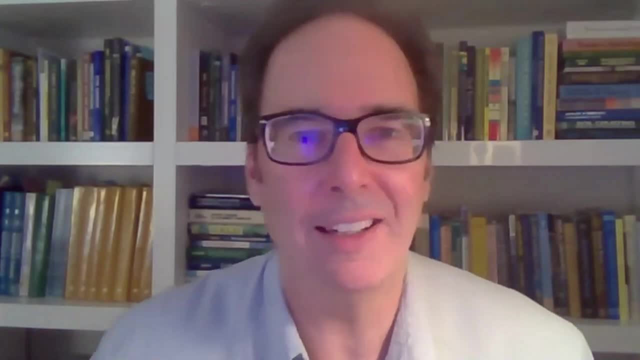 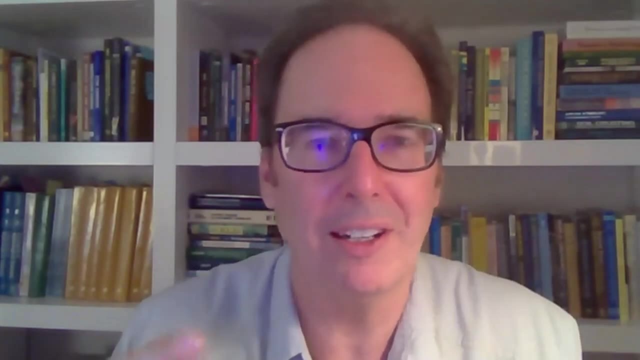 and we expel that water, but it's not this water, it's mixed with the water in our body and that's kind of the residence time of water in our system. yeah, Okay, thank you, And my next question goes. 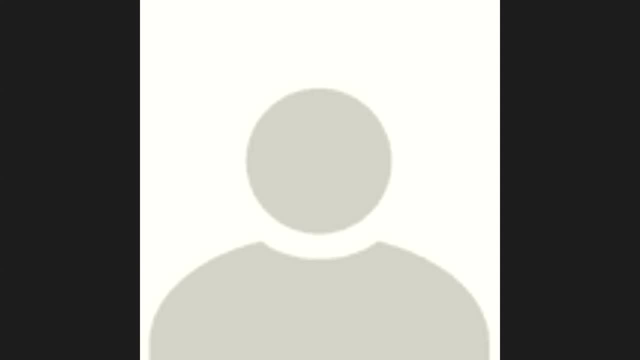 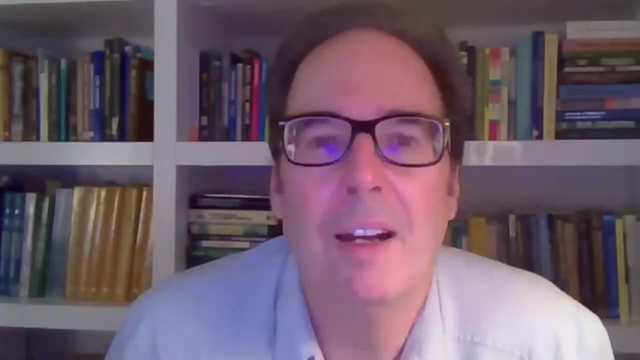 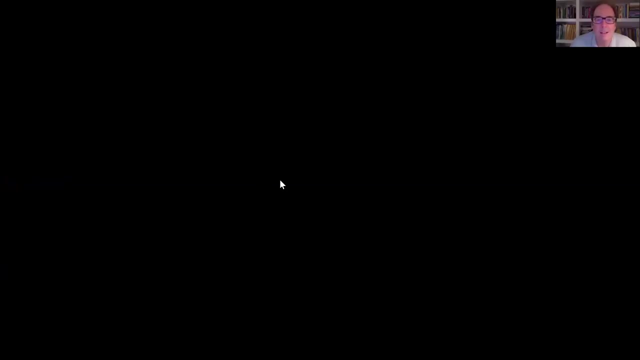 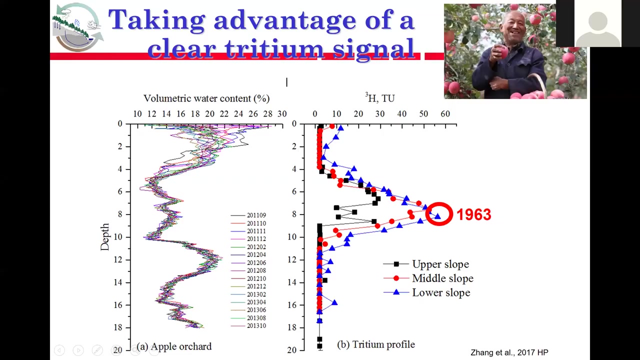 so can we go to the curve comparison between the apple orchard and the curve on the right-hand side? Sure, So yeah, Yeah, the 200, yeah that one. So there is some differences between the slope. we can find the apple slope. 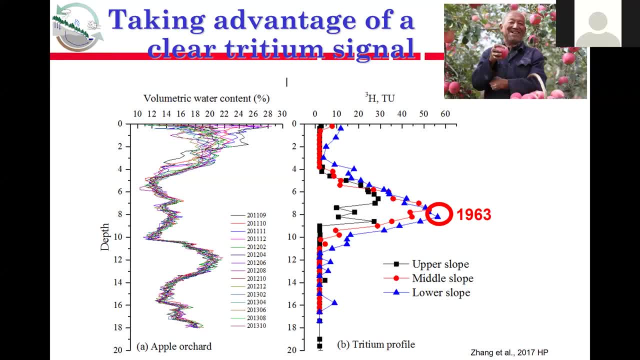 the middle one and the lower one. Is there any relationship between the slope gradients and the output of the time? Yeah, it's a very good question. We can't really comment on that with these data, but I'll show you on in lecture four. 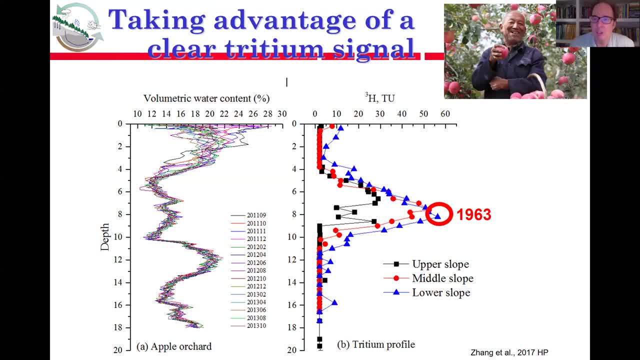 some examples around the world that do show that the slope gradient can have a big impact on the age of the water. So the steeper the slope, all things being equal, the more quickly water is cycling laterally through it and the younger that water would be. 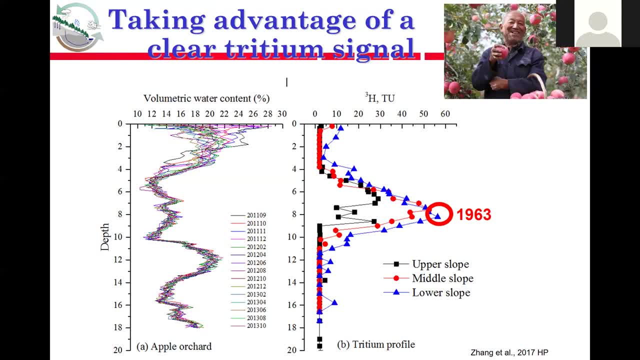 or the flatter would be, the older the water. So it's not a universal relationship. but I can point you to some papers in lecture four when we talk about this that do show that slope angle, slope position, can have an influence on the water age. 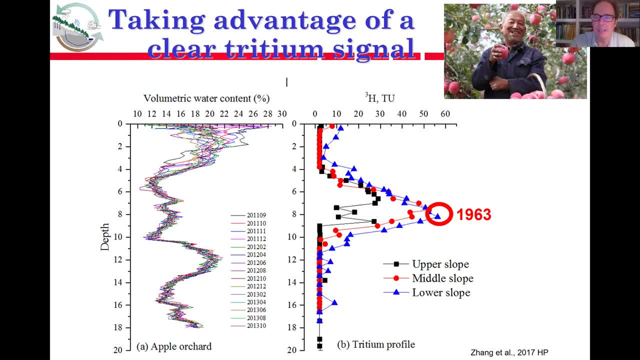 or residence time, just like your human body example. Oh, that's amazing, Looking forward very much, And this is such a hot topic that dozens and dozens of research groups around the world are trying to understand what controls this transit time of water in hill slopes and catchments. 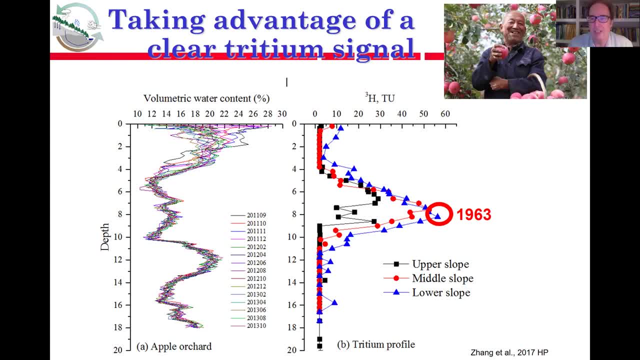 Because if we can understand it and almost predict it, based on climate, geology, topography, this can really help us in understanding where is sensitive to pollution or where maybe vegetation is able to research, recycle water in ways that are easier or more difficult. 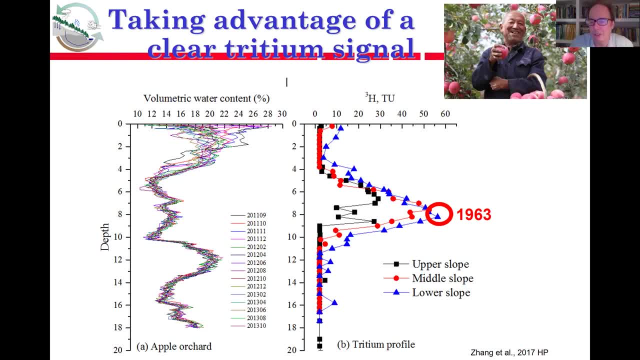 depending on the nature of the water moving through the rooting zone, And again, we'll talk about this in lecture four, which focuses on the transit time of water based on isotope data. I appreciate it, Looking forward very much, Thank you. 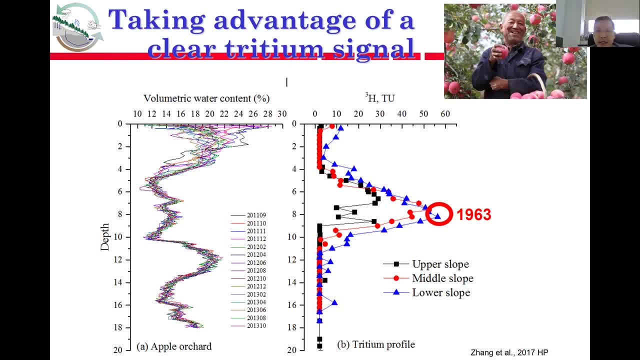 Okay, thanks, Hey, Jeff, just this question. Yeah, Also, I'll focus on this. this figure, Yeah, Yeah, From this figure can we result from? result just to the up-snow, the water, soil, water from the up-snow. 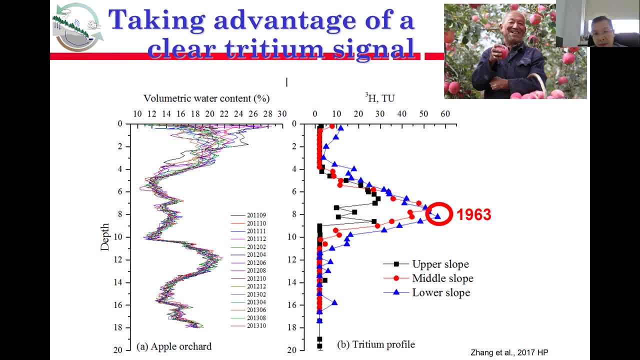 moved to the lower slope, especially for the older water, soil water, because the lower slope has a high value, then the higher value with an up and a middle slope. Yeah, Yeah, again I. it's difficult from just these three single slope positions. 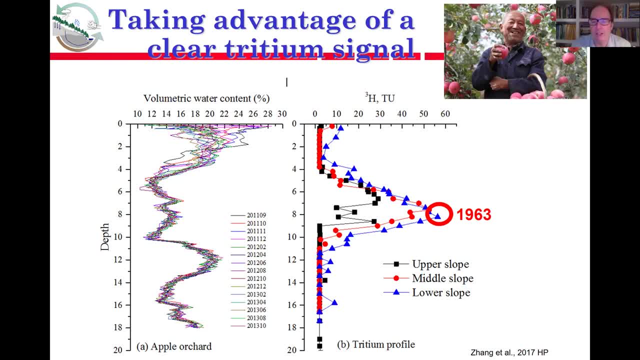 I'll show you examples in lecture four of studies that have looked at this at many different slope angles, many different catchment sizes, to really go after these scaling relations. Yeah, Yeah, yeah, yeah, I think we can do some further research on the different snow positions.